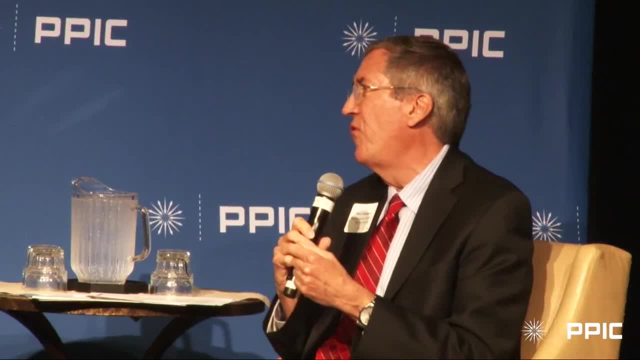 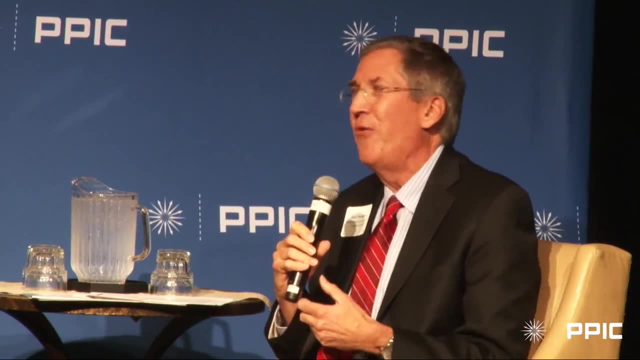 water and then exports it elsewhere. So we have these concerns on the San Joaquin River. We have these concerns in the Owens Valley. We have these concerns with respect to the Colorado River Delta system. We have growing concerns with respect to the Salton Sea. We 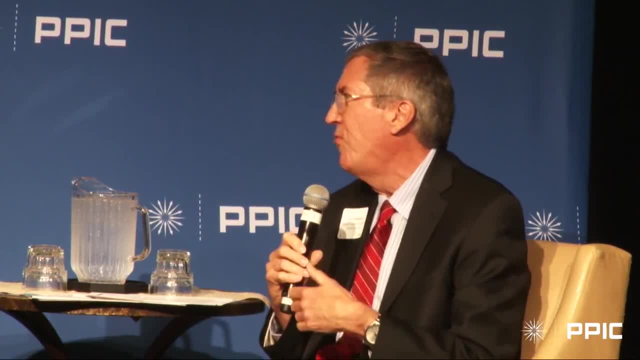 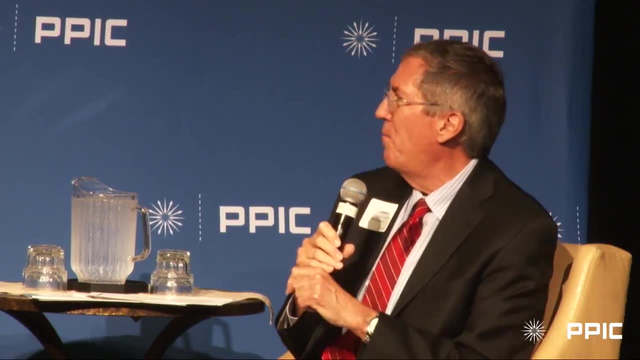 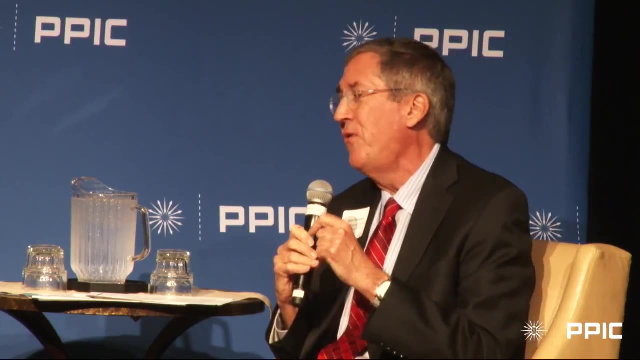 have these concerns with respect to a large number of our rivers and streams in the central and southern coast of California, And even though it's not clear that we're winning the battle, at the same time, the water users point to these environmental laws as a cost to their operations, And, in fact, 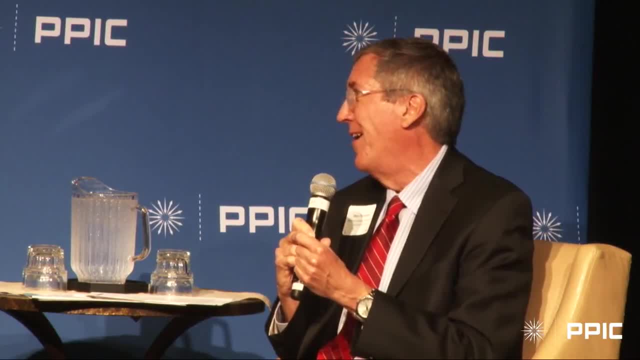 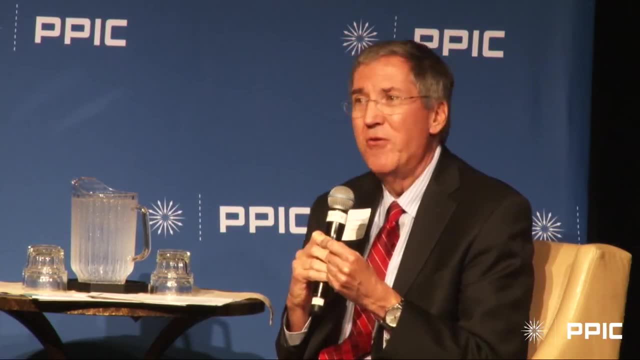 as you heard in the last panel, there's concern raised that our desire to protect the environment might be in conflict with our efforts to protect our underground aquifers. So to address this conundrum and offer solutions to a will that would be the task of our efforts to extract. 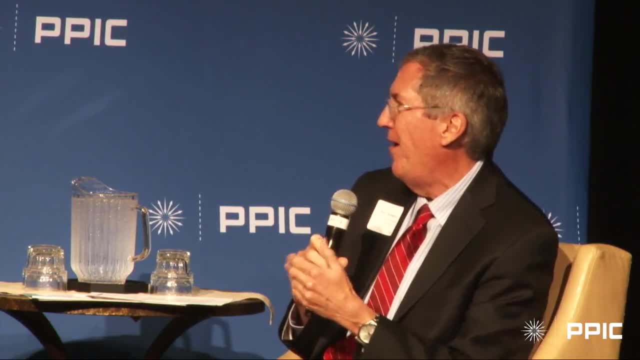 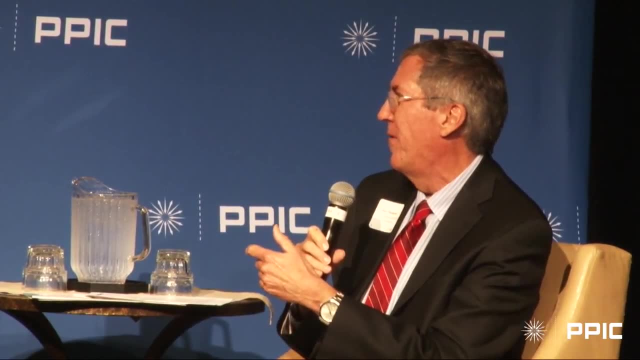 these environmental states, from these rocks, you would question the ability of the marine environment to be protected. So to address this conundrum and offer solutions to a very to it, we have a highly distinguished panel, distinguished scientist, a distinguished policy maker and public servant, and a distinguished environmental lawyer and advocate. 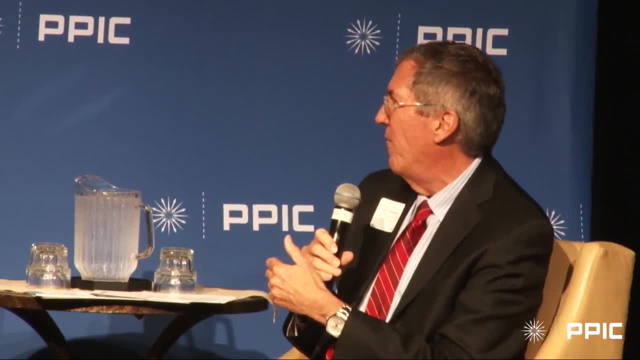 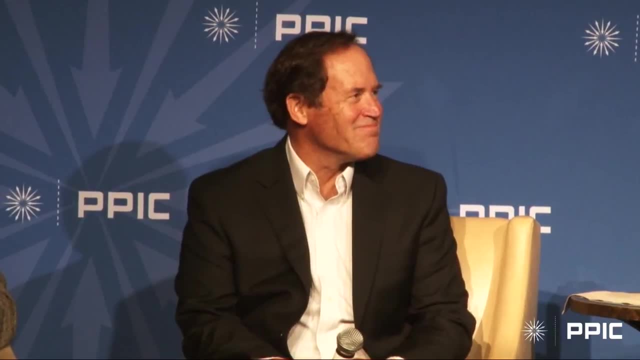 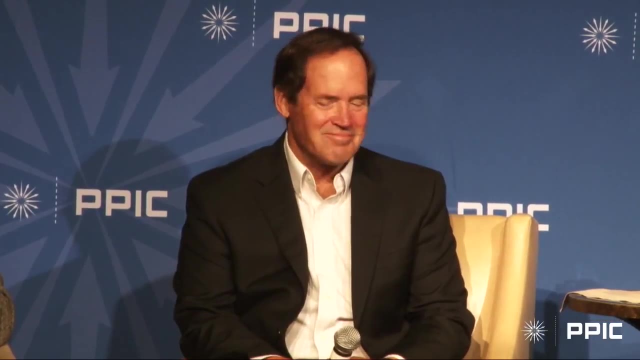 So, starting to my right, to your left we have Jeff Mound, who's a senior fellow at PPIC, a geomorphologist by background and a professor emeritus from UC Davis. To Jeff's right, your left is Phil Eisenberg. 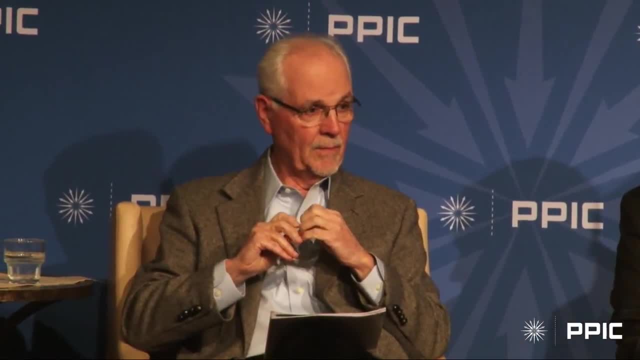 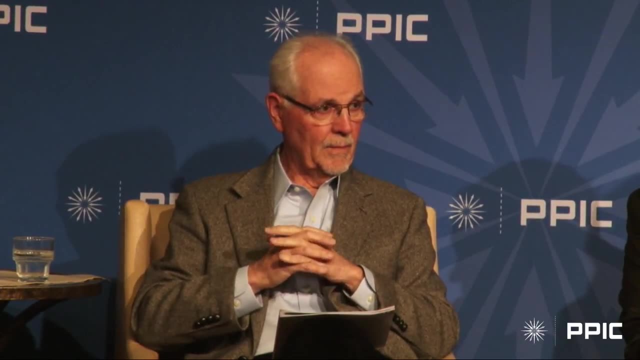 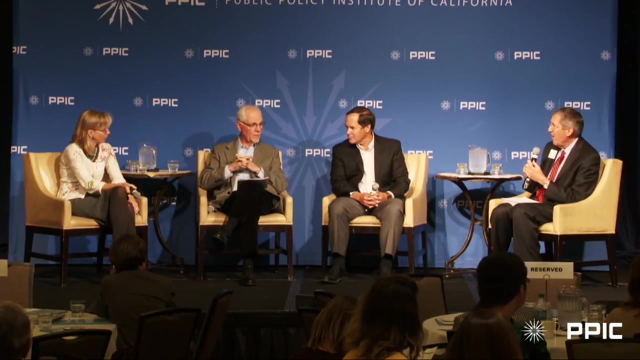 Phil Eisenberg has had a long career in the public sector, beginning with the city council and then mayor of Sacramento, 14 years in the California Assembly and most recently, and very importantly, chair and vice chair Of the Delta Stewardship Council. 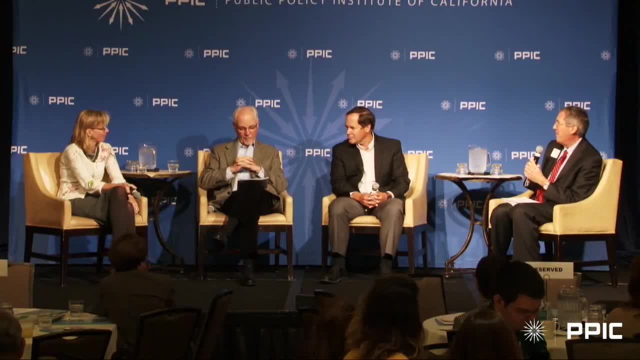 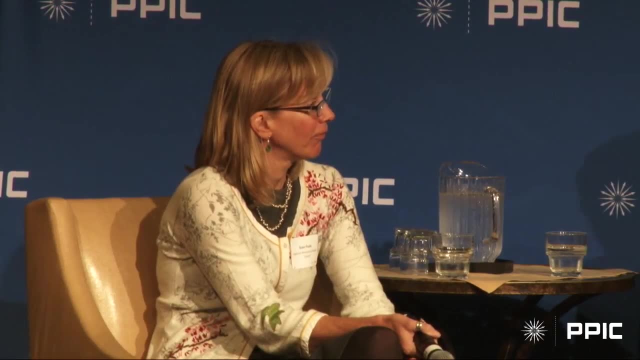 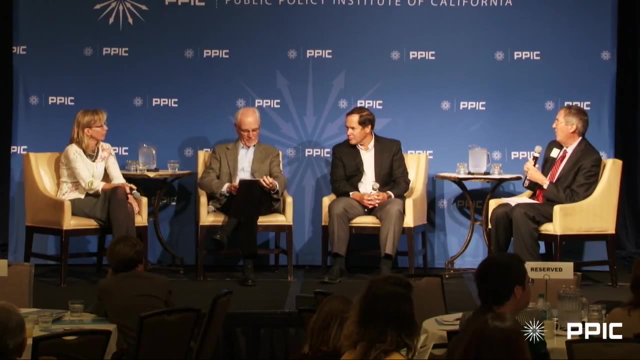 And then, at the far end, on this particular panel, we have Kate Poole. Kate is one of the leading environmental advocates in the state, has been with NRDC for 12 years and has really been leading the battle, most recently to restore the San Joaquin River. 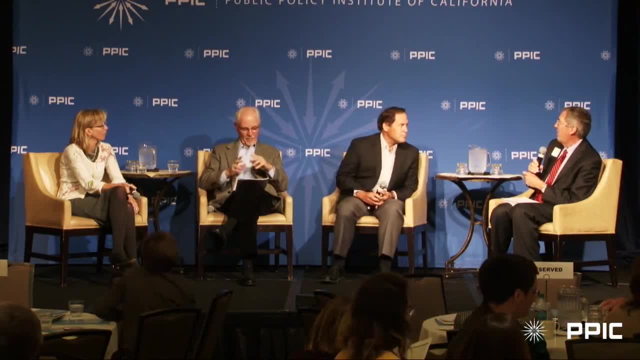 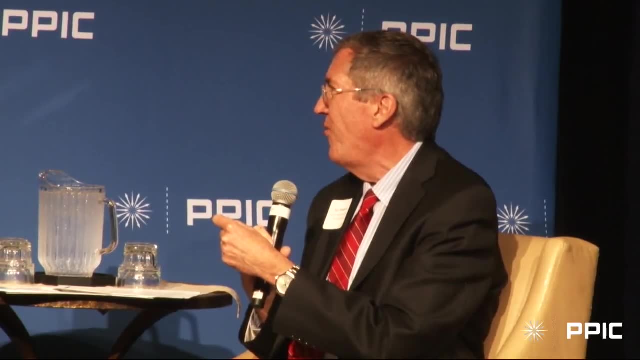 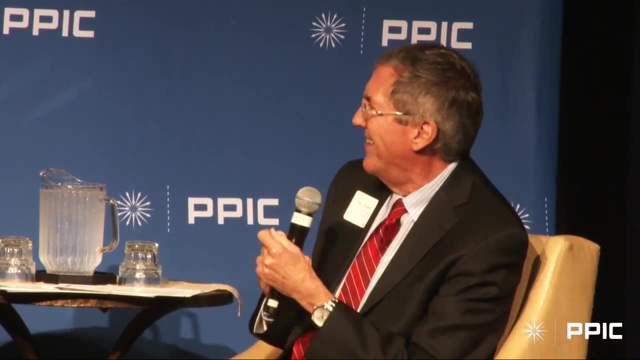 system. So I want to start with Jeff Mound. And Jeff, I would love your thoughts on whether or not the situation is as dire as I just suggested it was, And even though you have a reputation for being the Dr Doom of water, scientists are 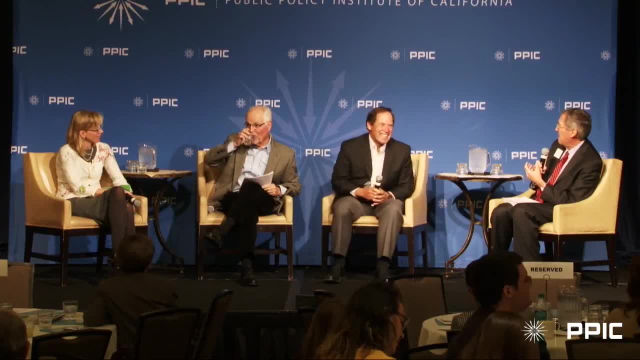 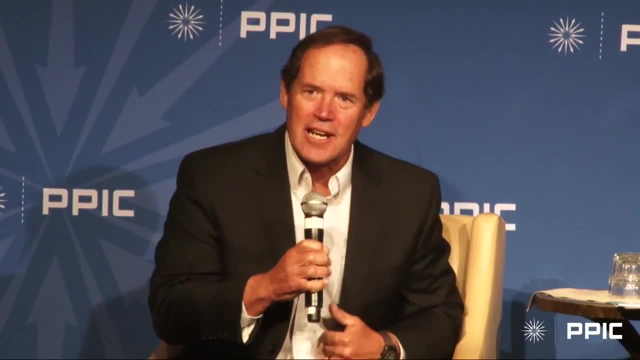 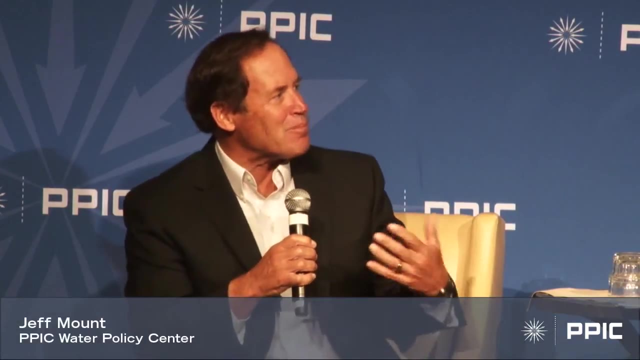 there any rays of light that you can provide us so that we have some hope in this situation? Thanks, Buzz. I just want you to know. today I am channeling Peter Moyle, Who we asked to sit in this seat. So, as a fluvial geomorphologist, I am taking the place of a biologist. 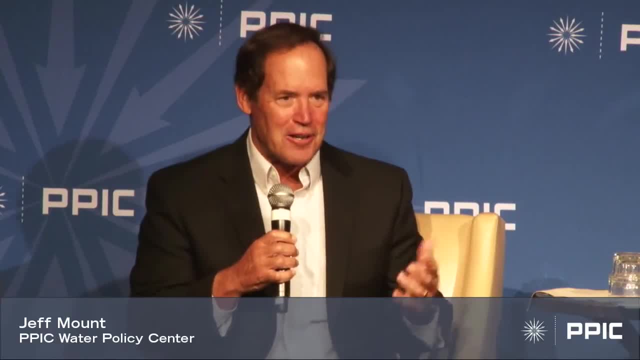 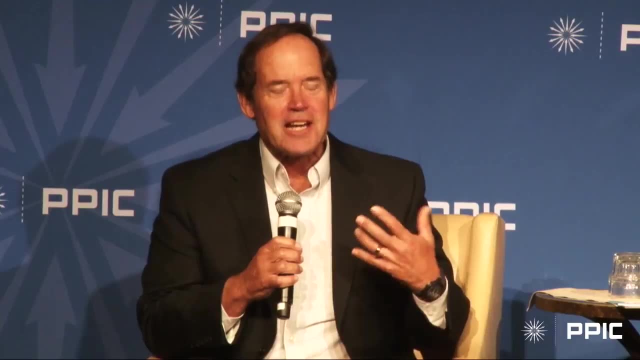 And, by the way, I'm in the friendly shark tank surrounded by three lawyers here, So I'm fully aware of that. But they're nice sharks, They're all nice sharks. So, yes, I do have a reputation as Dr Doom. 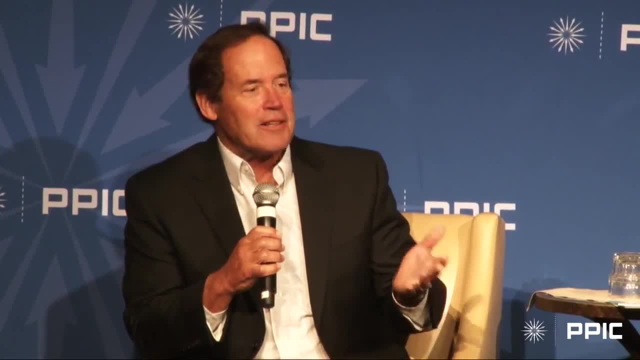 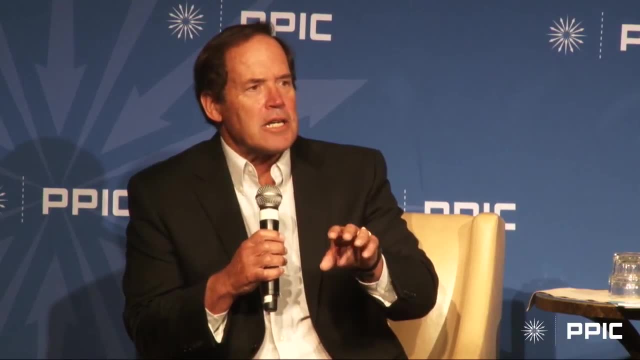 And I'm going to do nothing to dispel that at this point on the environmental side, Real quickly, if Peter were here. the quick lesson we need to take from this particular drought is: in this system The droughts are evolutionary bottlenecks. 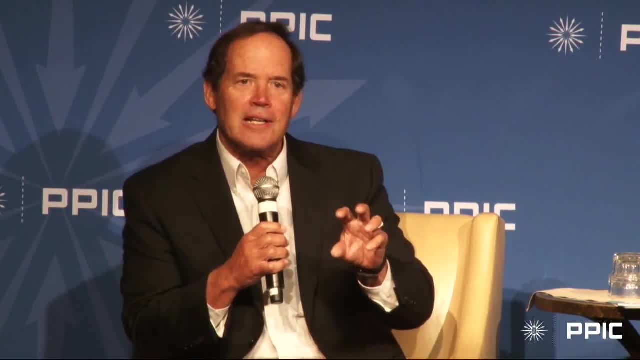 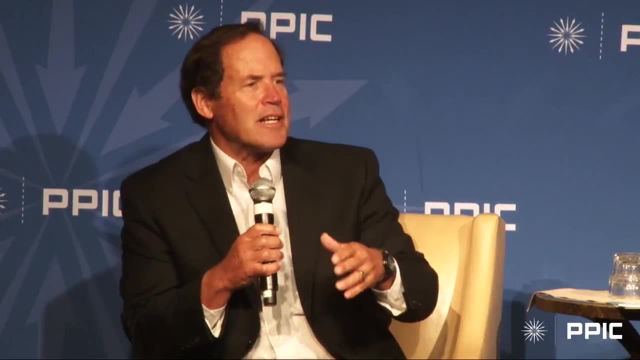 We force our ecosystems through drought periodically And actually that drives a lot of natural selection in this system And, as Peter and I see Ted Grantham's in the audience here- and others have pointed out, we're in a state of perpetual drought in California because of the way we manage. 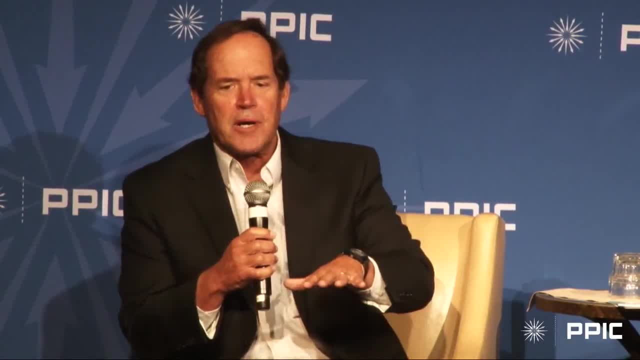 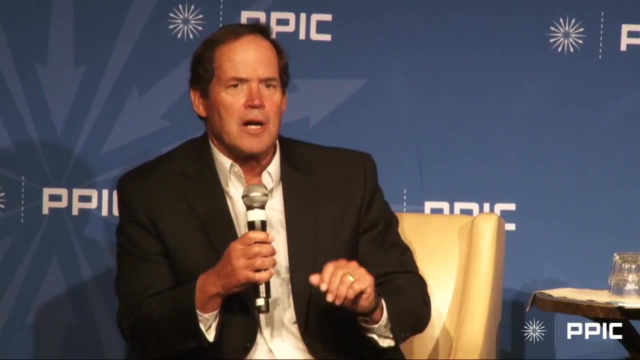 water. I mean, this is inarguable. We're in a state of perpetual drought, And then, when droughts come, they really have a profound effect: biological effect, because we're in perpetual drought, And then a drought of this nature, and this is the last most important thing to point- 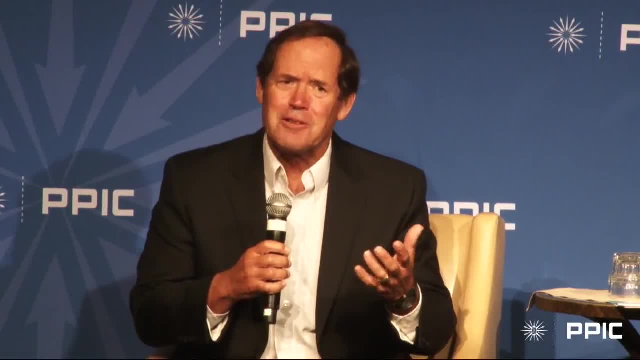 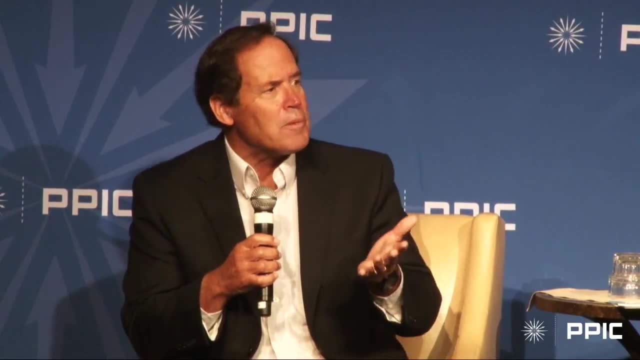 out in our thinking. I am hopeful that by this time next year we all actually understand that this is the drought of the future. We get a window into the future with this drought because it's so warm. Our climate flipped about 1980, 83, somewhere in there and we shifted into a much, much. 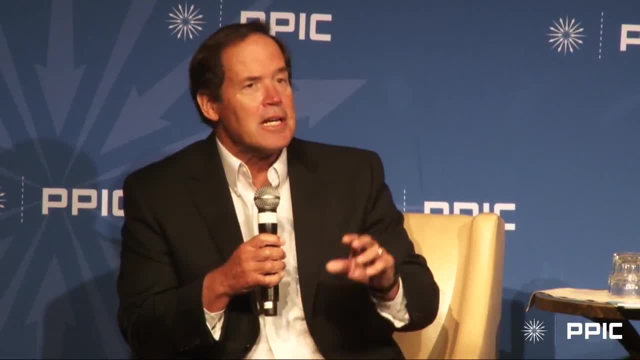 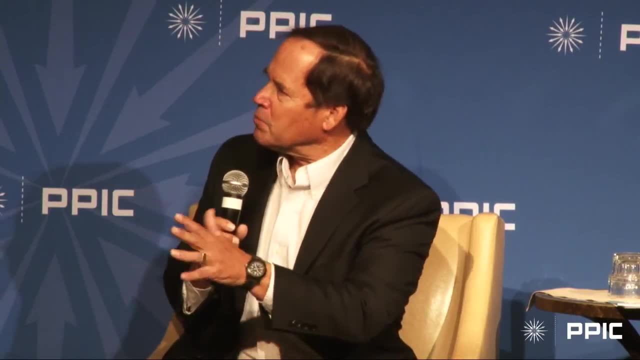 warmer climate, We also shifted into one which is highly variable, So there are some really good lessons to learn from this, particularly because of the temperature of this drought. To all of us who try to manage ecosystems, this is what our future looks like, and it's 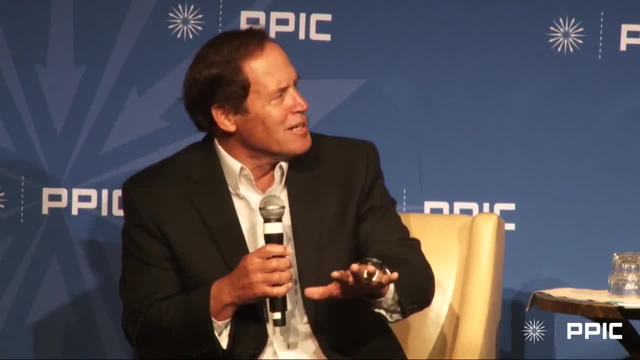 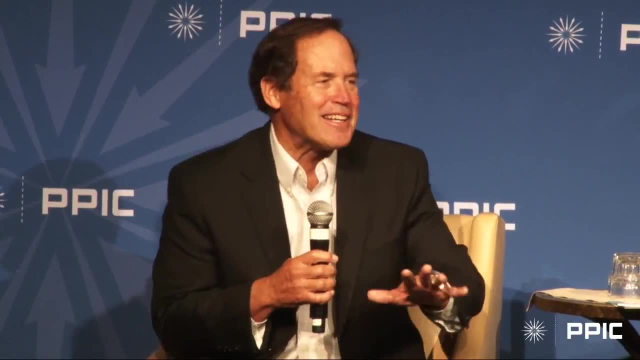 really valuable to take a look at it in that respect. So here let me give you, since we're onto that, what we know. This is all Peter Moyle. We have to remember that This is the most brilliant mind in freshwater biology in California, and so I'm only just 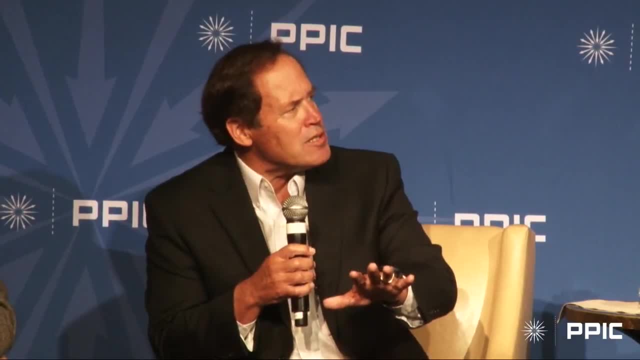 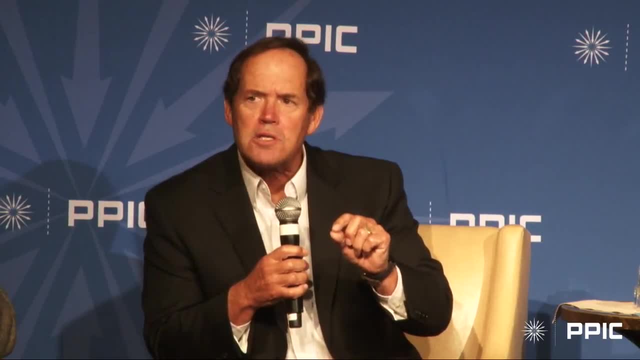 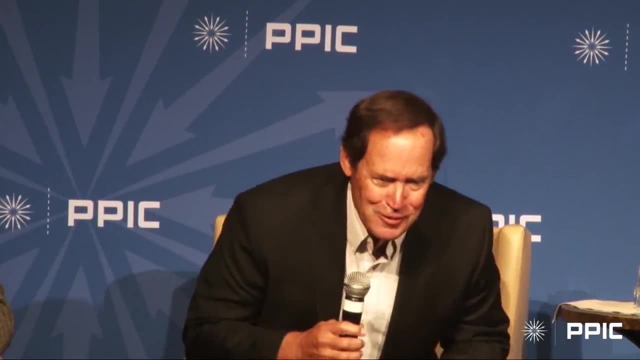 ones that are being hit hardest by this and that their future is pretty grim if we continue with the status quo. So that's one of the big challenges. But I want to flip this on its head, and it comes from spending yesterday reading as: 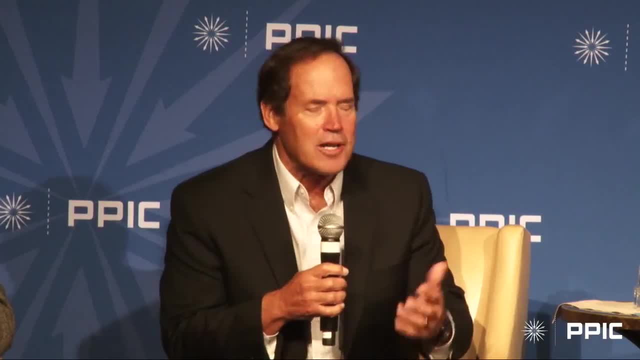 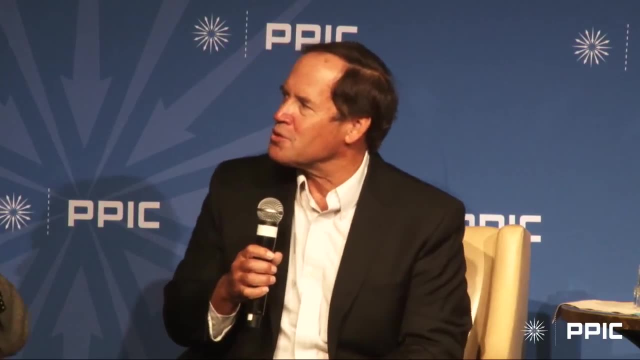 few of us have at this, the State Board's San Joaquin plan, their water quality plan and the approaches they take. Let me offer something particularly for you two to chew on, as friendly sharks as you are: Some general observations. 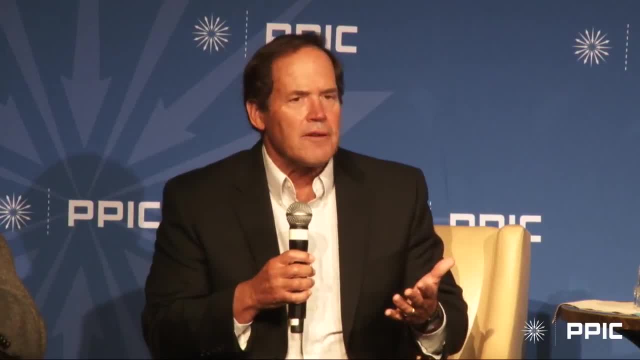 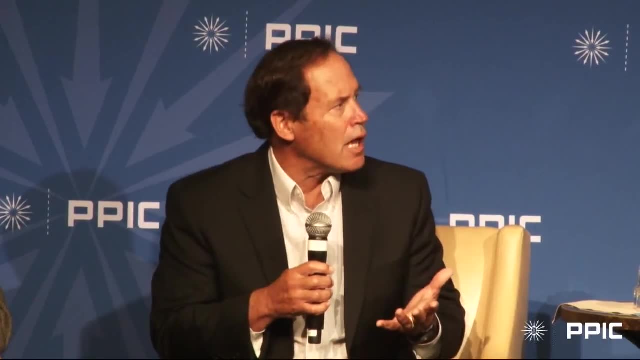 The federal government and the state government, despite well-intentioned efforts, have been unable to arrest the extinction trajectory of our freshwater-dependent species in California. It just simply- I don't know how you can paint it any other way- We have been unable to arrest that trajectory. 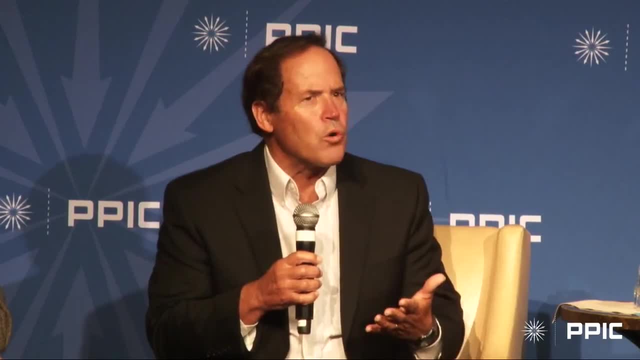 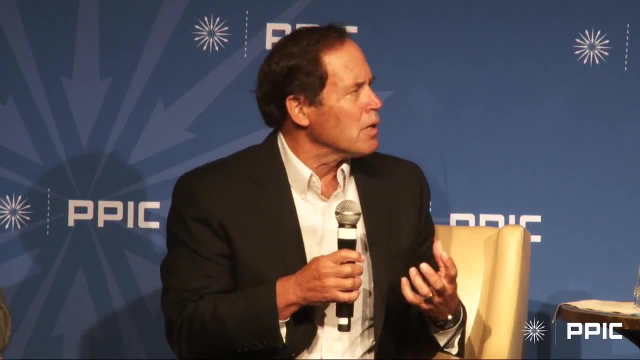 And that the methods we're using, the approaches we're using, are not working. And, in fact, what I'll argue is that what we have suffered from is we've wedded ourselves to incrementalism, And that's been part of our challenge, that what we do is. we say, well, if we just have 80,000 CFS more outflow at the delta. a miracle will occur If we just can release just a little bit more water out of Shasta as a miracle. I just don't think that's going to be the case And there are many sound biological reasons and physical reasons in the system that incrementalism. has not been working. So let me posit something crazy Which has been posited multiple times, Multiple times, since the beginning of the Endangered Species Act: That it may be, in fact we're going at this all wrong And that really we should. that, Phil- and this is in the delta plan itself- is we take. 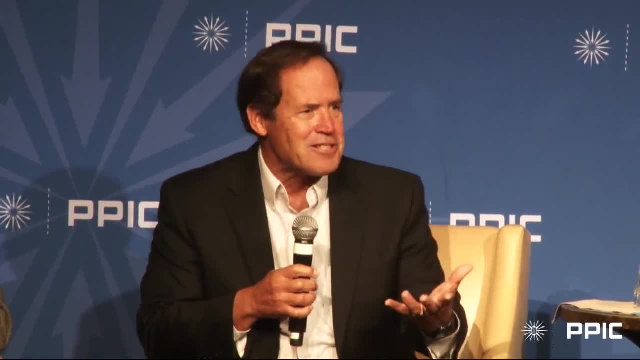 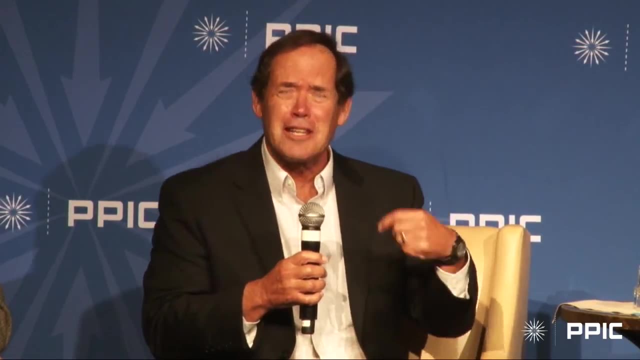 much more of an ecosystem-based approach, That these are ecosystems that we're managing, not species, And I realize that is anathema to many people, Because that is a sort of rethinking of the approach of the Endangered Species Act, And my question for all of you is: can we think more about ecosystems? 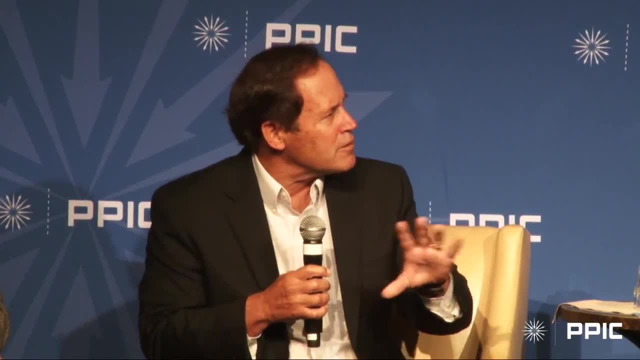 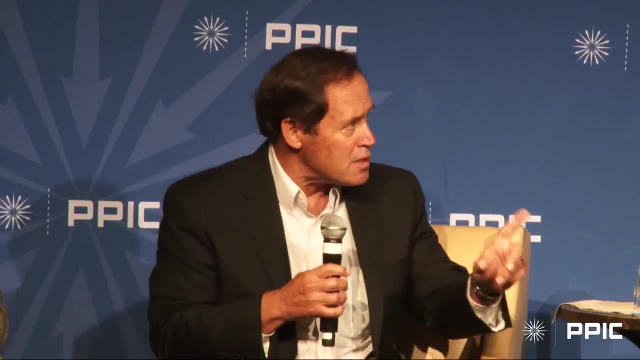 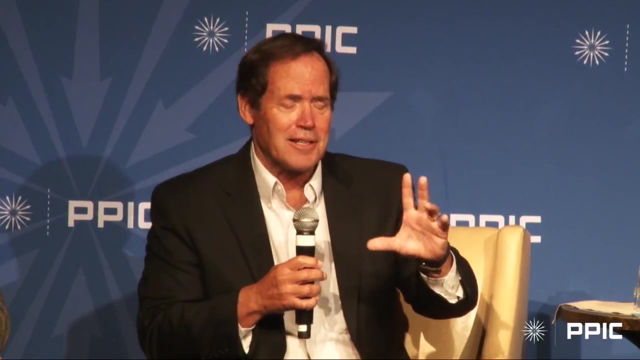 And if you think about it as ecosystems, you begin to stratify, Rethink risk in this system. Right now, what we do is we focus on species-based approaches with extremely high risk of extinction. I'm going to end with that comment about that. 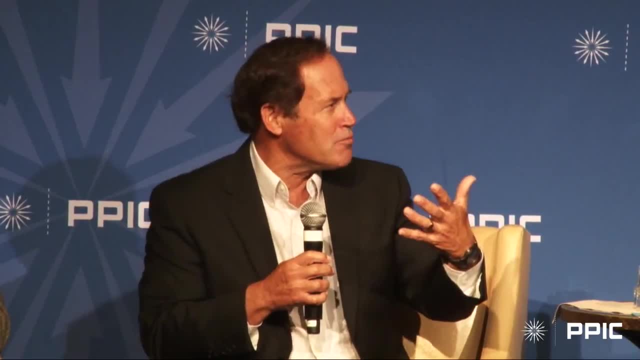 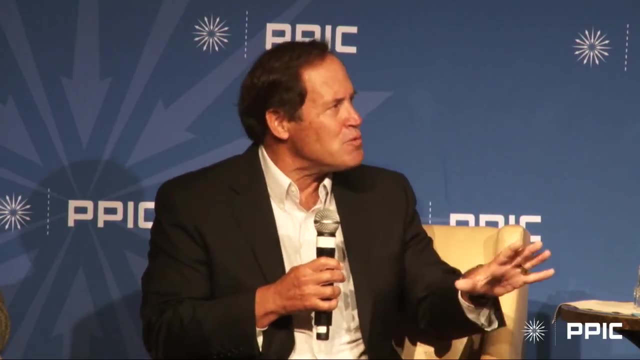 And we put all our eggs into that basket. We need tremendous resource investments in that, Whereas the more moderate risk species with moderate investments might actually do better. And that's if you take an ecosystem-based approach to that. That's what I'm getting at. 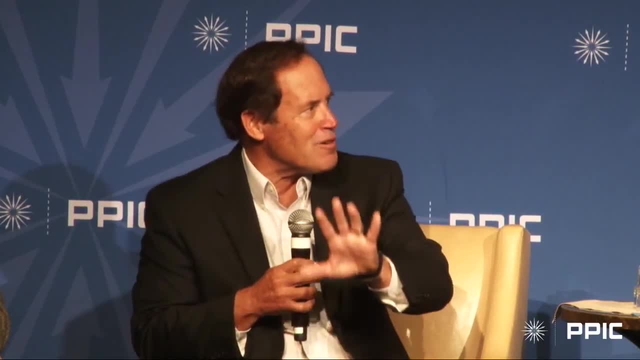 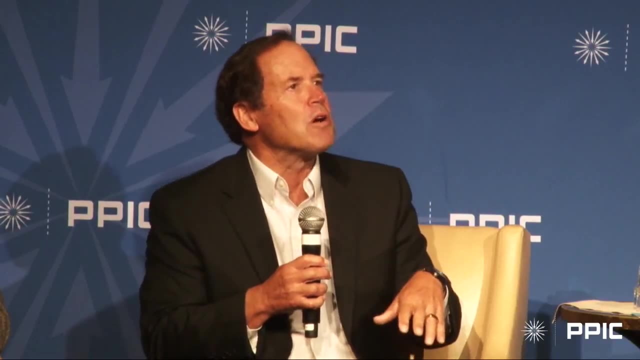 Is that you know we can do really great things on ecosystems if we focus on the ecosystem function rather than the species. So let me keep going with that. One of the radical things we wrote about. you were an author on it too, in a book in. 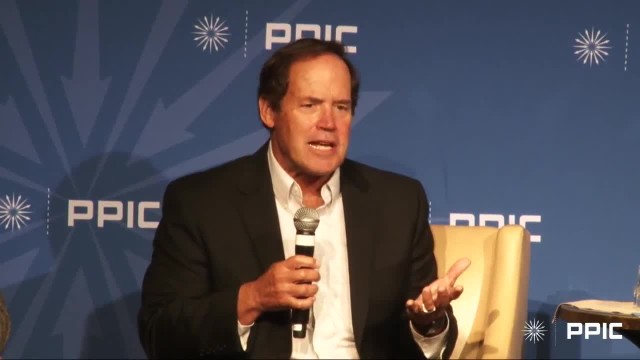 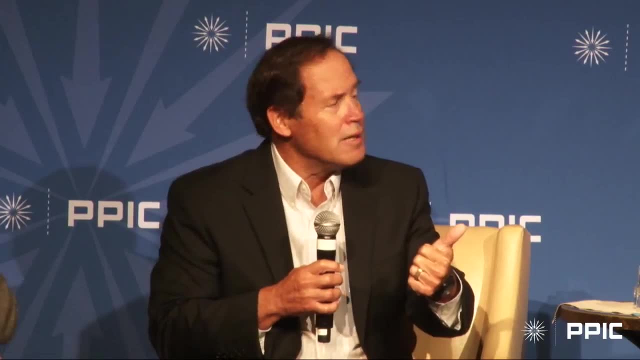 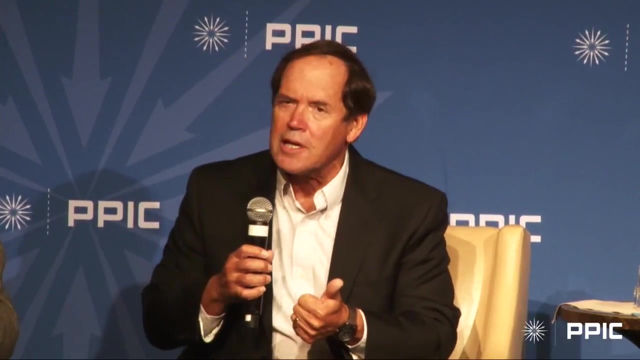 2011, we said rethinking the approach that we take. if we do it as an ecosystem-based approach, what we're doing is we're starting thinking about specialization, Not trying to do everything everywhere at all times. It's acknowledging that not all species will exist in all of their historic habitats. 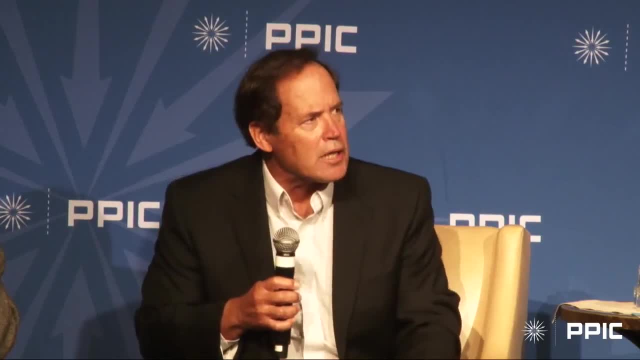 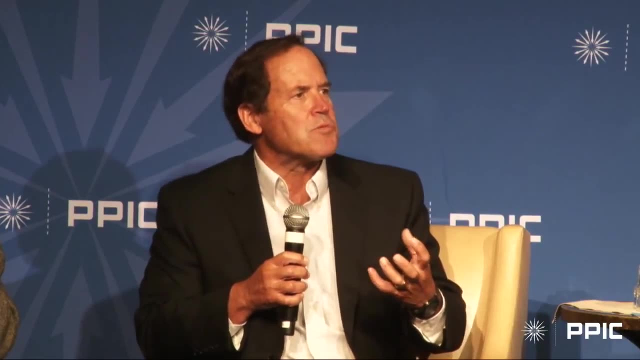 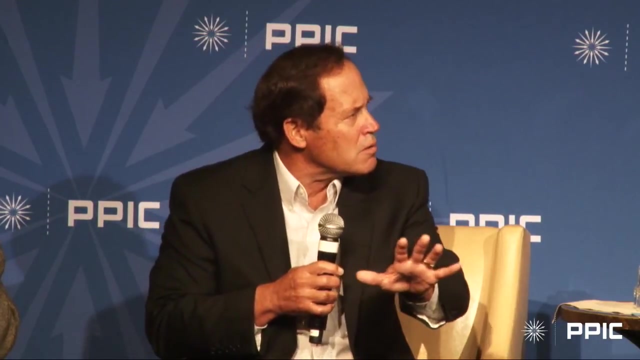 And that we should be making investments in improving habitats where we can get the best return on those investments. So this is a notion of specialization, Or, as Peter Moyle would say, making investments which have very, very high level of return, and some of this could be refugia. you know, conservation of cold water is a good example. 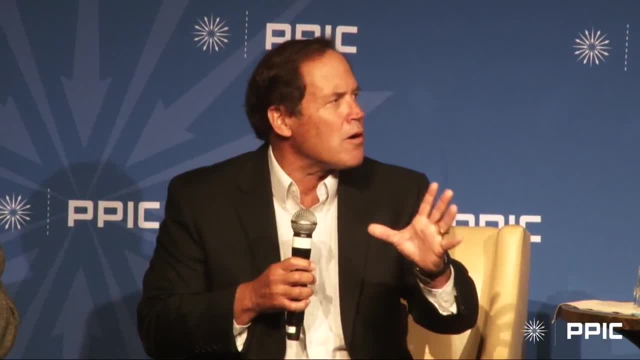 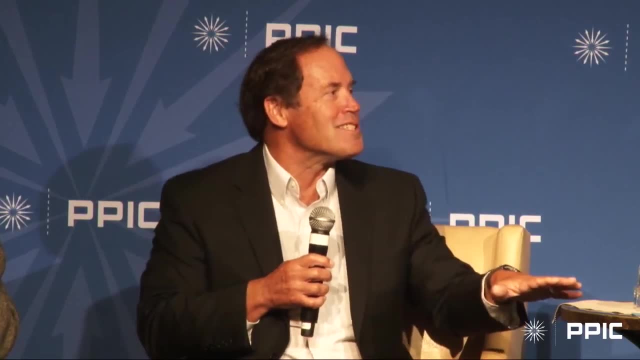 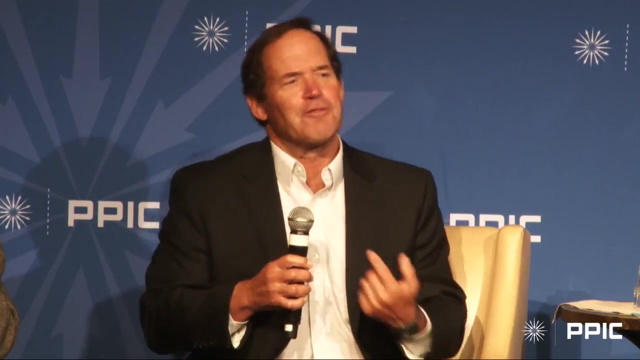 Finding those places, that those river segments which are of very high value, and making investments in those, And that means not making investments in other places. And specialization also is the radical notion and I'm going to get in so much trouble from this to my right. 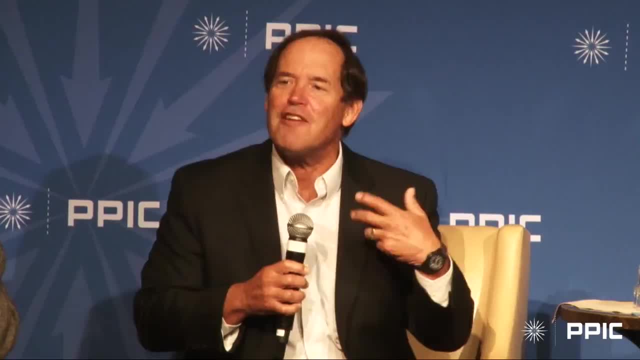 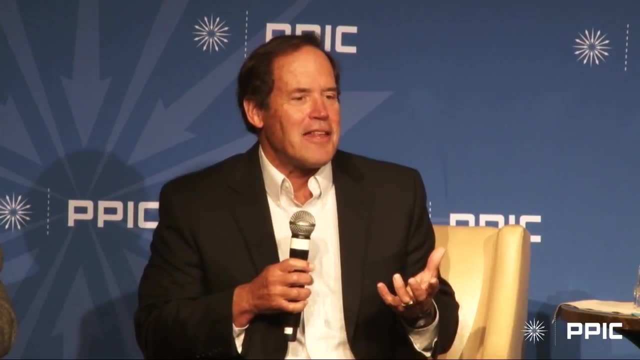 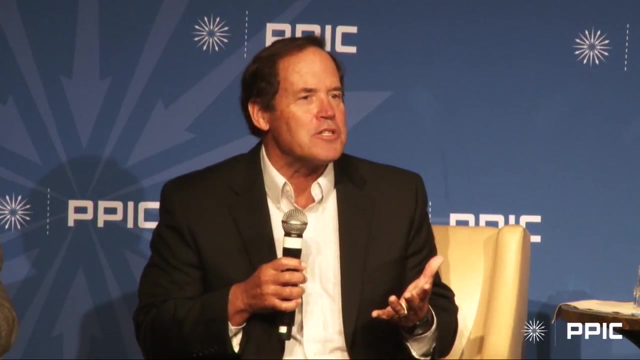 Well, you always get in trouble. I know Well this. I mean, I have been instructed to be provocative, so I am being provocative. There's this radical notion out there that we can't have salmon everywhere And we need to concentrate our limited resources so that we have salmon everywhere. 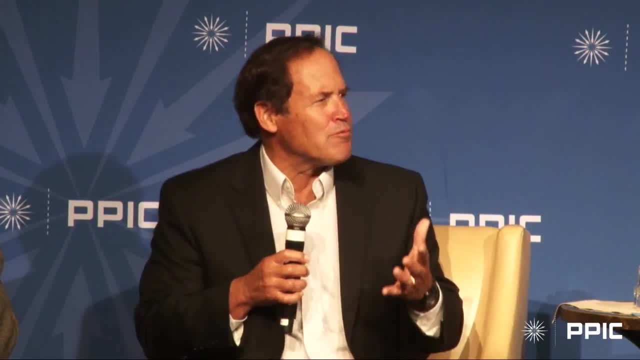 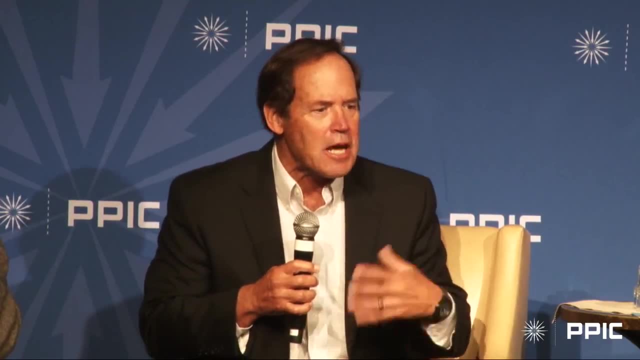 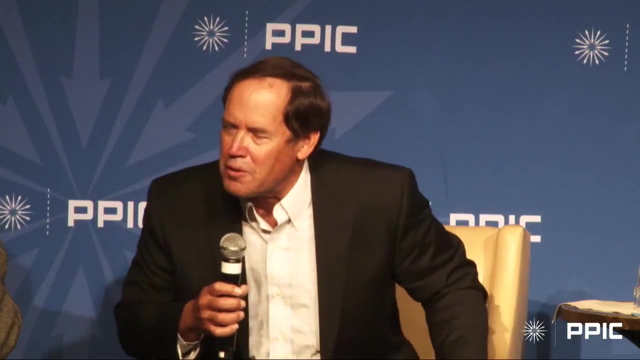 And that we have salmon where we can have salmon and make for robust populations. That is a radical notion. And another radical notion is that some species- and this is getting to the end of this- look for those of you who don't know, we surprised the biological community and Phil remembers: 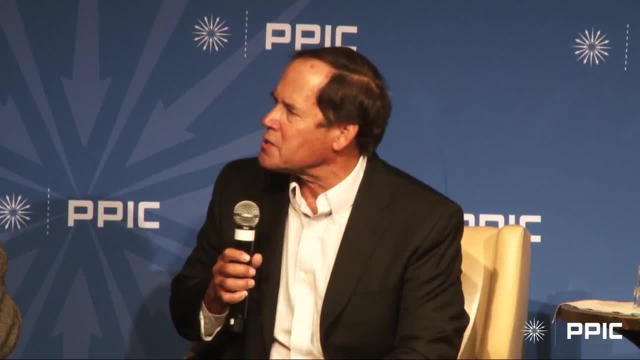 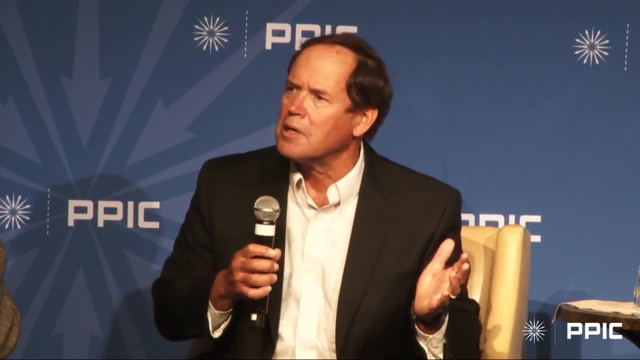 this well, a few years ago, where we did a survey and we asked them- an anonymous survey- to look out into the future And the conditions, The conditions of some species out in the future. And if you haven't seen this, this is a PPIC report where we looked at multiple stressors. 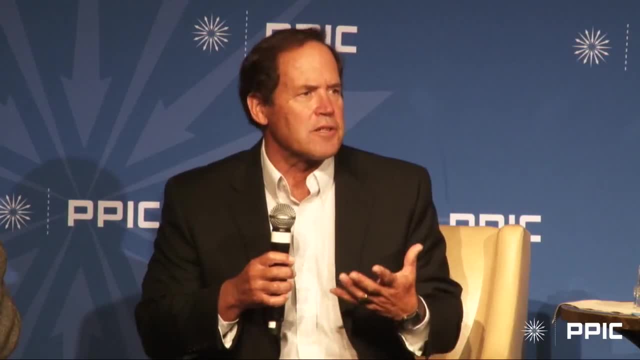 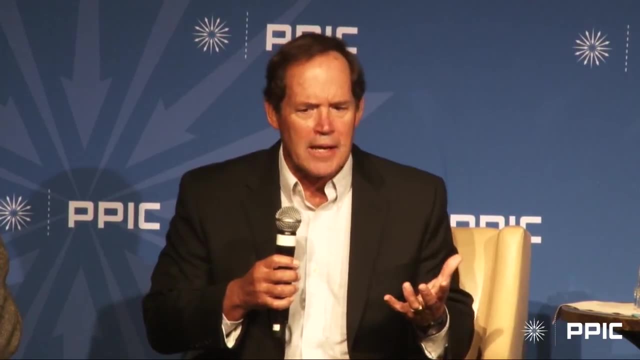 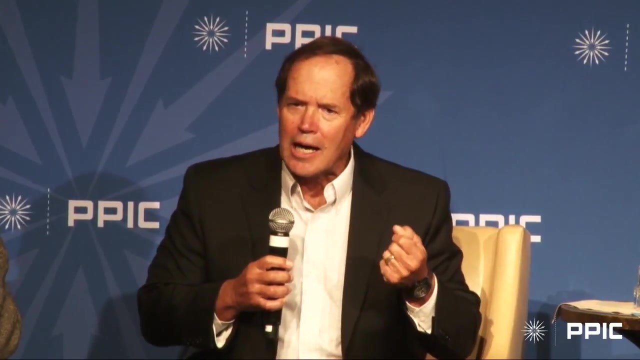 in the delta. It was illuminating to see what the biological, the scientific members of the community would tell us about the future of these species everywhere. And this is the now painful discussion, because I've been told to be provocative- My friend Peter Moyle will tell you that he thinks some species are now functionally extinct. 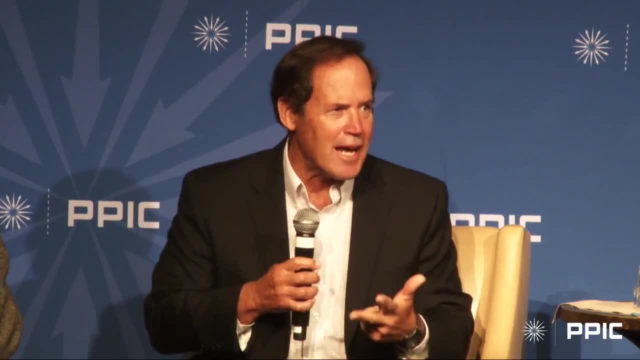 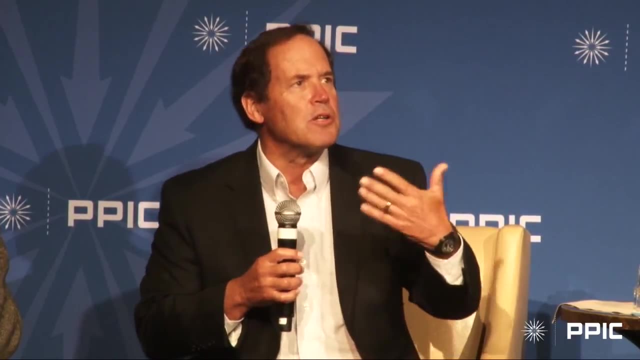 and some species are headed for extinction and we need to have an adult conversation about what that means For some members of some communities. I believe the ding-dong- the witch is dead- will come up and we're going to be. this is great. it's going to liberate great quantities, vast quantities. 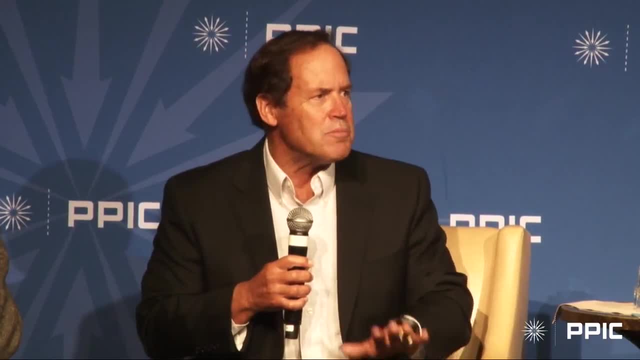 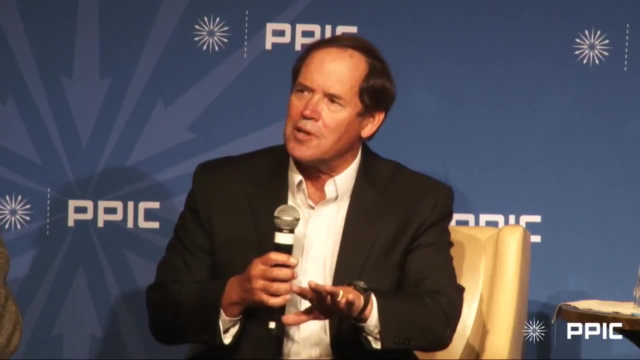 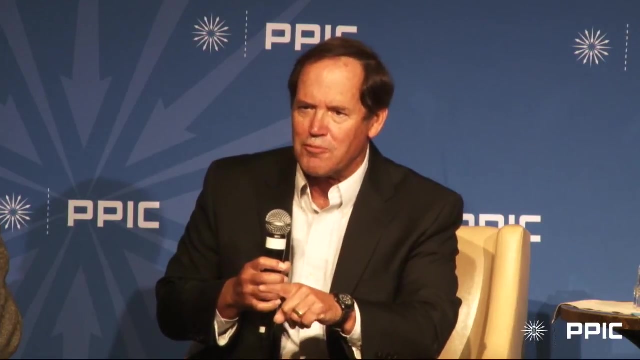 of water for other uses, consumptive uses. That would be a terrible mistake, because what has happened for us is so many of our ecosystems- if we're taking an ecosystem-based approach- are actually now reliant on the Endangered Species Act to basically keep those ecosystems in some way shape or form. 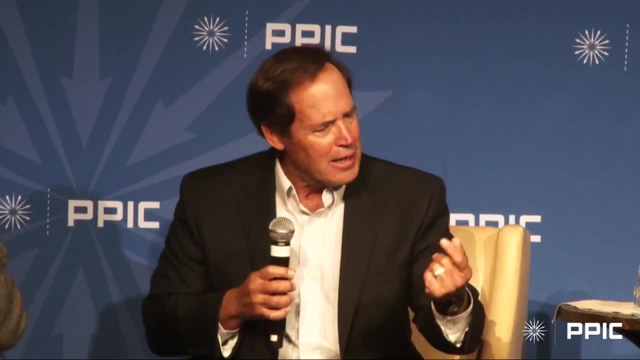 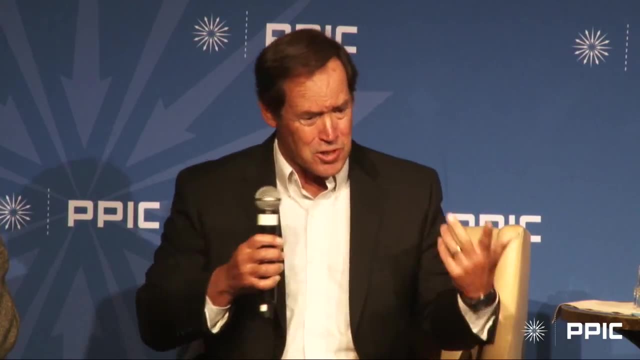 So that's the last provocative thing I want to add in here. I think we need to take an ecosystem-based approach to management, and the reason I think that is because our ecosystems are changing and the pressure's on them and we cannot make perfect endangered species habitat everywhere. 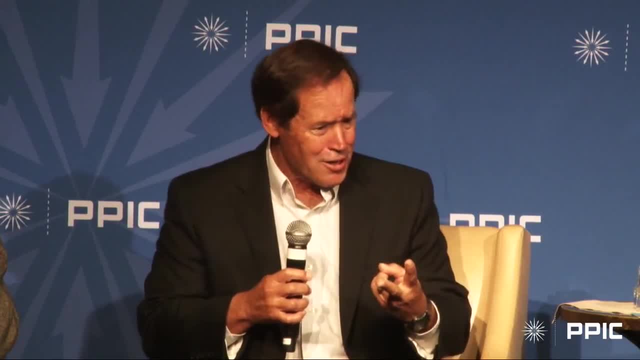 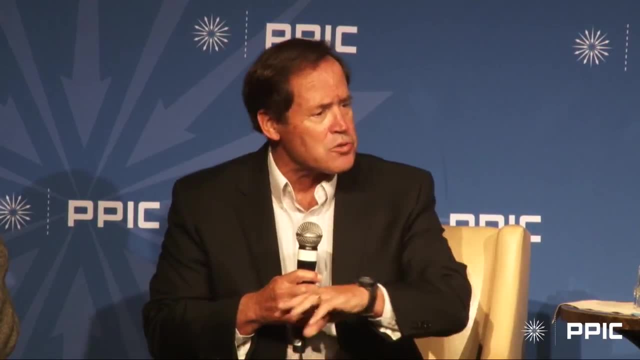 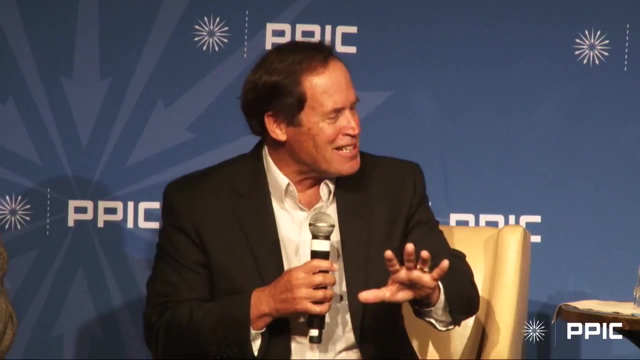 And an ecosystem-based approach also has us stratify our risk and invest our resources more strategically, rather than trying to make sure it is good everywhere at all time. And then, finally, as I say, I'm supposed to be provocative here, but let's have a conversation. 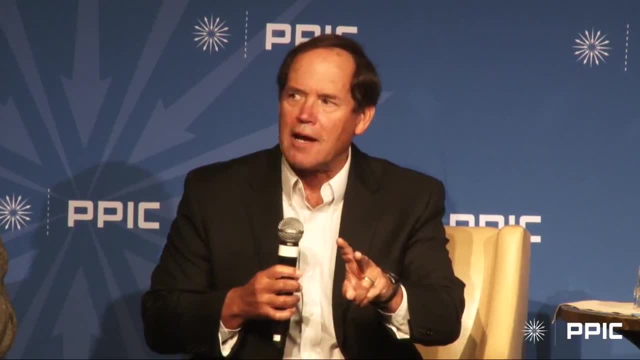 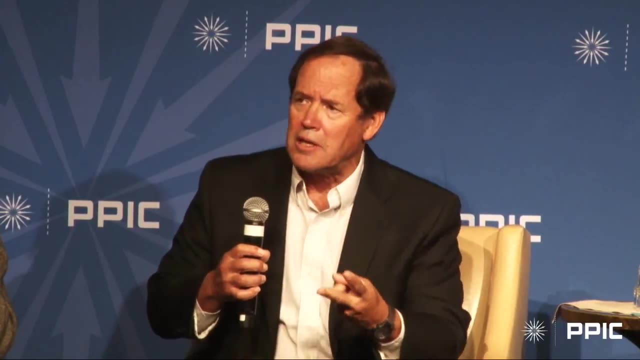 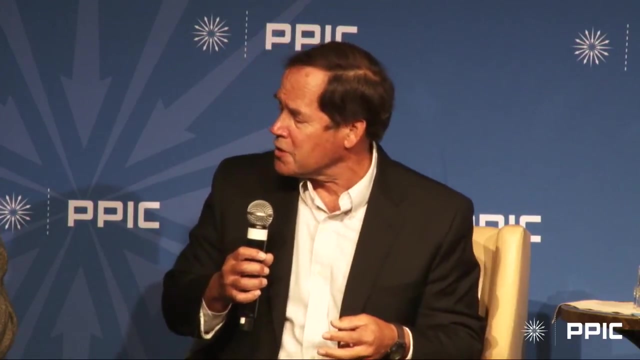 about what extinction means. We all know the Endangered Species Act did not consider it in detail and did not consider extinction and what the consequences of extinction would be. And then the second aspect: is it never anticipated climate change, changing climate conditions and changing habitat conditions, which will put stress on the ecosystem? 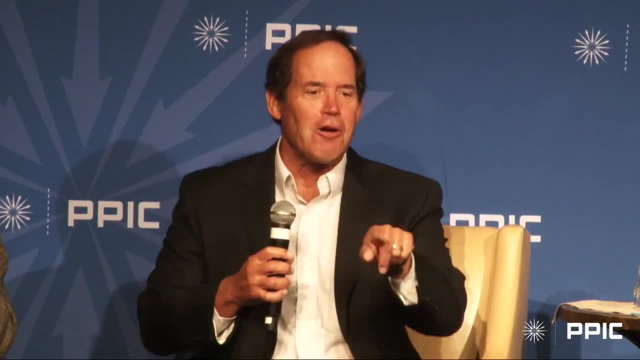 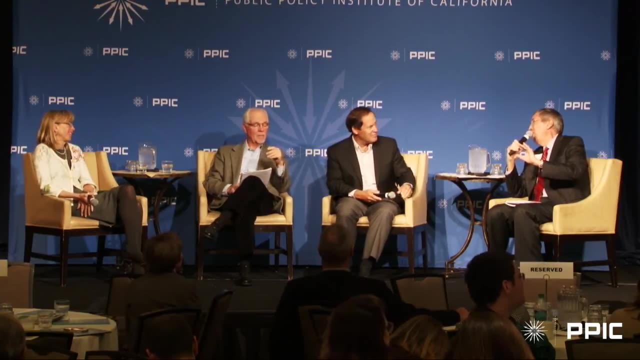 So, with that being the provocateur, I shall now crawl under a table somewhere and wait for my answer. Okay, So, Jeff, you have now answered virtually every single one of my questions. Your bottom line is: we're not doing very well. 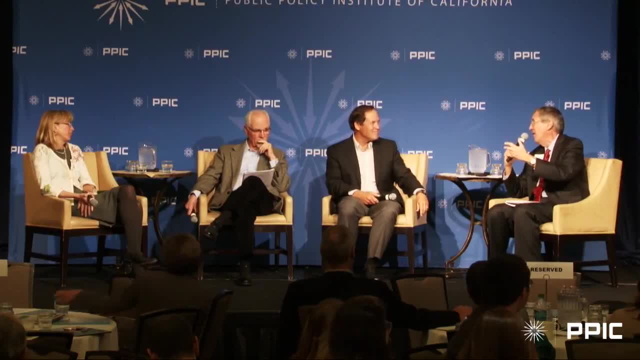 The trajectory is awful. Our current approach is not working And in your view, as far as I can tell, that's largely because we are focused on species rather than a broader ecosystem approach. So your solution is to move to that broader ecosystem. 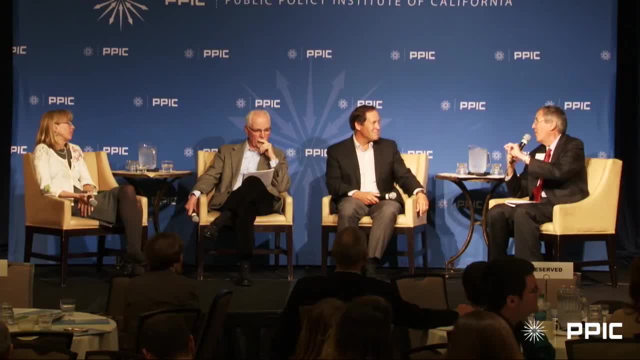 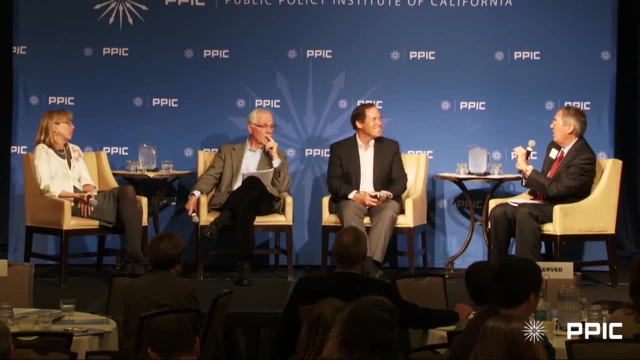 Okay, So you have a very interesting approach, and what you then, of course, address is whether or not we can do it under our current laws. But I want to break that up a little bit and start out by also asking both Kate and Phil. 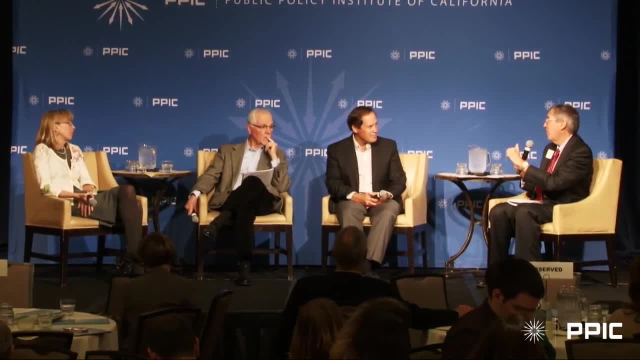 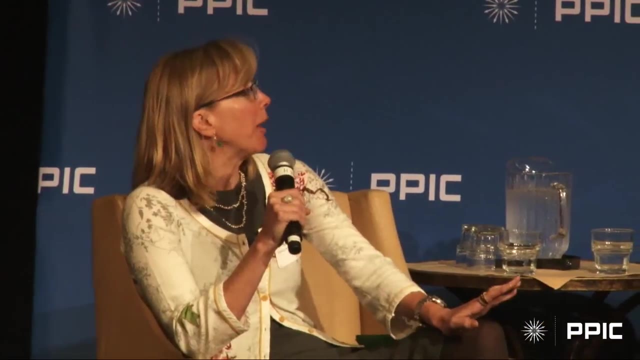 their views as to is our current approach working? And if it's not working, what's your view as to why it's not working? So start with you, Kate. So I agree with Jeff. I agree with Jeff that we're going about this all wrong right now. 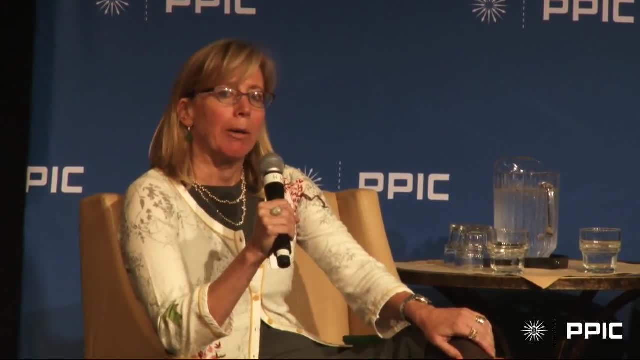 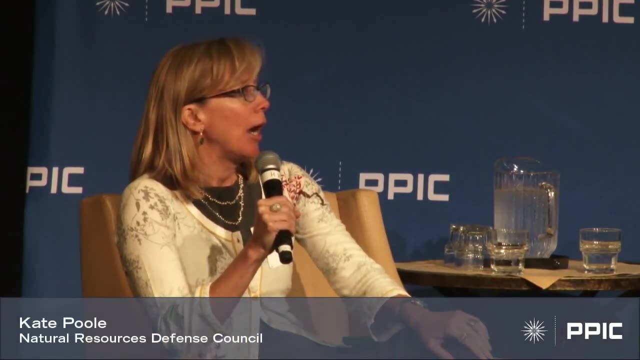 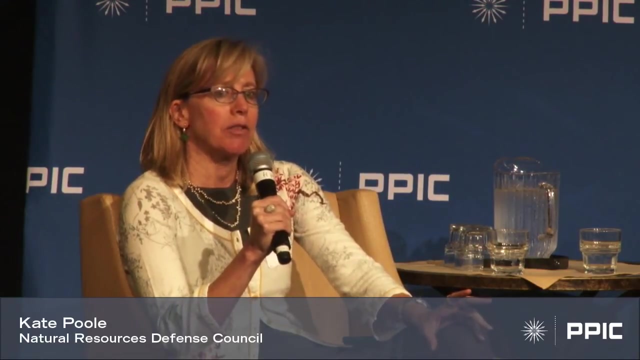 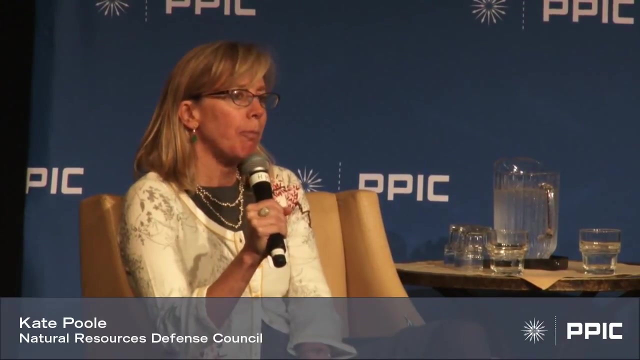 And my view on how we're going about this wrong is that we are generally operating- particularly the Bay Delta system- way too much by relying on the Endangered Species Act. The Endangered Species Act is designed as the emergency room for species. It's the last-ditch effort to stave off extinction. 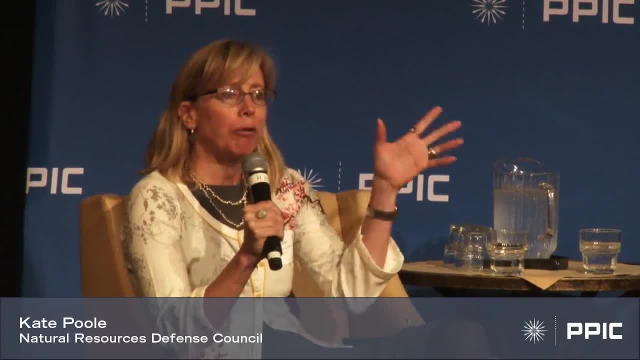 And what it basically does is it's the last-ditch effort to stave off extinction. But what it basically indicates it's- you know, you know, it's a flashing neon sign that we have failed to enforce all of those other good laws that that you mentioned. 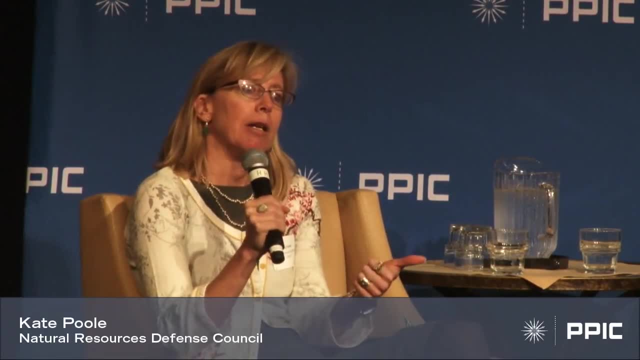 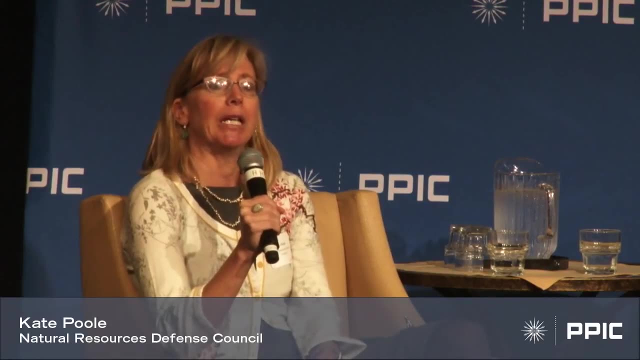 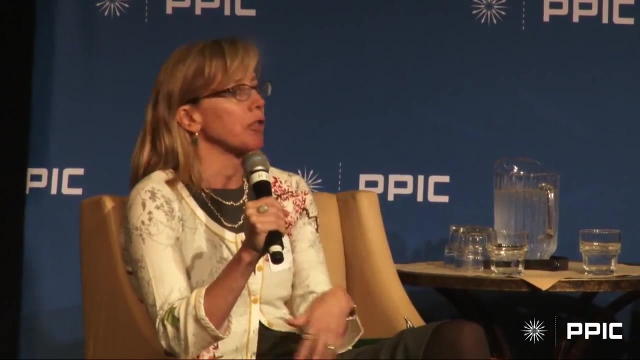 in your opening buzz. We have an updated water quality standards in the Bay Delta, substantively in more than two decades. That's a big failure for you know, reflecting the current science and the current needs of this system and the pressures of climate change and all of the other things. So the issues of water quality must be careful That dealing with things of the system bate on if they must be taken into account. this incident will have a negative impact, sign that we have failed to enforce all of those other good laws that you mentioned in your 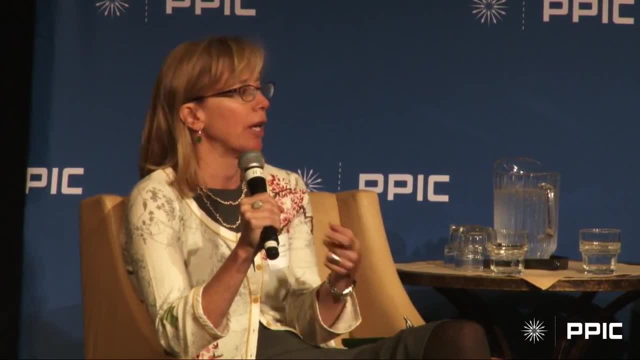 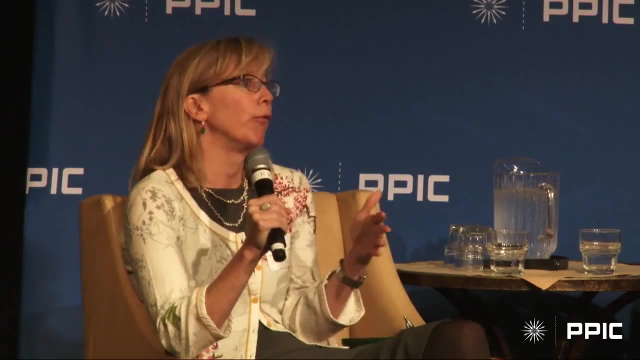 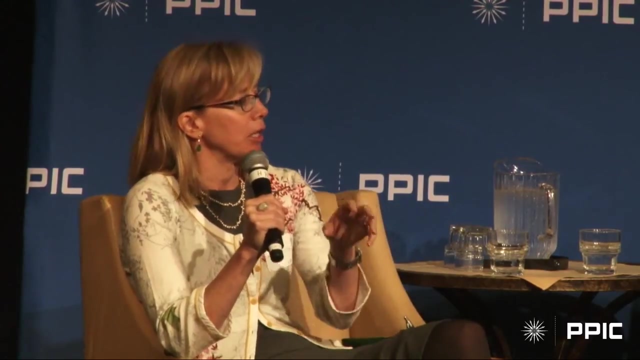 opening buzz: We haven't meaningfully enforced the public trust doctrine 5937, a number of other laws that really are much more foundational and much more focused on the bigger picture of trying to create a healthy ecosystem. that addresses a lot of issues and, in the case, 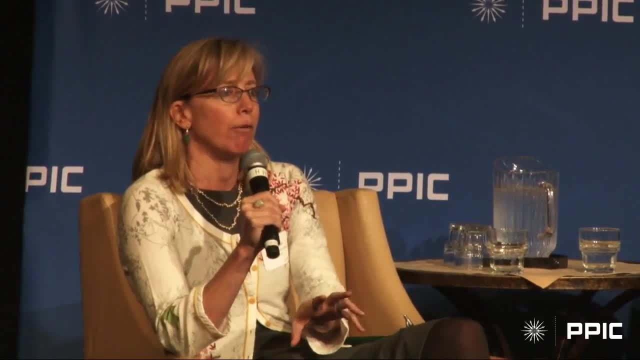 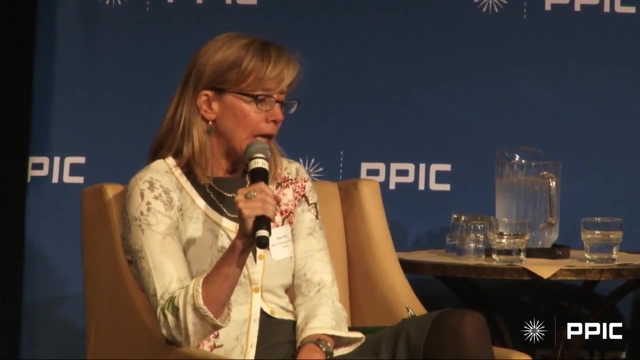 of the Water Quality Control Plan. does that in the context of? you know what are the other needs that we have to meet while we're doing this. So I think you know the fact that we have basically called jeopardy on this system, for 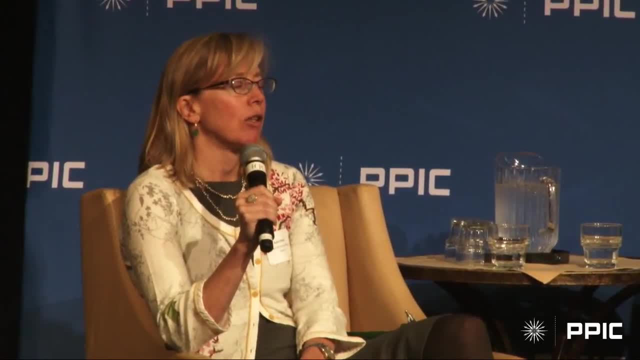 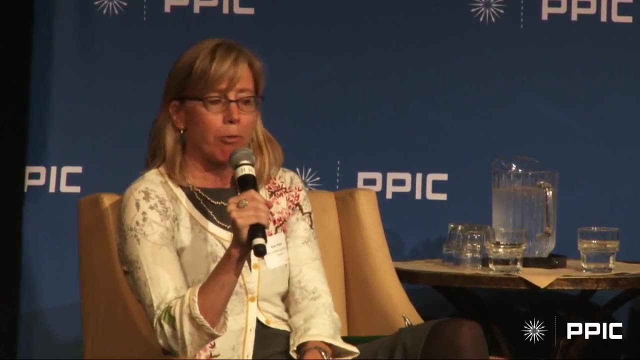 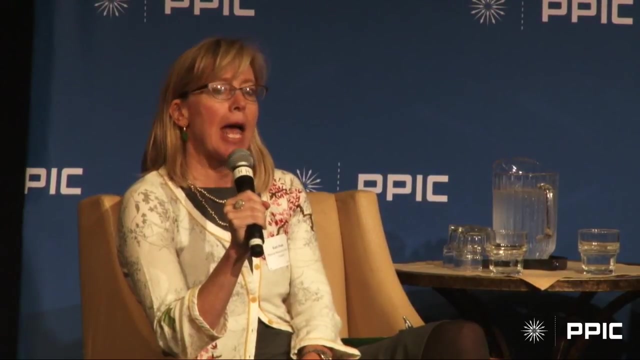 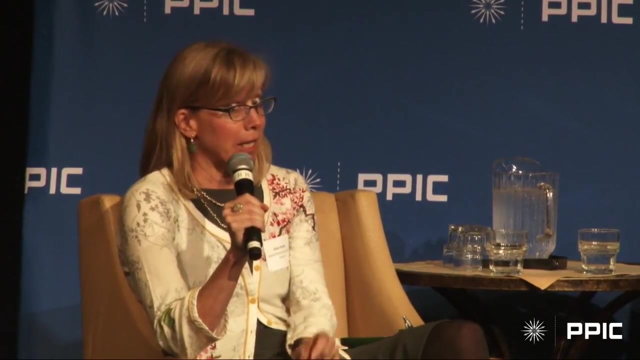 almost a decade now and haven't yet called on some of those other laws to replace. the emergency room that we're operating in is a big problem. That said, the ESA has acted as a necessary stopgap measure To stave off extinction, which we've managed to barely do so far. but you know I sat in 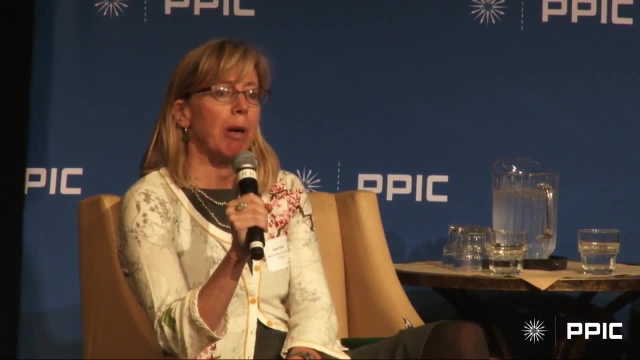 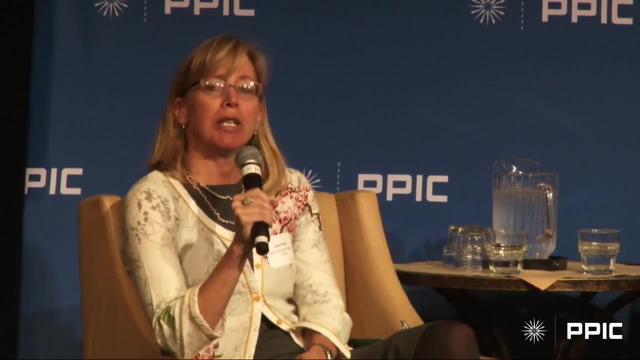 a courtroom in 2007 when a number of very respected biologists, including Peter Moyle- not the real Peter Moyle- said, you know the Delta smelt were likely to go extinct within a year. So they're not yet. 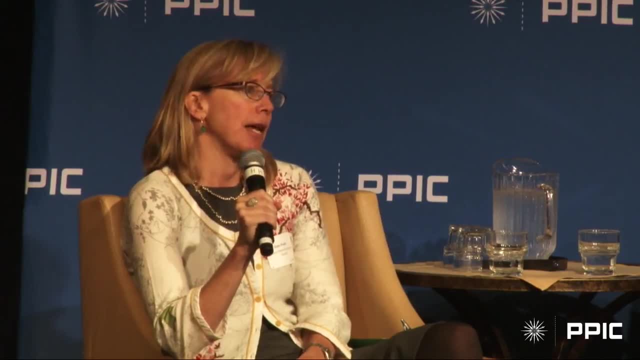 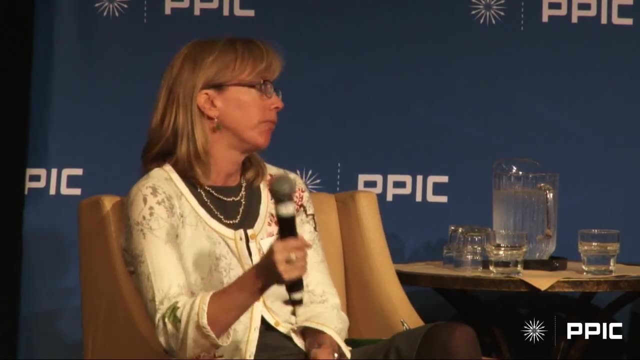 We need to do a lot better, But the ESA is a necessary but not sufficient measure, Part of the puzzle and we need to call on many of those other laws And Phil your thoughts on. are we succeeding and if not, why not? 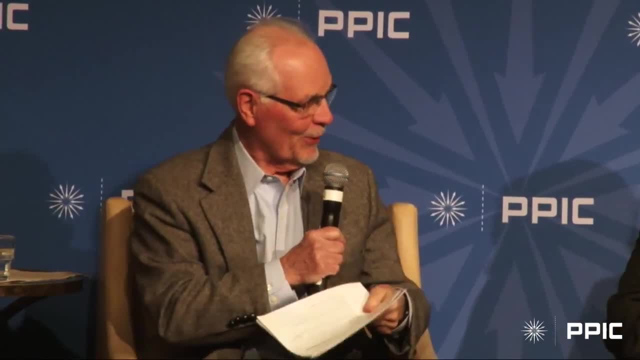 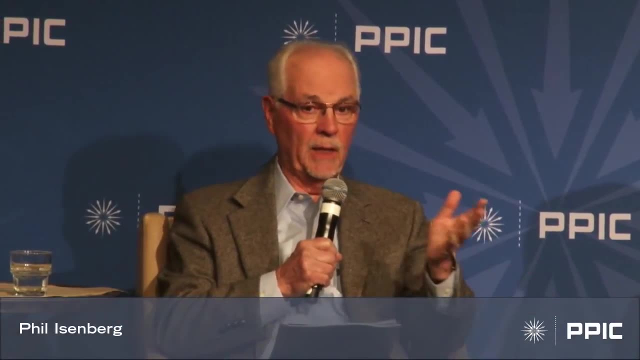 Well, the answer is: you have to set the goal you want to reach first before you can decide failure. And since all of us spend all of our time setting different goals, ignoring the laws we don't like and only talking about the laws we do like, it's really hard to figure out. 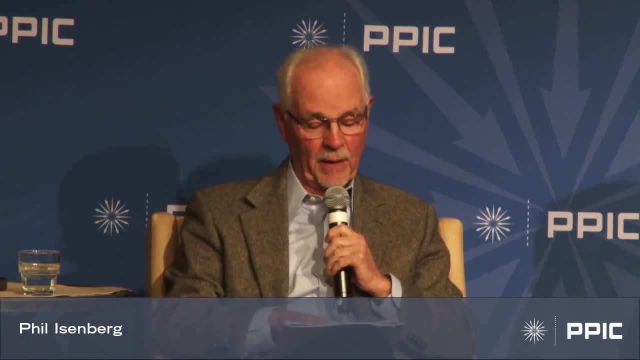 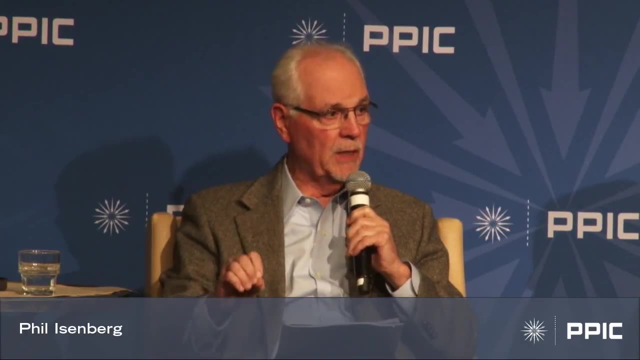 how to answer that question. So we'll go at it a different way, Because the environment is still a junior partner in the actual actions of the federal government, the state government and local water agencies in California, in my opinion. By the way, I speak personally at this conference today and for no one else. 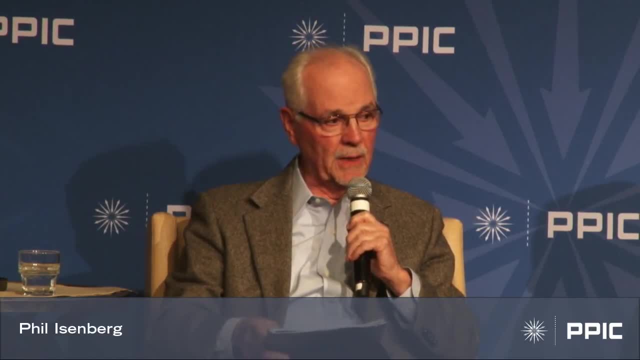 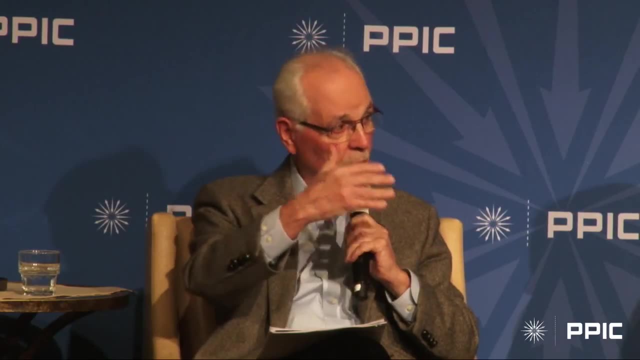 So the answer is: as an inheritor of all of the things you talked about was the early days of water development and the destruction of urban areas. it's really hard to tell if it's failing. It's not going to go any further than we thought it was. 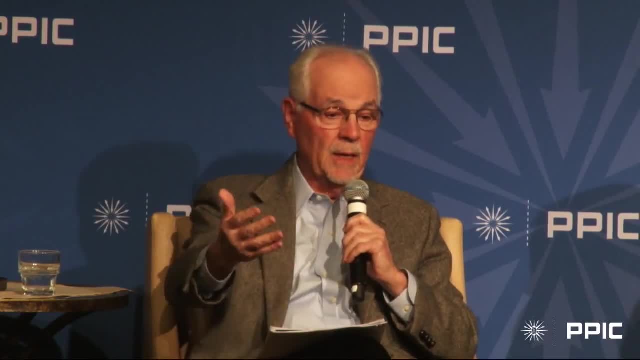 It's going to be a great challenge, But the major issue is it's going to be a very, very short-term decision of the environment and wetlands and so on, the Clean Water Act, the Endangered Species Act at the federal level and everything else. 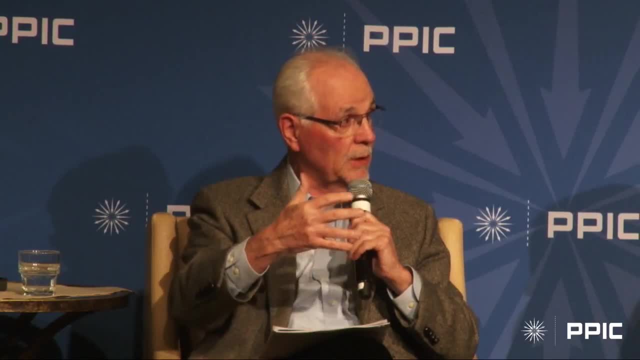 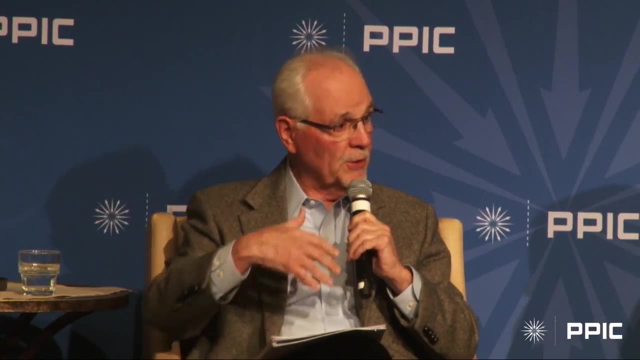 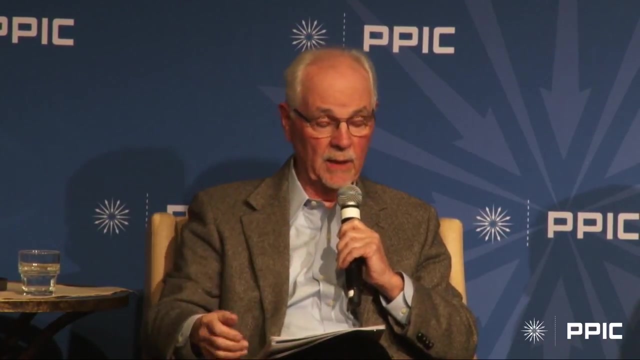 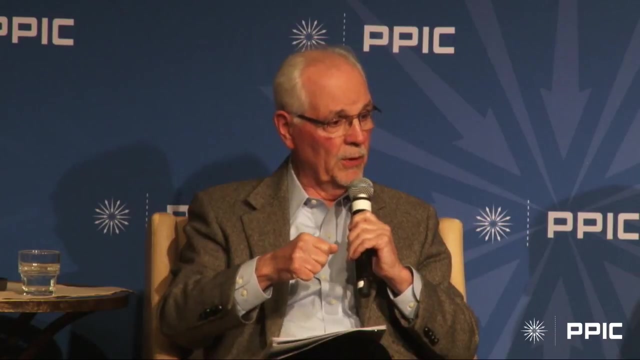 was the first wave of major reaction to what is now mostly conceded as being a bunch of actions taken for human purposes, where nobody paid much attention to the consequences, the likely consequences. But it doesn't mean that we've advanced to the point that California law now requires. 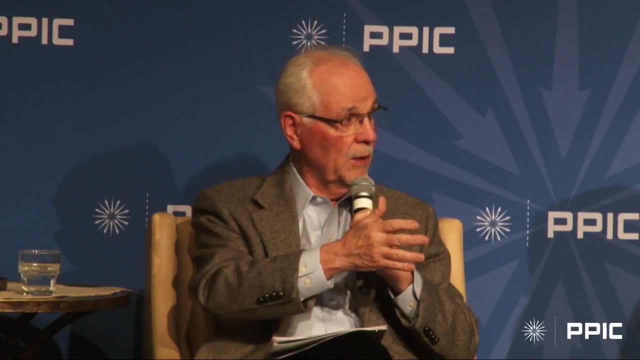 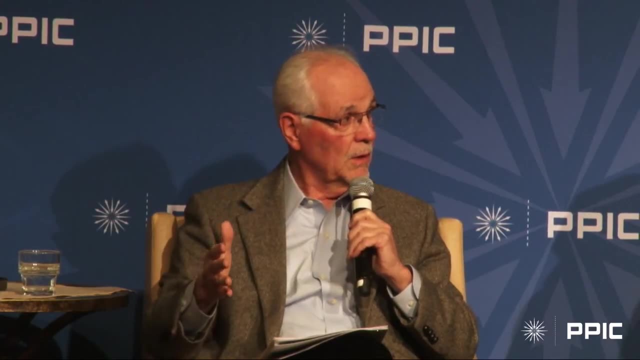 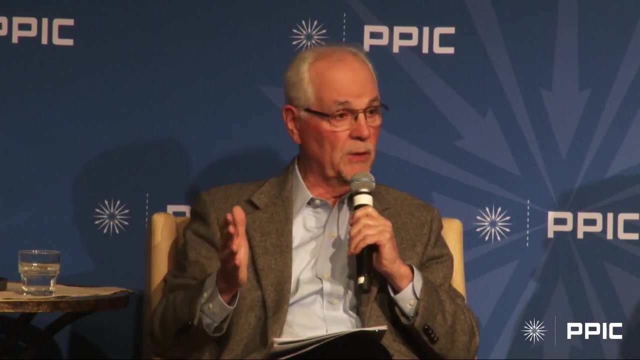 which is co-equal status, at least in the Bay Delta, for environmental protection, restoration of the delta and a more reliable water supply for California, in my opinion, And that's of course, because even people who supported the 2009 legislation 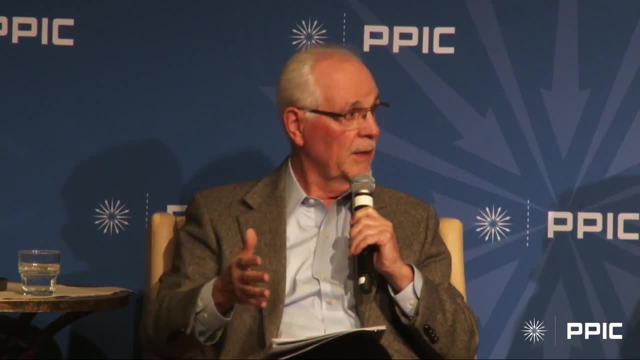 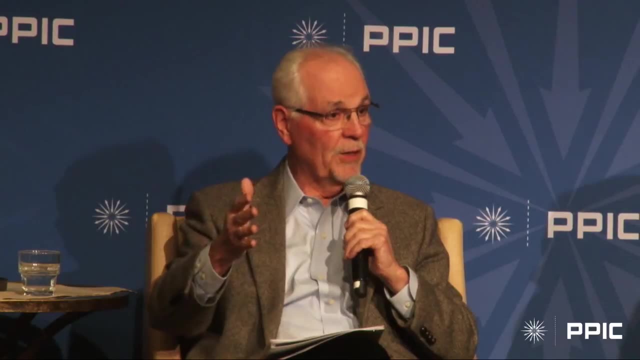 aren't happy about seeing it applied. Laws don't enforce themselves. You can, and we've got a history in California of hundreds, probably thousands, of laws in the water field promising water to every activity of human beings, either directly or preferred activities that they favor. and you add them all up. 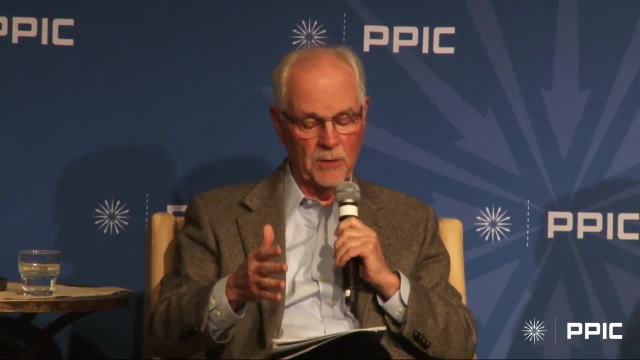 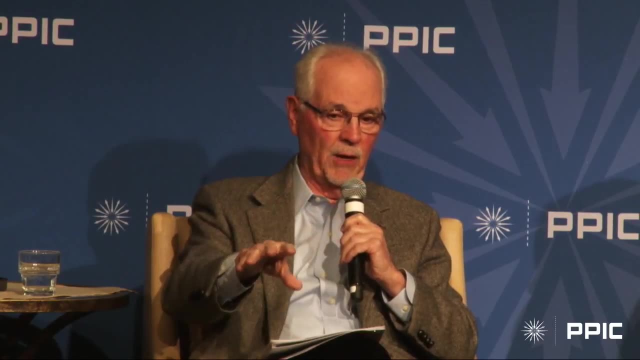 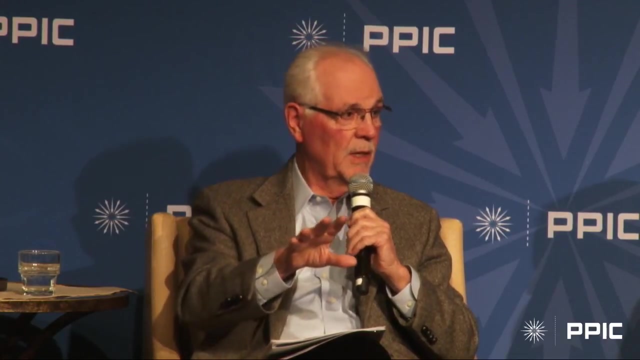 and it exceeds the available water on a pretty regular basis. So subsidiary question: Is the Endangered Species Act, a species by species Species evaluation- really a good idea? if you're talking about ecosystem management, No, it isn't. Never heard any serious scientist argue. 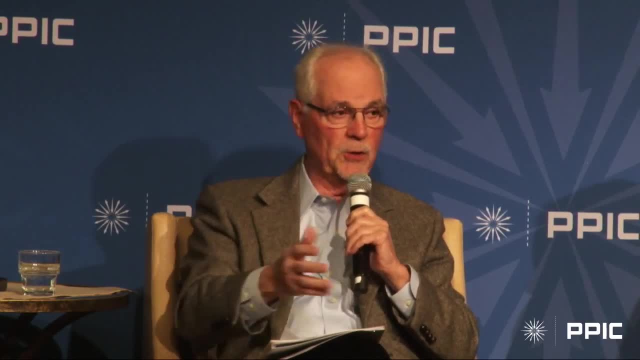 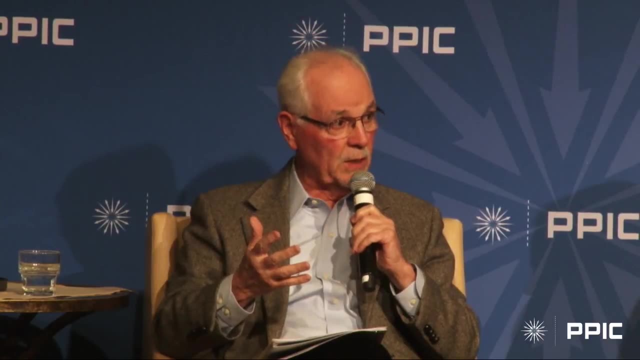 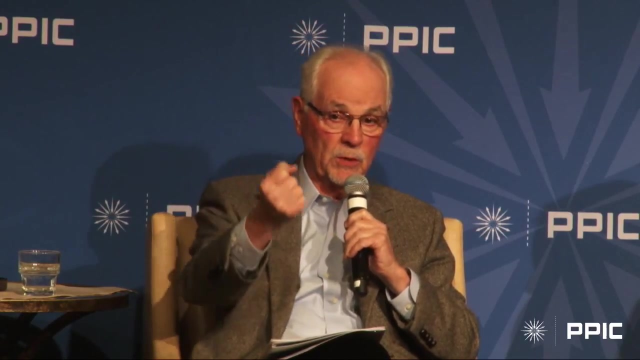 that it is a great tool for multi-species, habitat, water and all the other ingredients that go into an ecosystem, But at the same time, in the political context, it is one of those few things remaining that forces governmental agencies and private parties to pay attention. to what ostensibly is legally now a co-equal goal. And just to avoid any misunderstanding, I always thought, for all the problems the Bay Delta Conservation Plan had, they had a major statement of giving protected status to a very large amount of land, up to 150,000,. 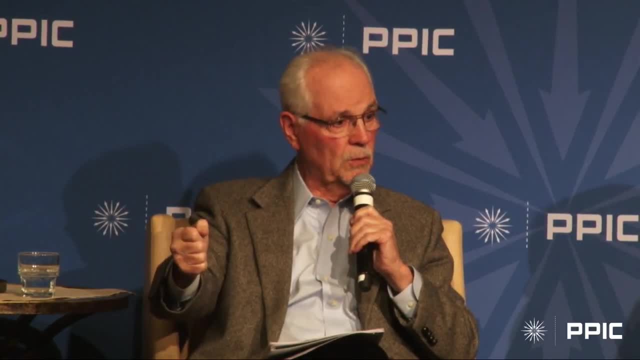 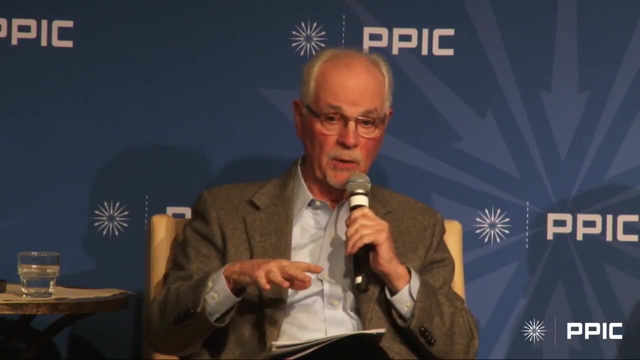 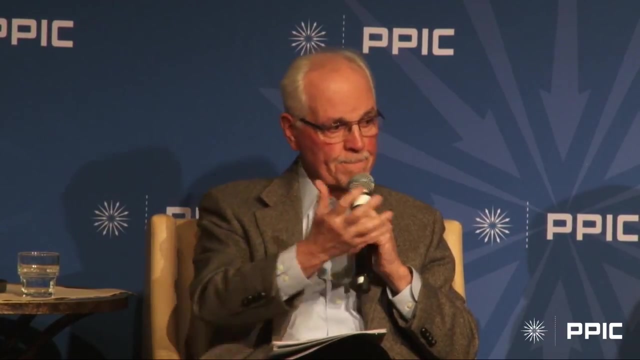 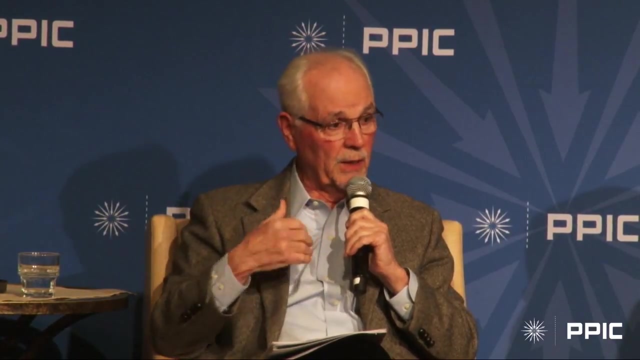 acres. Shifting to water fix has retained the magnitude of the tunnels but decreased the amount of conservation and restoration, And it's hard to visualize how that's going to work over time, consistent with the co-equal goal. Personally, I always thought that 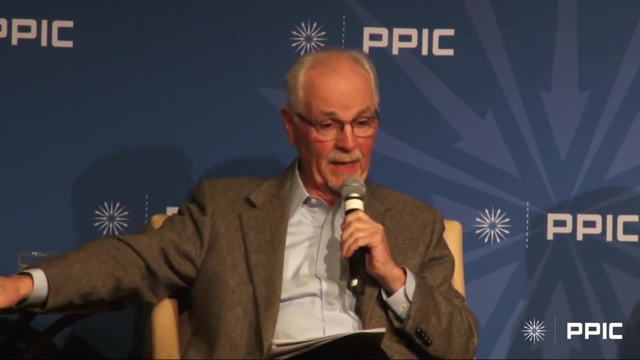 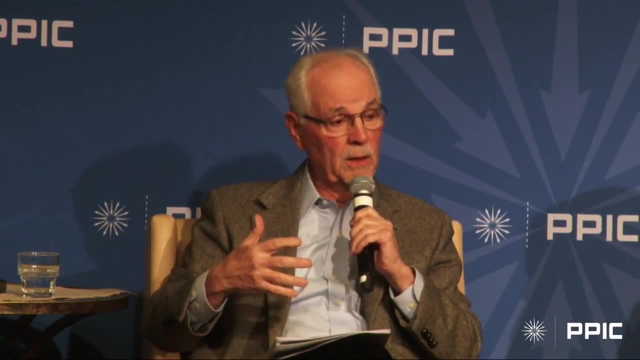 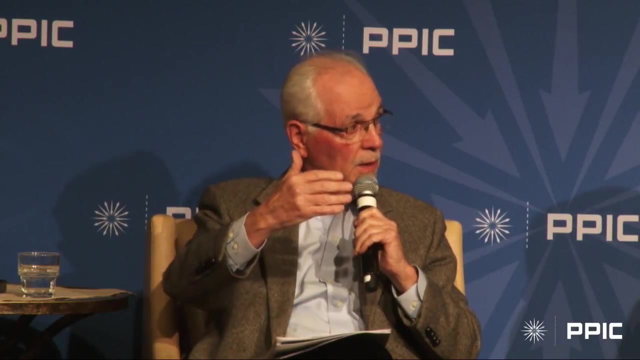 if the problem, if Kate and the water, the water contractors, could get together and work out some general thing, you might have gotten federal and maybe federal but state authorization to try general ecosystem management through what was then the Bay Delta Conservation Plan in a more meaningful way. 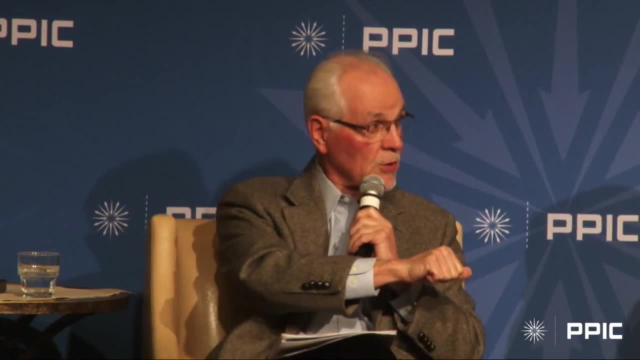 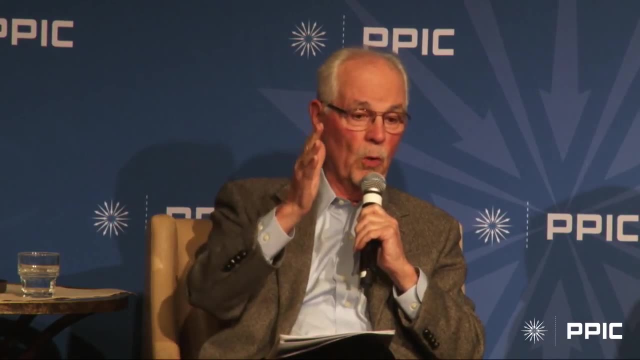 Now that requires the involvement of scientists with decision-making authority, not just the ability to comment, And it involves serious and substantial amounts of money And it means that water operations are merged with the decision-making on ecosystem. But that opportunity, I think. 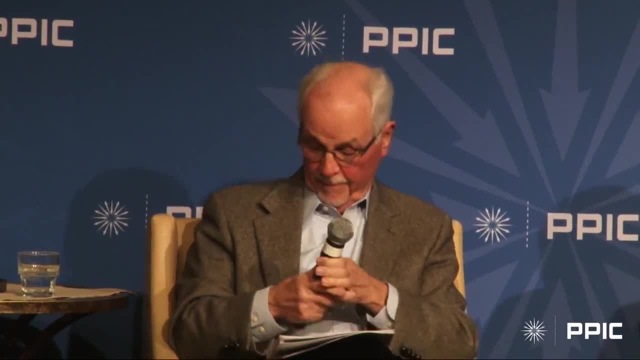 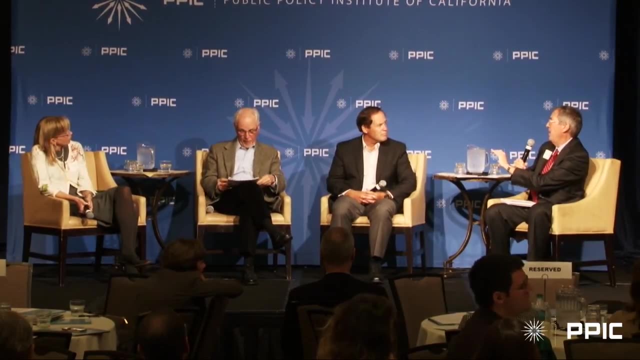 has been lost for a while, although it's worth thinking about. Okay, so let me see if I can summarize here. I think I hear actually all of you advocating a broader, more ecosystem-based management structure, But right now, the key environmental act. 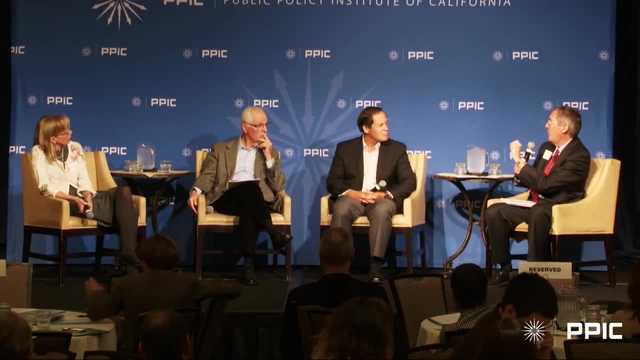 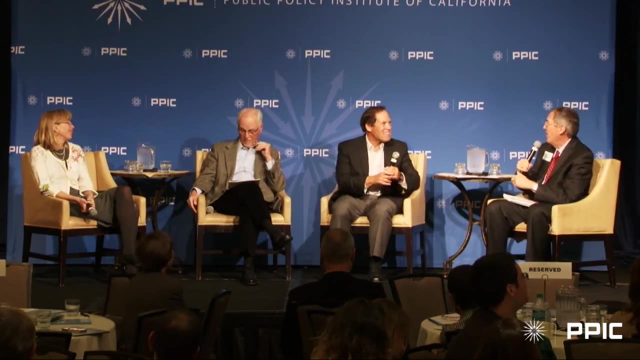 the one that has the teeth is the Endangered Species Act. So thoughts as to how one actually moves from the Endangered Species Act, which understandably is the focus of environmental attorneys, to this broader ecosystem approach. So, Jeff, you brought it up to begin with. 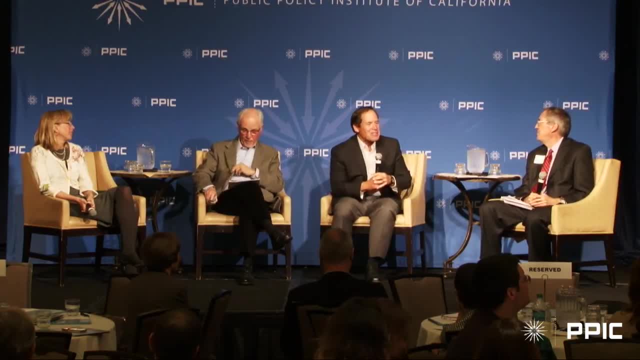 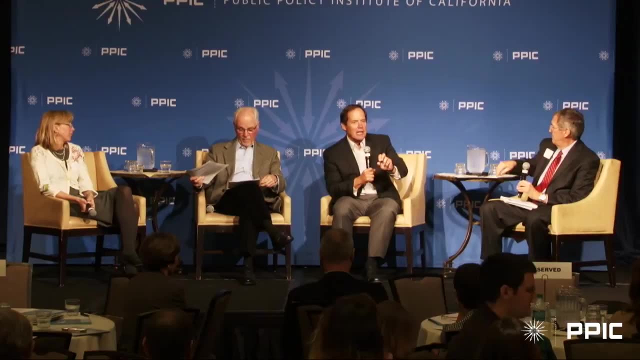 I guess I did Okay, so this again. for many of you this is an unwieldy document and I don't advise it unless you need some sleep. And that is to go into the state board's description of what they want to do in the San Joaquin. 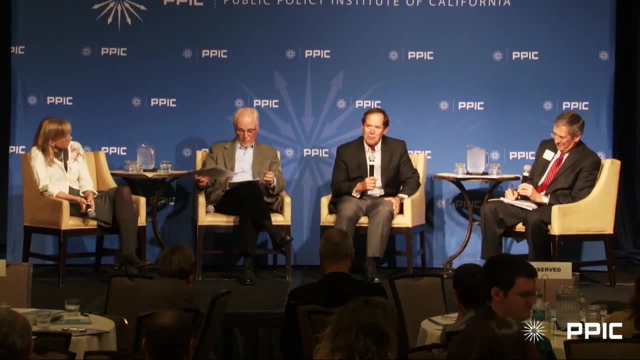 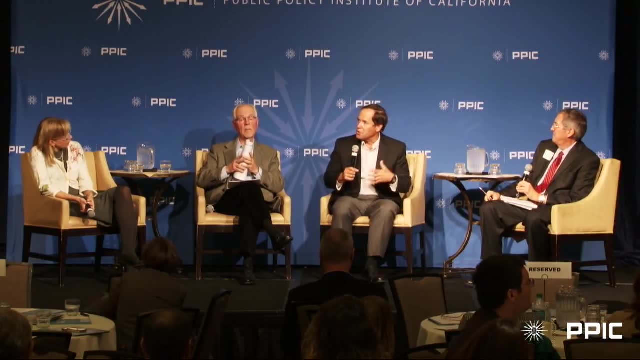 And what we miss in there is that what they're proposing to do. I mean, most people are focused on the fact that they want to increase the amount of water for the environment. So, essentially, the notion of the staff recommendation of 40% of the unimpaired flow. 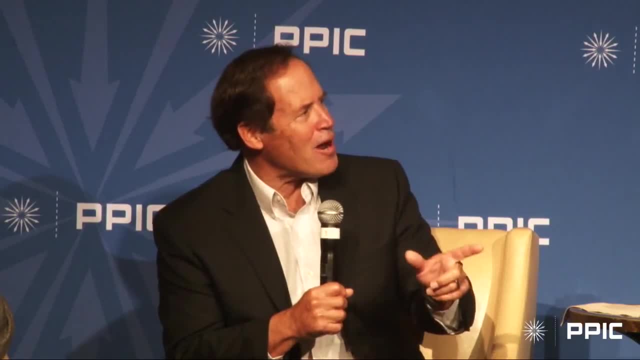 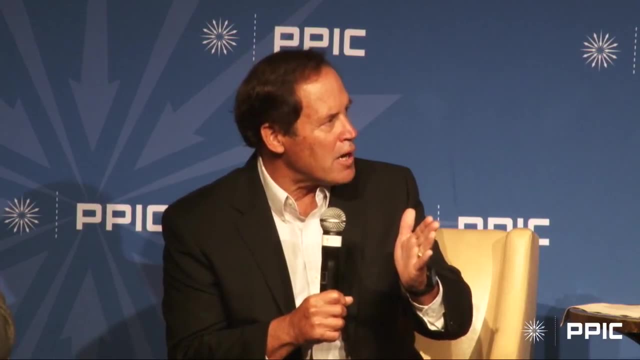 But look, read it closely. What they're suggesting in this- and I thought this was actually why I thought it was so intriguing- is it isn't 40%. specifically, It is an allocation of water of the unimpaired flow. 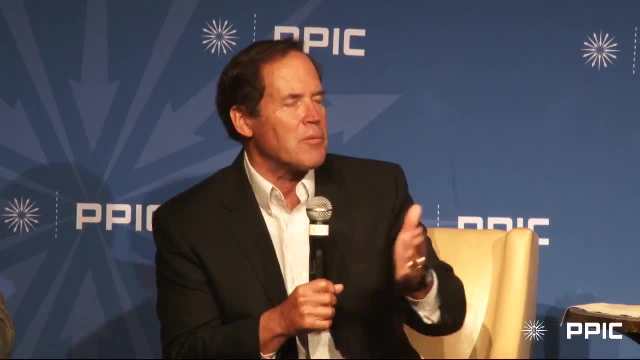 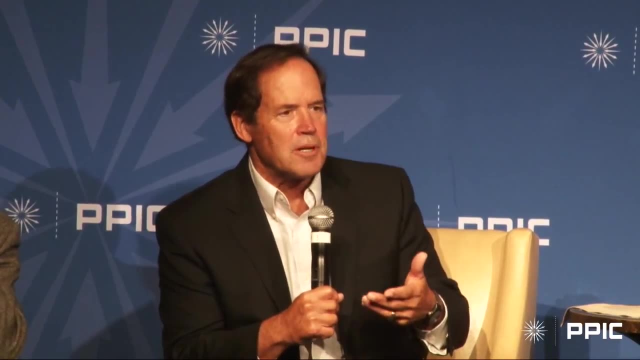 which can be flexibly made. It can be managed at least in the period February to June. So it's a baby step in the right direction of something we have been pushing now for some time in this notion of allocating water to the environment. 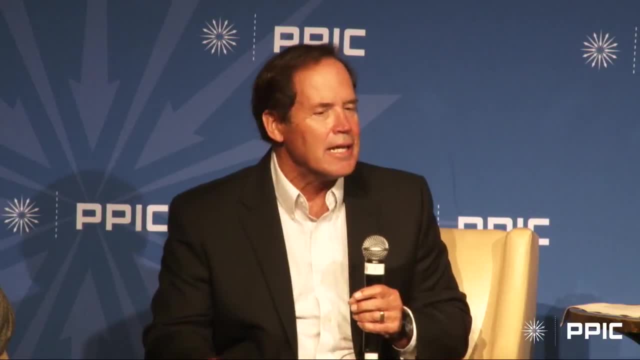 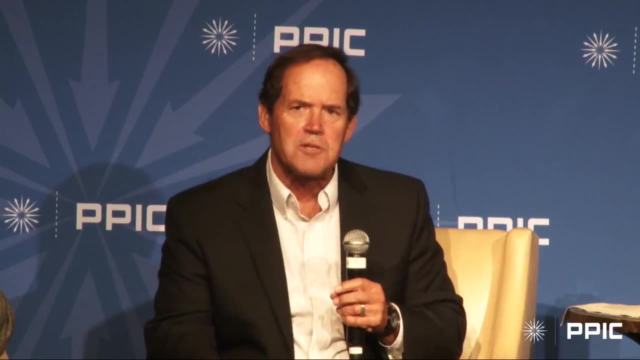 and creating the ability to flexibly manage it. I am greatly influenced by what happened in Australia in a very different way than most of you are. Most of you focused on what happened in the urban management, the environmental management in Australia during the drought. 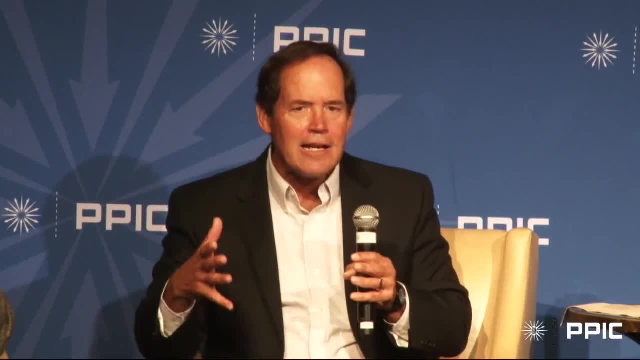 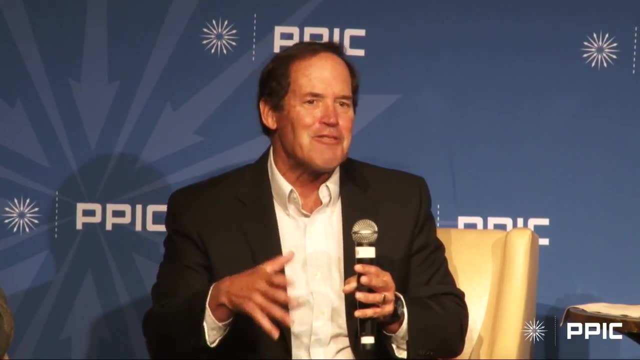 What was so striking about it is that they allocated water to the environment and gave the environment the tools to flexibly manage it, And so the environment became a partner, which is what I'm after here, Instead of a constraint, which is the way we currently do it. 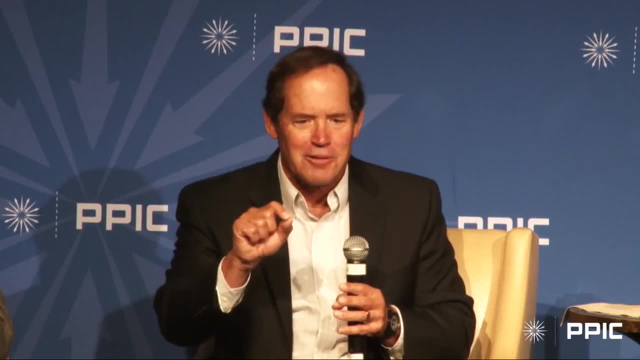 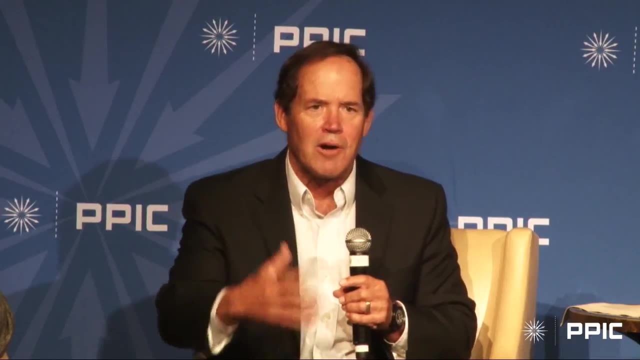 the environment became a partner. So, in that now, mind you, I expect the process, the political process, to chew up a lot of what the state board is proposing to do. Indeed, the state board has said: go out and you all do settlements. 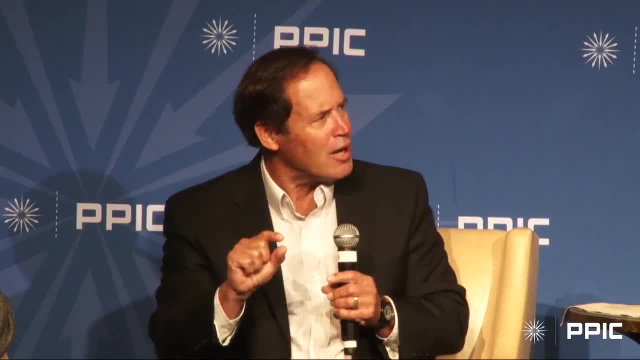 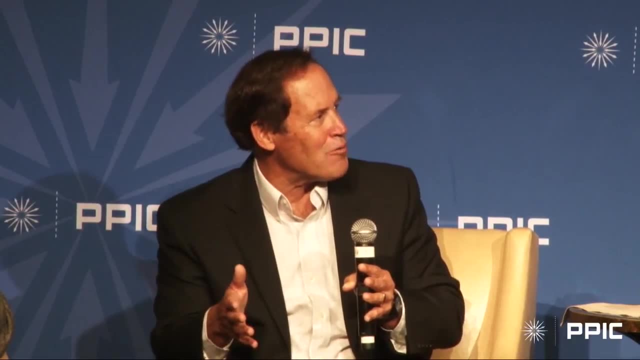 and come back to us with your settlements, And there's the germ of a really good idea in there and essentially it represents an allocation that can be managed as an ecosystem in the San Joaquin Now, where we could probably get a really good argument going. 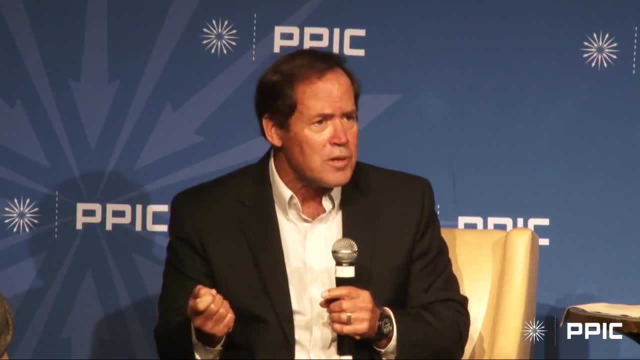 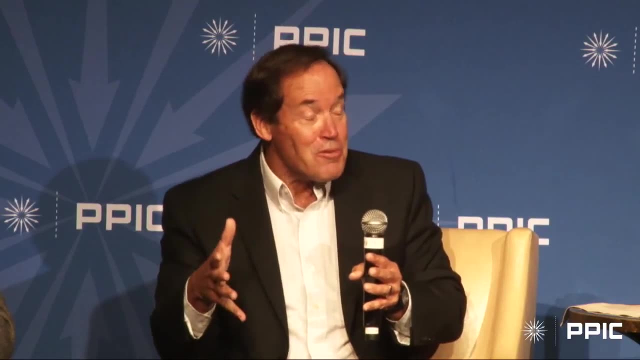 is what that ecosystem ought to look like and what its functions would be, and whether it's dedicated principally to steelhead and fall run Chinook salmon. But the fact is there's the germ of a really good idea in there and I'm sure members of the state board here. 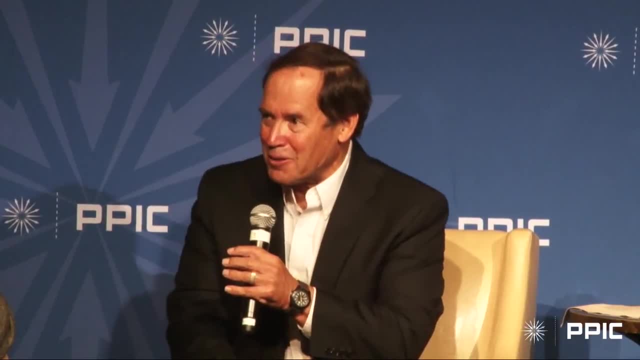 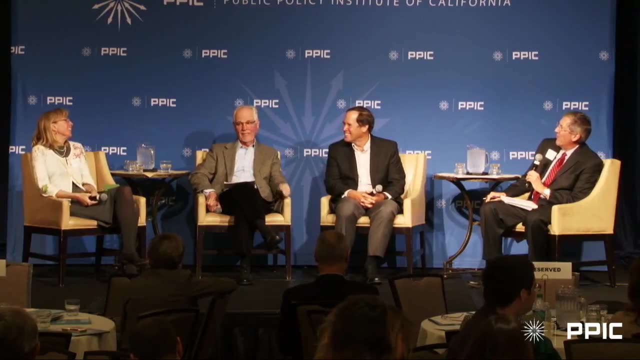 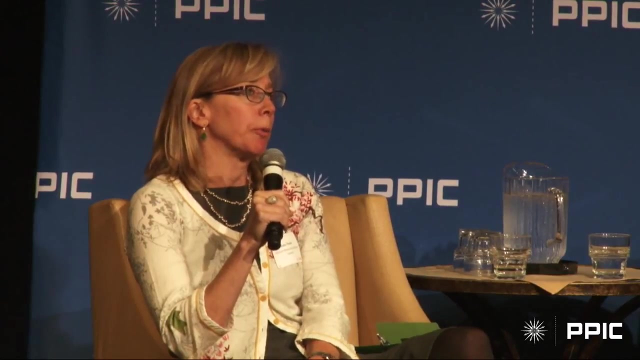 are shocked to hear somebody saying something nice about them. So, Kate, you've been involved in the San Joaquin effort, so do you share Jeff's views that this might be a very important approach to utilize? Well, I think the state board's San Joaquin Flows proposal. 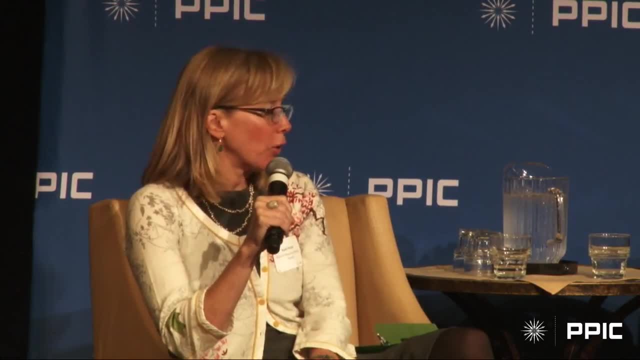 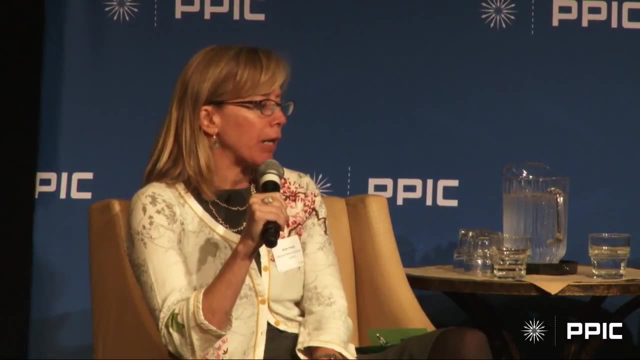 that's on the table is a marked improvement over where we have been, and it's a much better, I think. way to put it. It's a much better, I think. way to put it. It's a much better. I think way to put it. 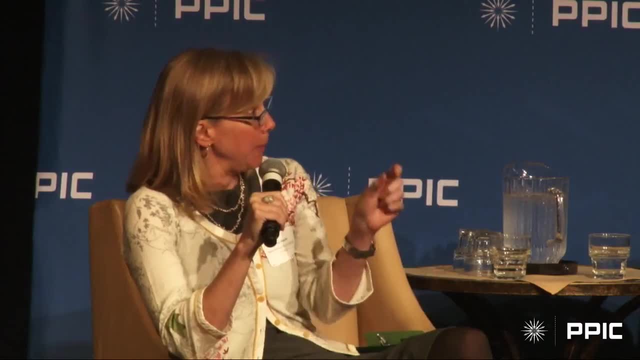 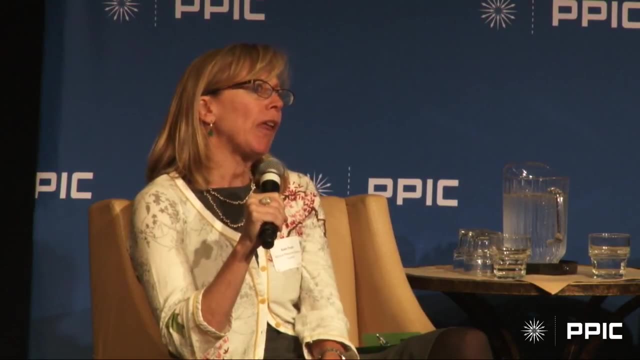 sort of more holistic approach than the ESA approach, the species-by-species approach we've been using. So for that reason I think it's, you know, a much better management tool. I'm not quite sure what Jeff means when he talks. 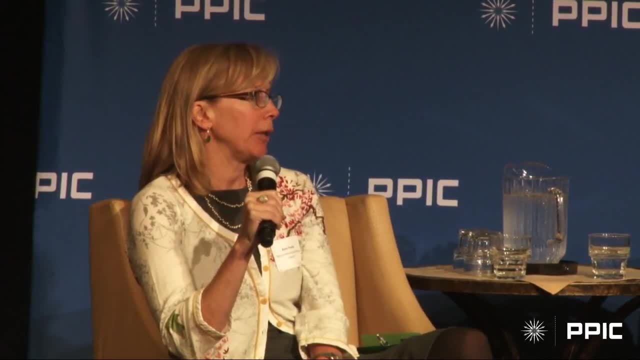 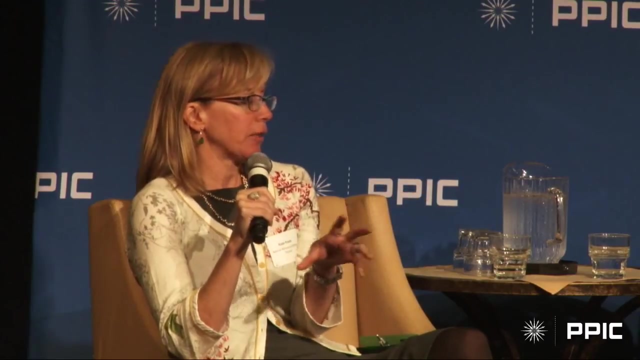 about a water budget, and what worries me about that approach is that I flash back to the early 2000s, when we had the environmental water account under CalFed, and what that essentially did was constrain made them feel like there was this set amount of water. 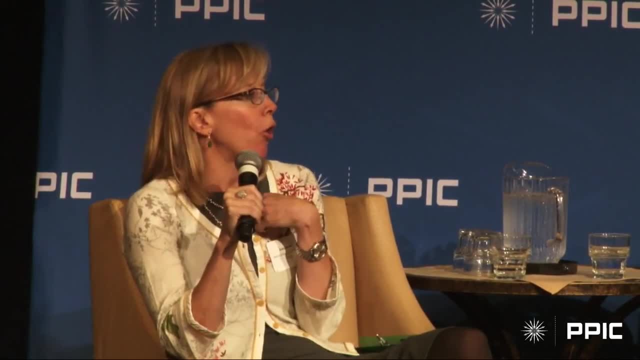 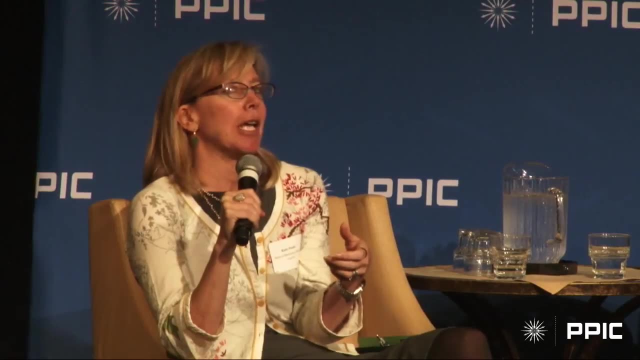 that they could use in any given year, and so they would hold back on calling for necessary actions- and this is all sort of laid out in a bunch of meeting notes, because they said, oh, we might need that water later in the year for salmon, or we, you know. 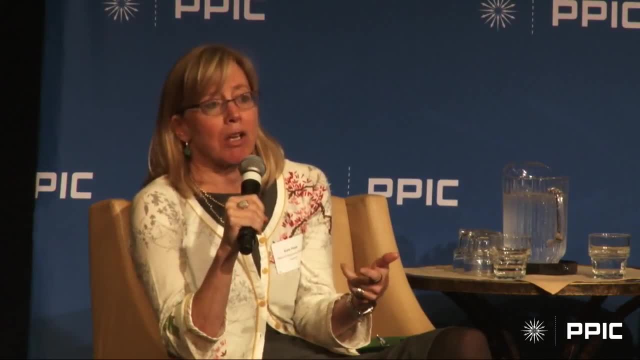 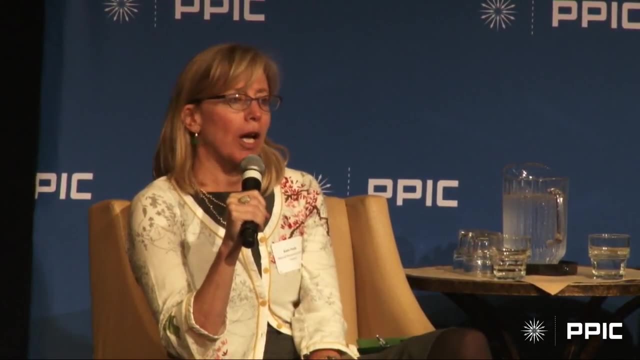 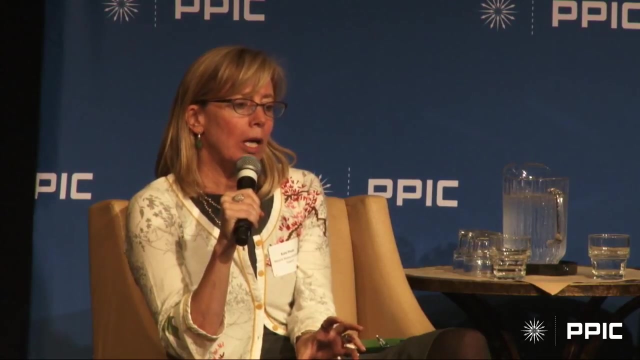 we might need it for some other reason And, as a result, the Delta ecosystem in particular went in the tank. so That's a bad approach In terms of sort of being more flexible and being able to allocate water where it's most needed. 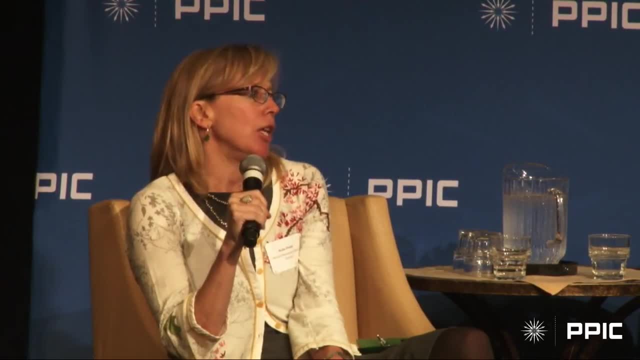 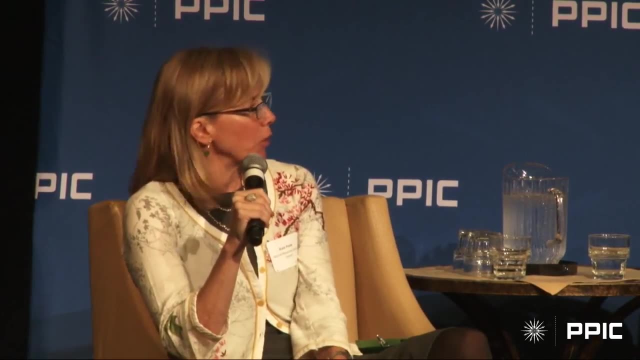 when it's most needed at the right time. you know you can't argue with that. I think that's just sensible and I'm not sure that anybody is proposing something different than that. So, Phil, your thoughts and I'm also curious. 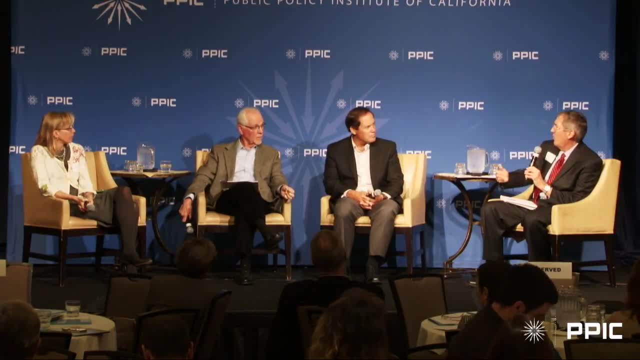 one of the things that a number of you have now mentioned is the difficulty of actually coming up with an agreement as to what it is that we're managing at an ecosystem level, and you've brought up the Bay Delta Conservation Plan. I have always thought that that the Delta Stewardship Council. 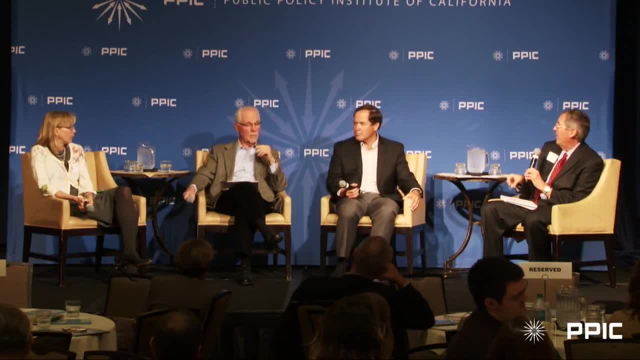 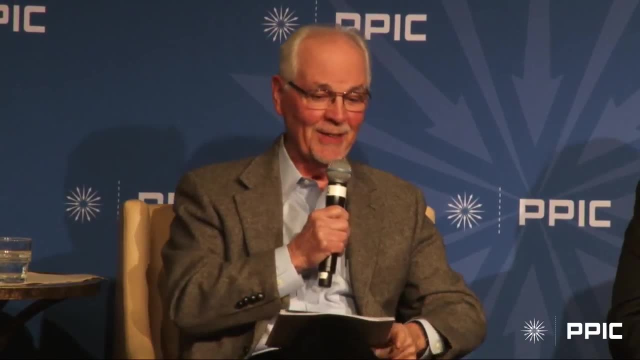 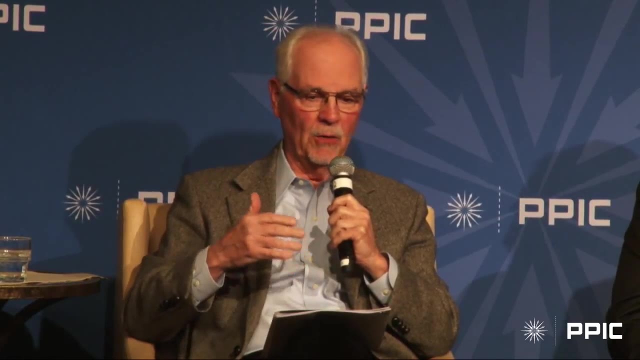 was really an approach that could get us there, but it didn't quite work. Going to show that you're remarkably insightful but very naive about the political process: Look, they Look for all America's talk about how self-reliant we are. 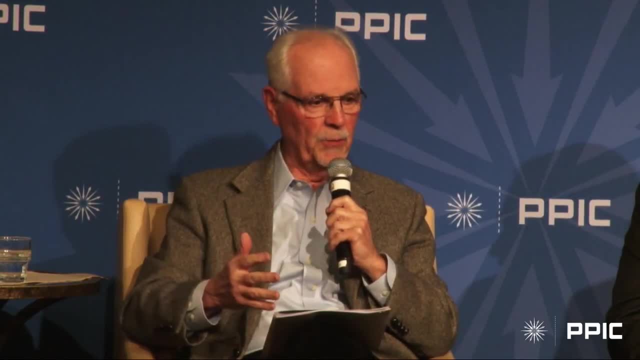 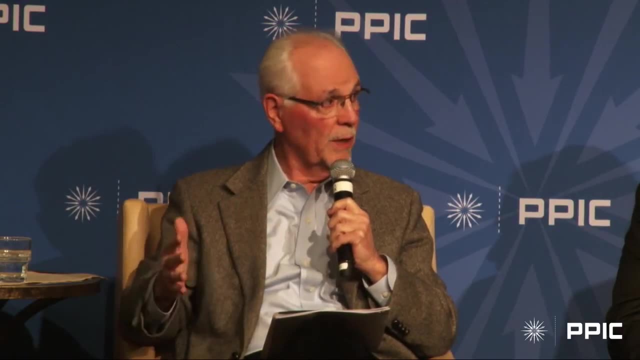 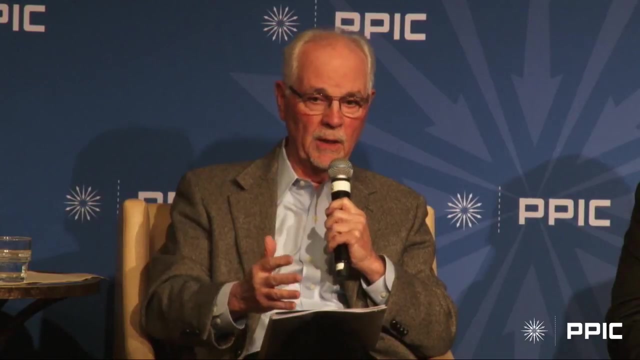 and how independent we are and how action-oriented we are, we actually, in my judgment, are risk-adverse and want someone, anyone, someone else to protect us from the risk of any change. So if the federal government, or if Karen, for example, 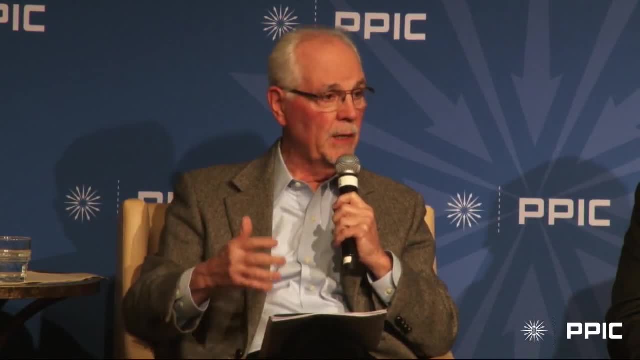 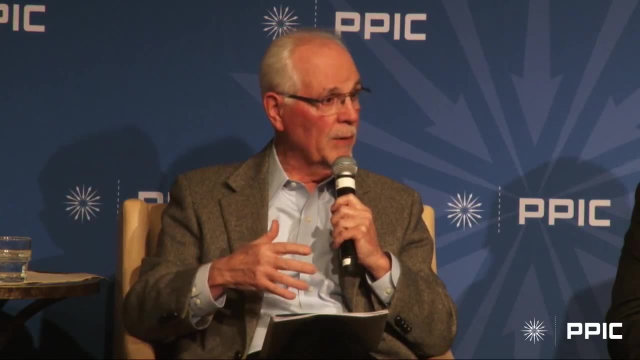 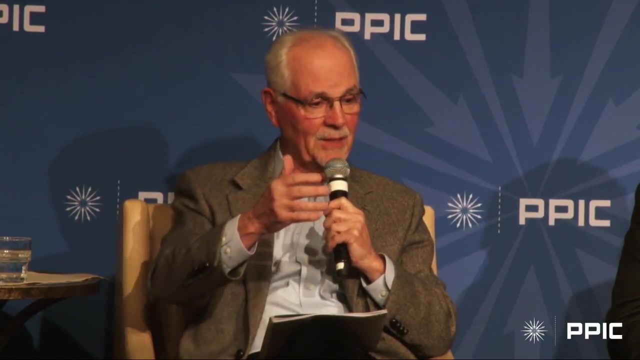 would stand up and announce that the state and the governor have now agreed to simply give trillions of dollars to anybody who complains about the lack of water. that would probably get a certain level of support in this room. It isn't exactly what I call a plan for managing water supply. because the reality- I've said this so many times, I apologize to most of you who've heard it before- The water supply is not infinite. We cannot supply water in amounts desired by everyone for everything every day, Just because you want it. 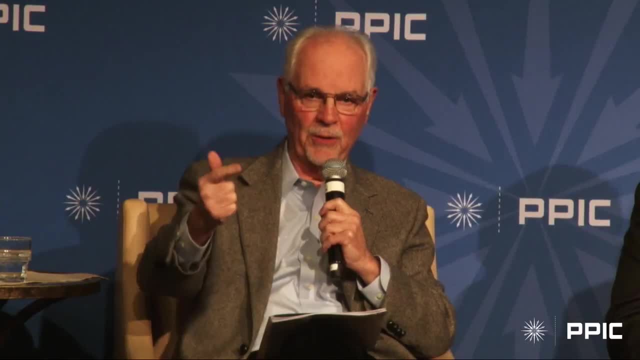 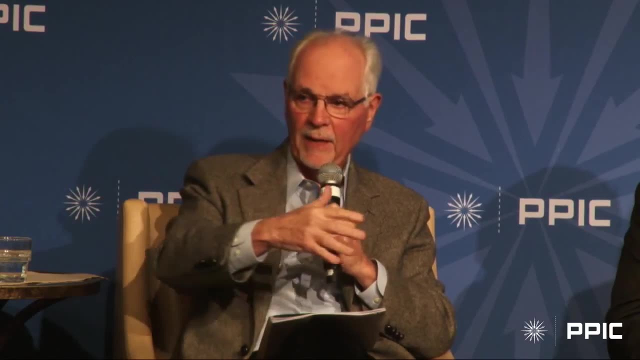 And it ain't going to improve, because the population's growing, the economy's growing. Even for the good conservation that's going on and the drop in per capita use, the fact is we're consuming more and more water And it's more costly the farther you go up the chain of these actions. 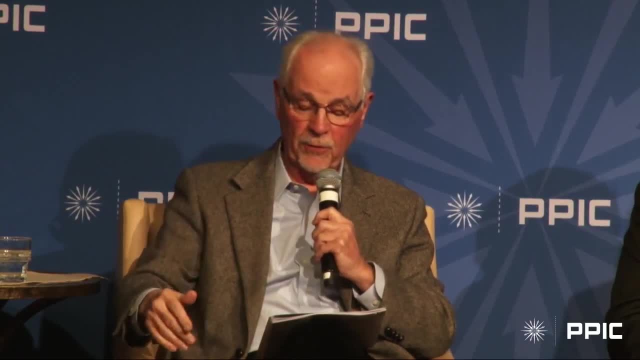 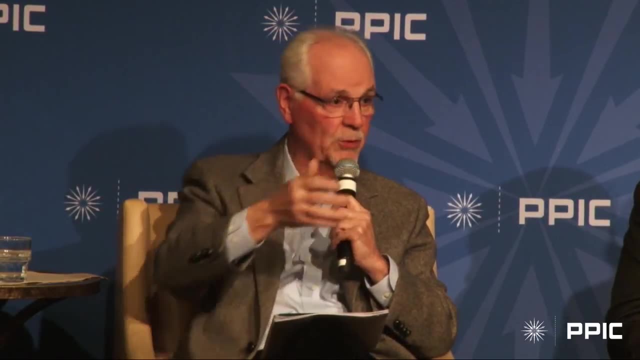 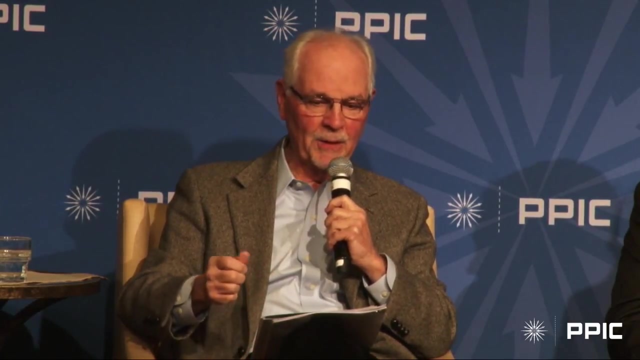 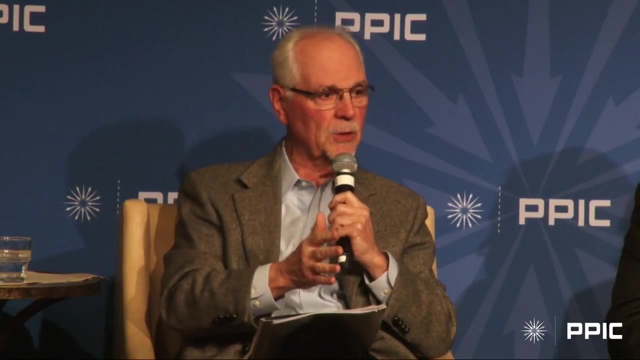 to generate reuse water for various kinds of things. I think the real dilemma here relates back to the conversation in the previous panel, which I thought was terrific. It was Sigma government public psychotherapy for water managers, And it's a continuing debate in American society. 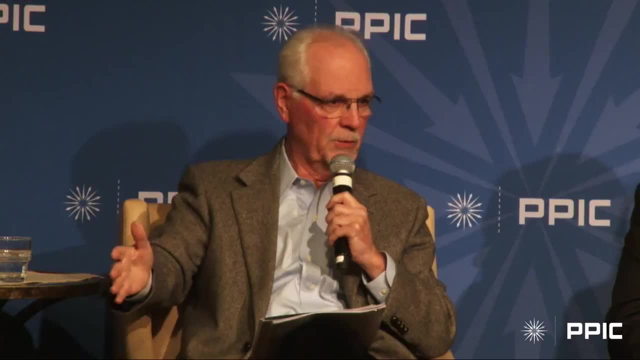 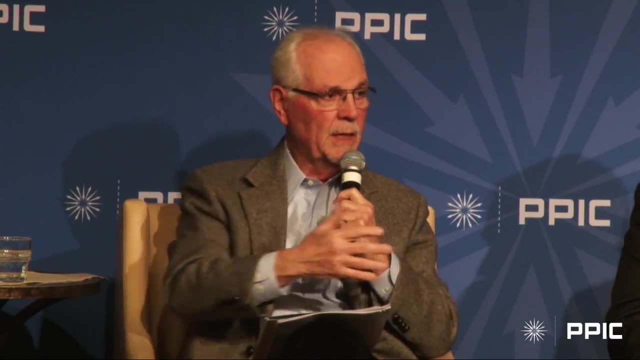 The preference for local control over evil federal control, but the constant desire to have the evil federal government give us all the money we think we need once we have the decision Now. I spent 11 years as a local elected official and 14 as a state official. 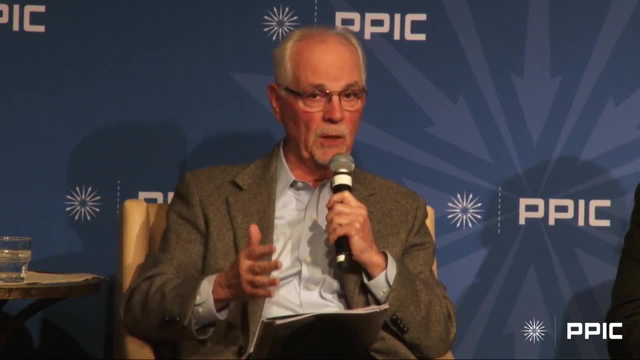 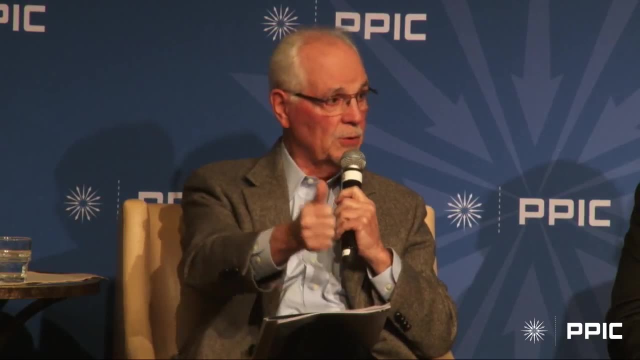 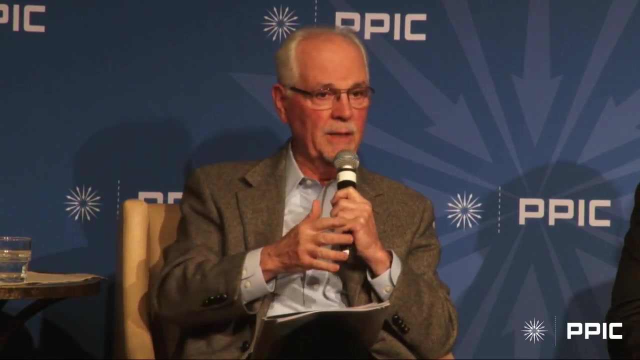 I see no higher level of courage on either between the state level and the local level of elected officials. on imposing taxes or fees, I found a general reluctance of all of my peers to do that and nothing has convinced me since that local officials are more brave. 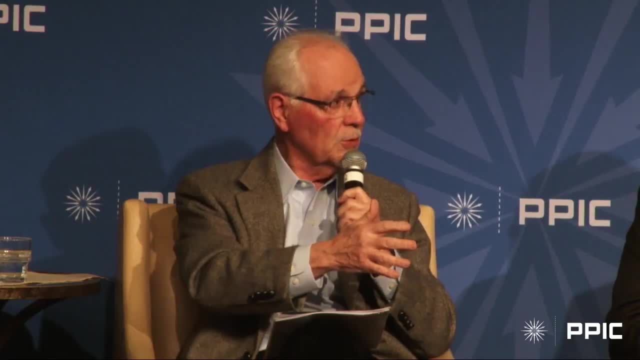 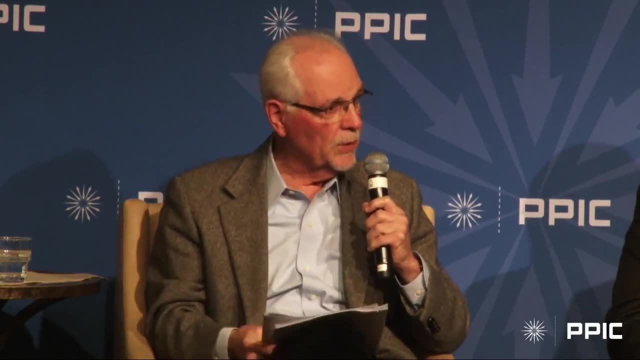 than state officials or federal officials. Matter of fact, Donald Trump has solved our problem. He announced there is no drought. Therefore, I don't know hell. is that the one? the last? well, the last meeting is solutions that really work right. 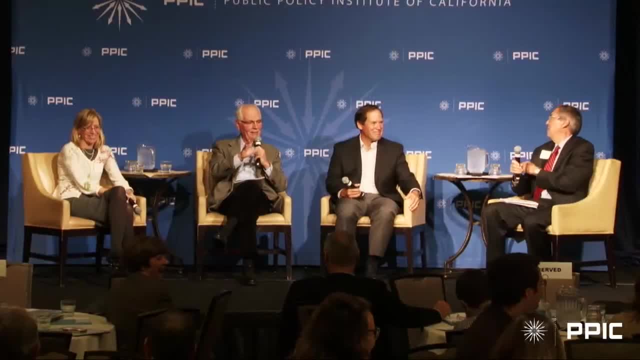 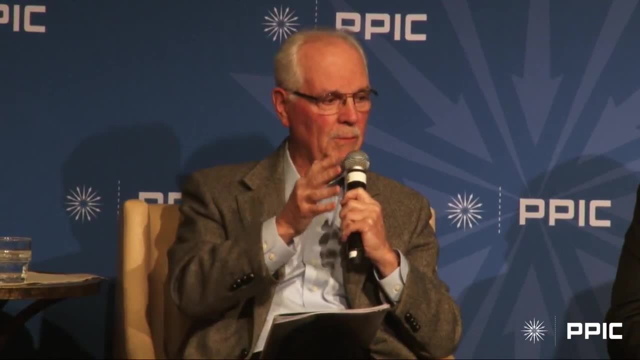 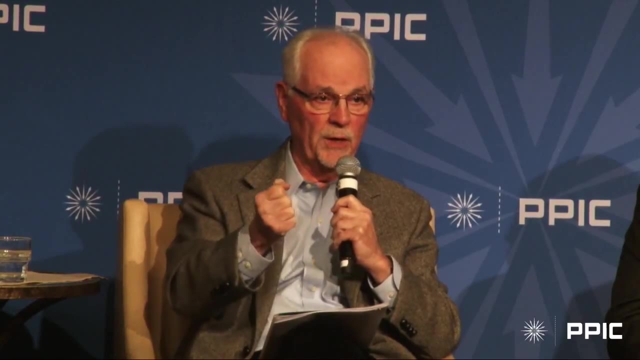 Okay. So look, I think, Buzz, I think what you ought to do on this one is think about the complication. At what point do human beings decide they have to do things they don't want to do, and are there things we could do to help, to encourage? 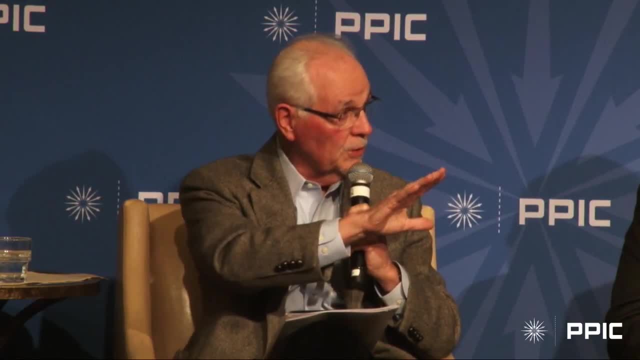 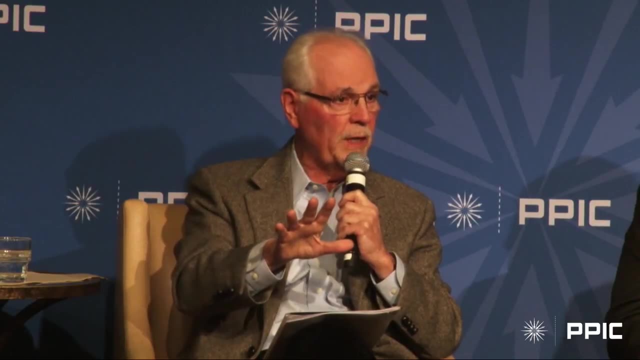 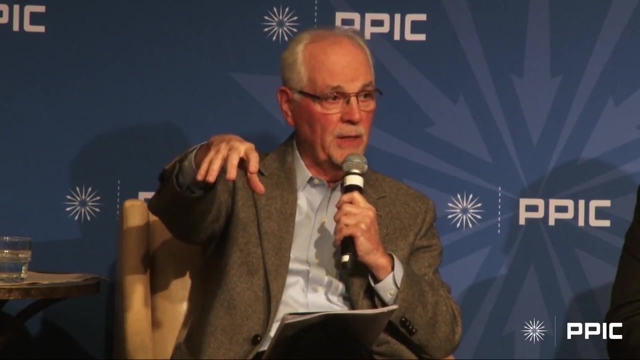 to encourage reaching that point. John Fleck's new recent book on the Colorado River, called Water is for Fighting About and Other Myths in the American West, is worth reading because it's the it's behind that threat and fear of independent action where you find that, God, you really can do things. 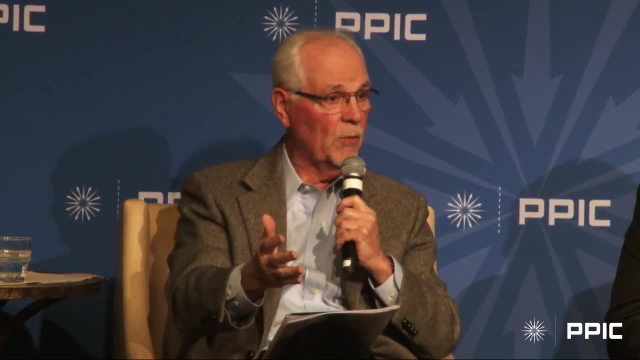 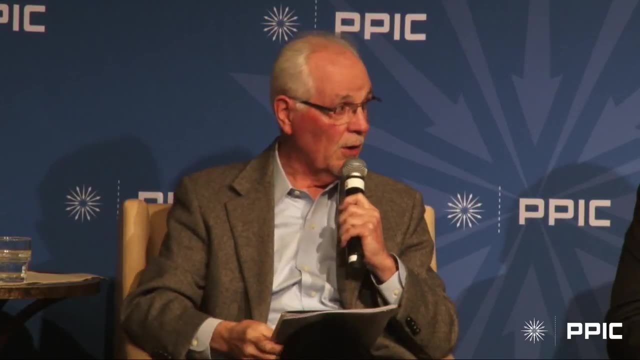 The first panel on urban water conservation. yeah, you can save a lot of water. Now how do you make other folks in that jump past the gap And I? that's an art form. It's very difficult to do. John didn't say it in his book. 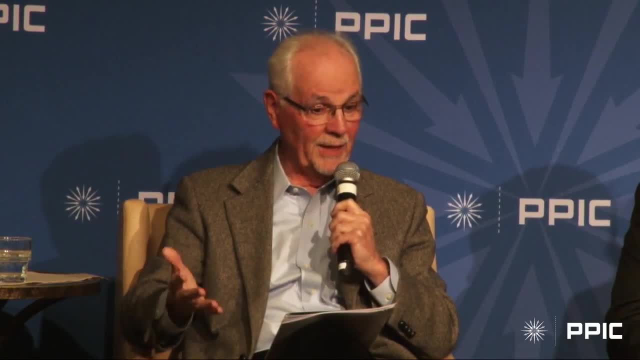 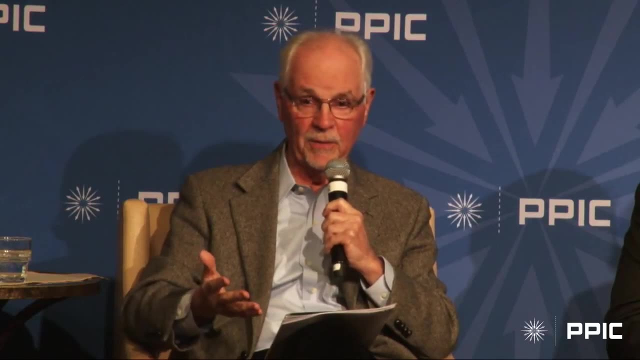 but it seems to me the intervention of the United States Supreme Court most lately in the 1960s had a lot to do with it, because if there's anything scarier than Jerry Brown, it's probably the United States Supreme Court. It may need, it may need, you know. 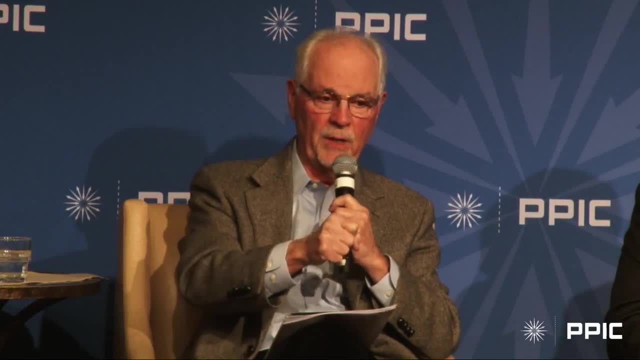 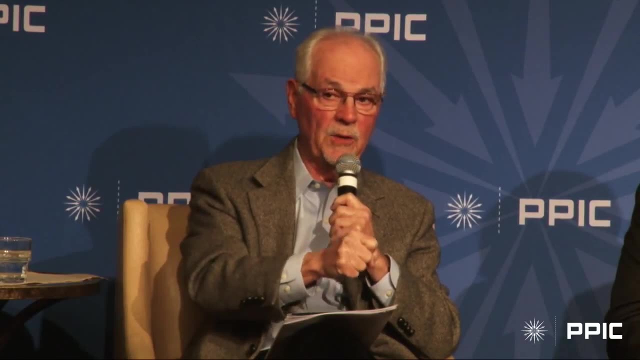 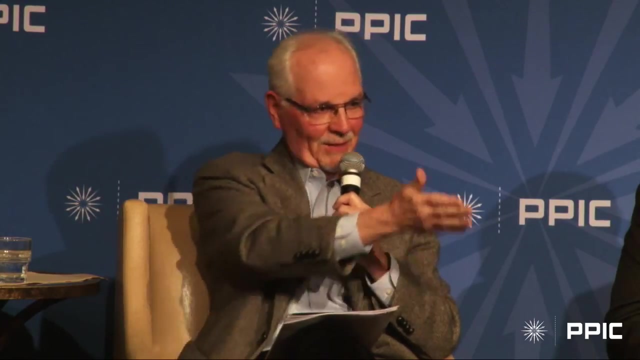 politicians are realizing every day that water is a terrible political issue for them because they can't deliver what their loudest constituents want. You know, because you're loud, the folks you deal with in the panels that yell at you for the first hour or hour and a half. 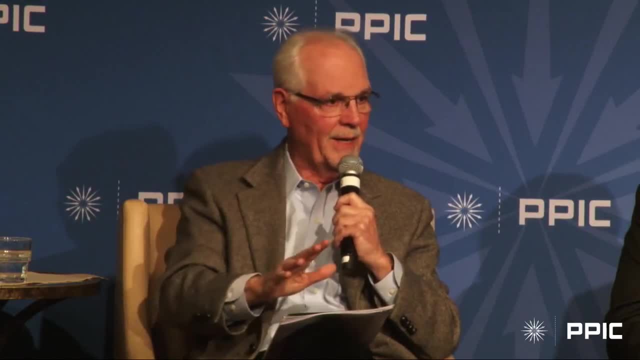 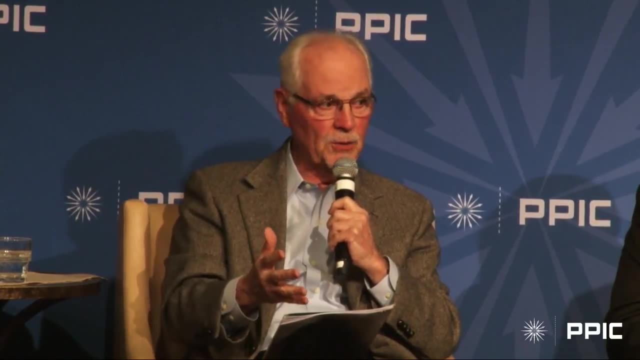 before you can talk to them on the issues. they don't care about any of the rest, They just want to be fully protected. You can't deliver that. No one can deliver that. Politicians are eventually going to want to turn some of these hard issues. 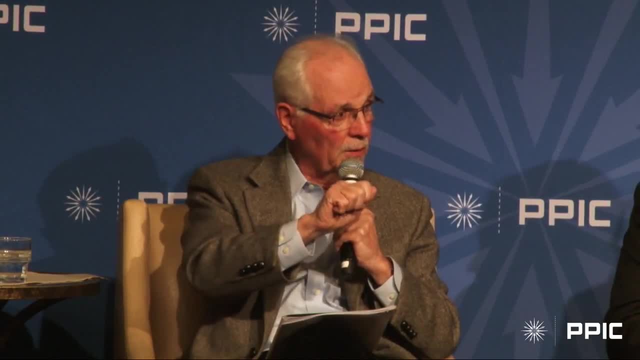 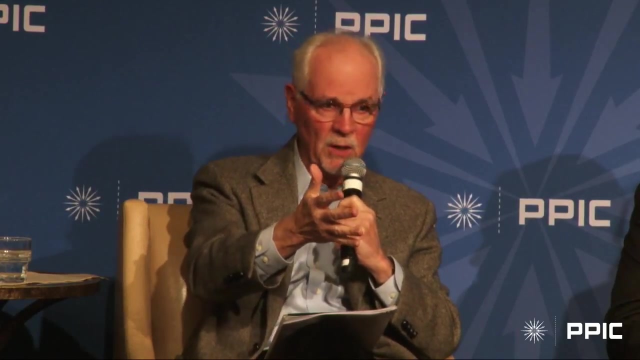 over to someone else, And one of the things that occurs to me is the Bay Delta could well afford to have a merged water and ecosystem operating system. I keep looking at the coordinated operations agreement of the federal and the state system. all these retired military engineers that push buttons. 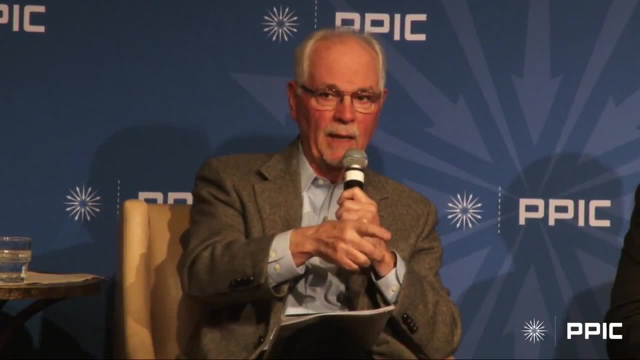 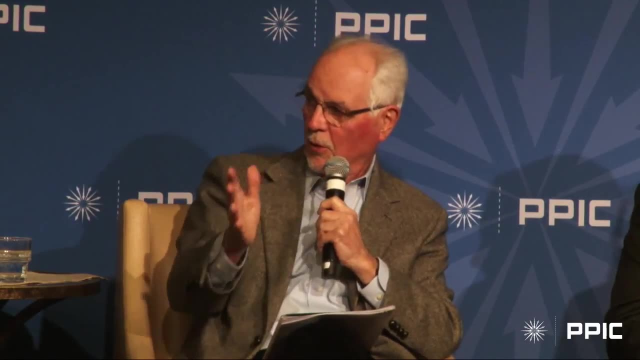 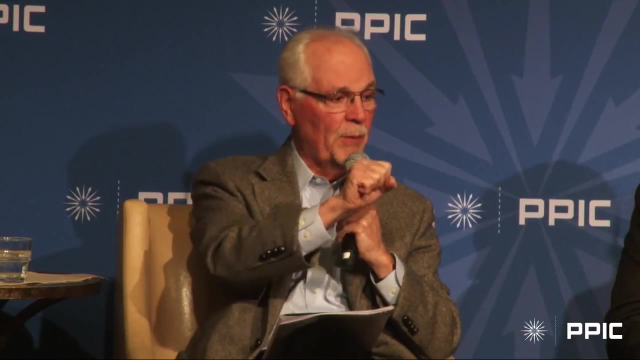 and you know they look like Thad Without the beard, And you know these. they just do what they're told to do, which is solve problems, And they don't like the politicians hovering around. Anyway, the purpose of politics. 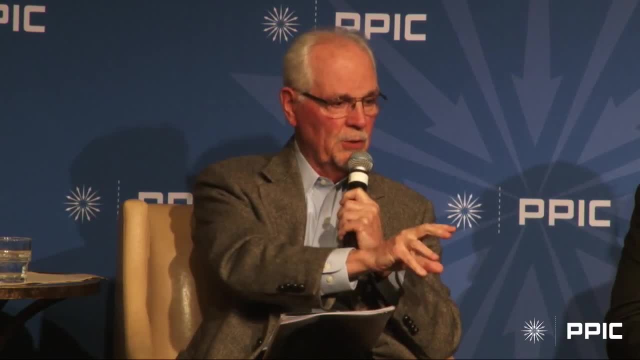 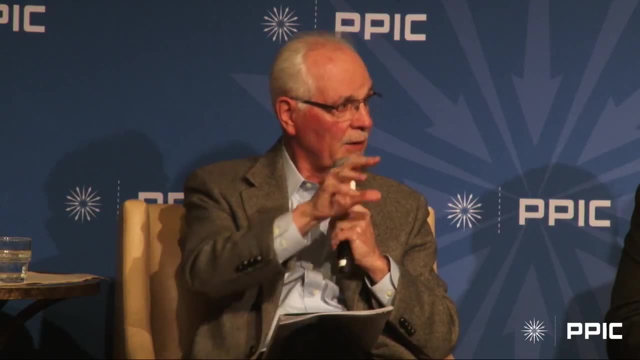 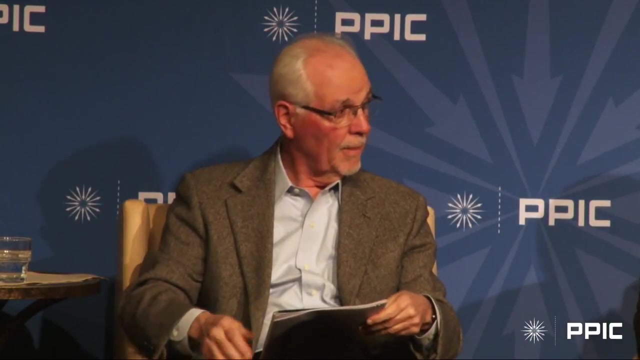 is to convert contentious social issues into boring good government. And that's what interests me: How do you take a contentious issue and convert it over time? So, Kate, actually I think this brings us back to you for a second, because one of the things I heard Phil say is: 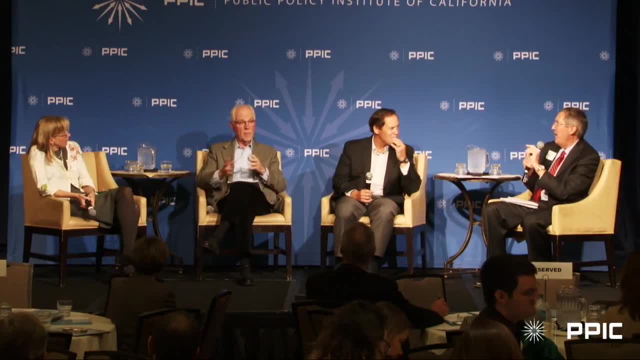 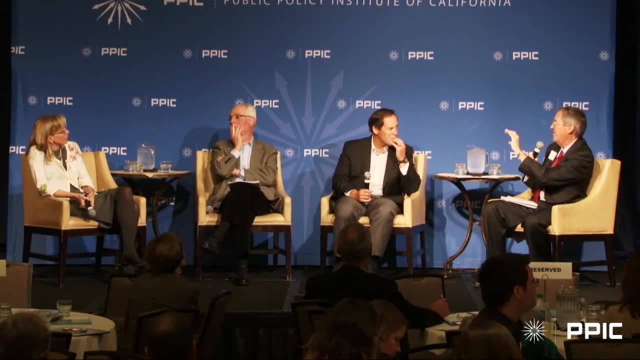 that there actually is a role for the court sometimes in providing that pressure that then good public servants can use to try to convert what is that contentious issue into something which actually works. So, from that perspective, any thoughts as to how we might be able to better utilize our current laws to get us there? 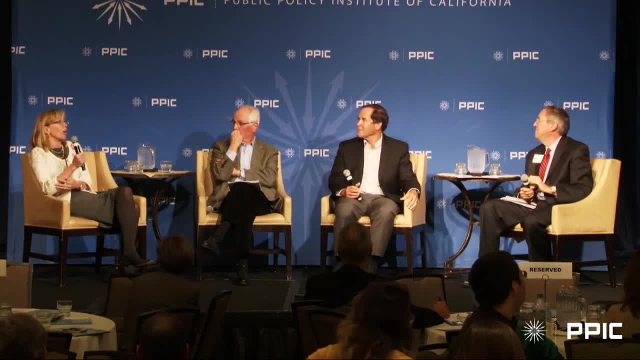 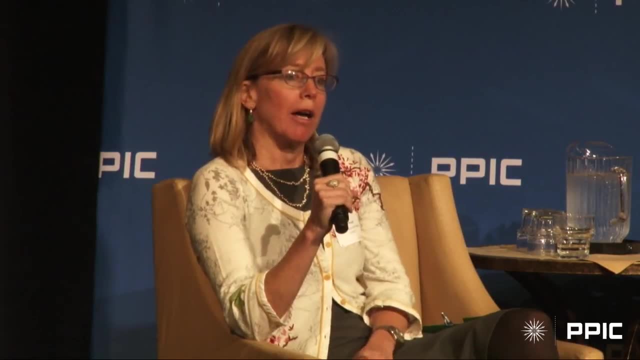 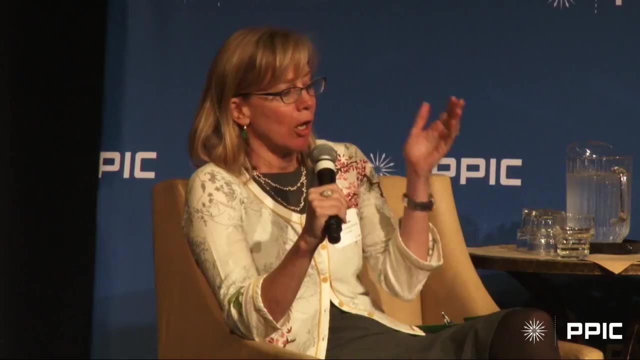 Or do you think we're already doing exactly what we should be doing? Oh yeah, I think there's a big role for the courts, an action-forcing role, much like Governor Brown's conservation mandate was an action-forcing role. I mean when a court or the governor says: 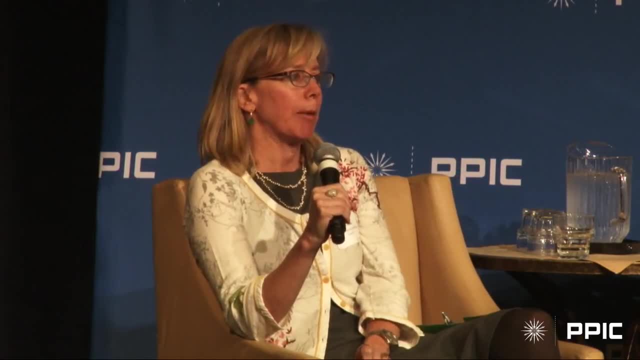 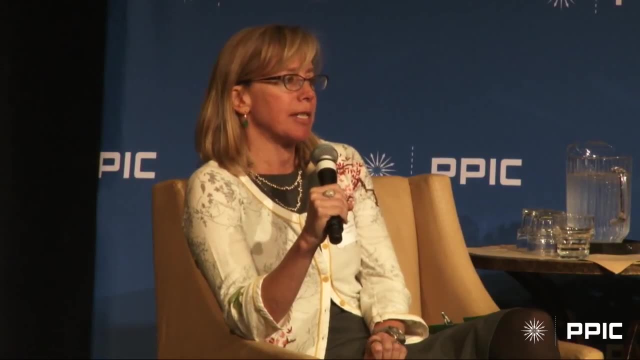 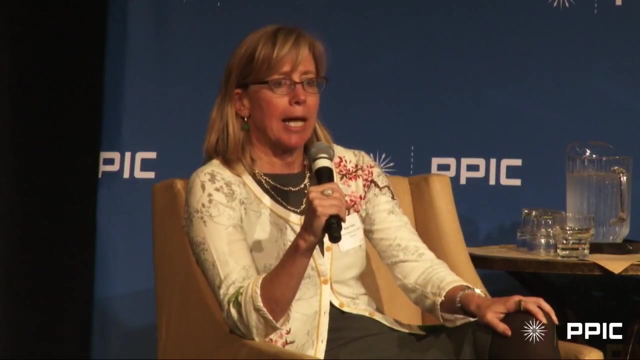 no, you really got to do this. it makes people step up and pay attention And you know- I agree completely with Phil- that we are in a very painful transition period in this state where we're still moving from, you know, just reaching for the Natch River or groundwater basin to tap. 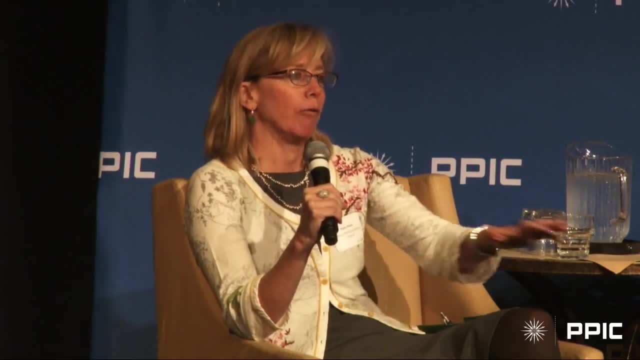 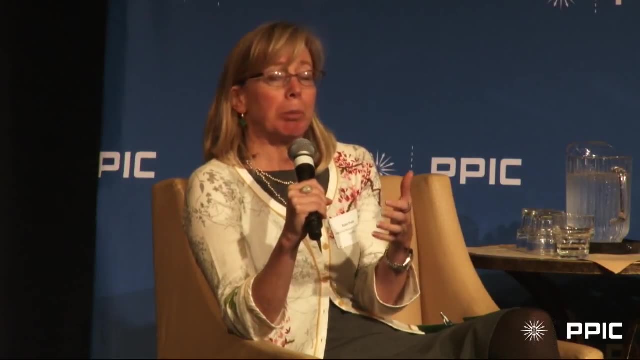 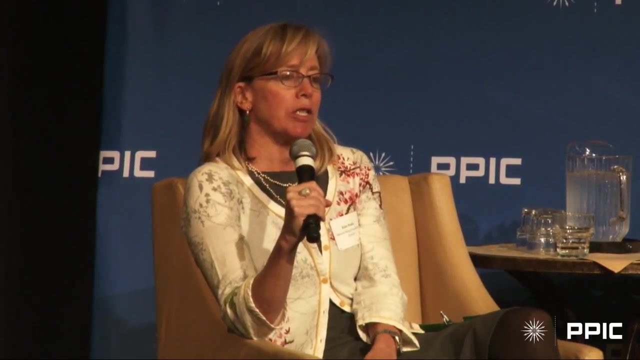 to a realization that we have overtapped those systems and we got to look for different sources of supply in terms of recycling, stormwater, capture, those sort of things, and different sources of management, including efficiency improvements, in order to get into the future. 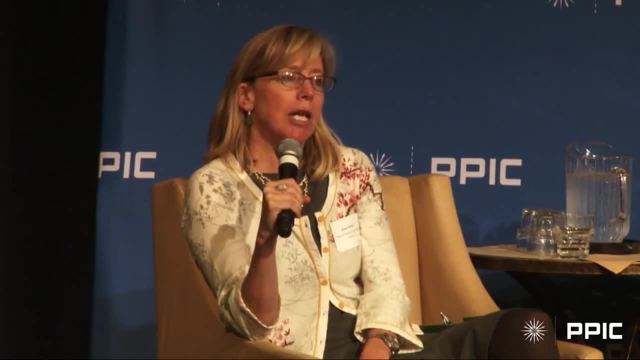 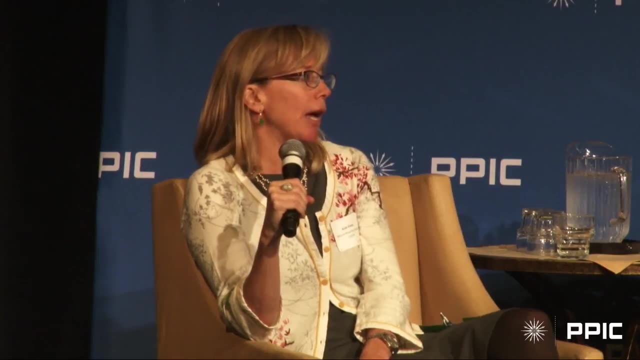 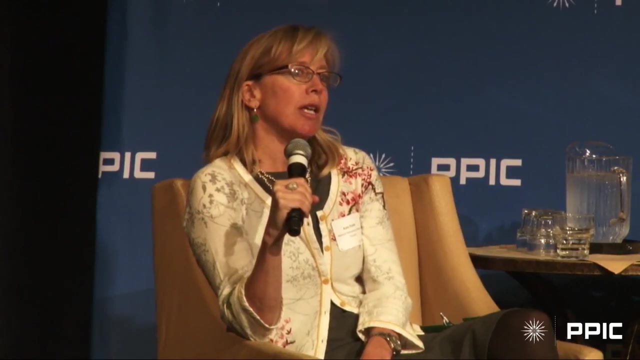 And that's going to be, that's going to be hard, But you know, one of the things we have to do in the near term is stop the bleeding, And we have actually gone to the court to try to prevent many of the waivers. 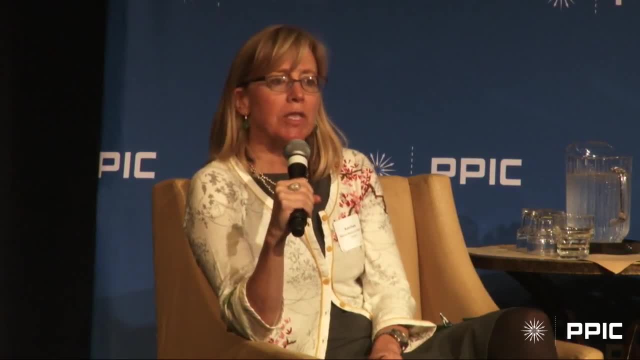 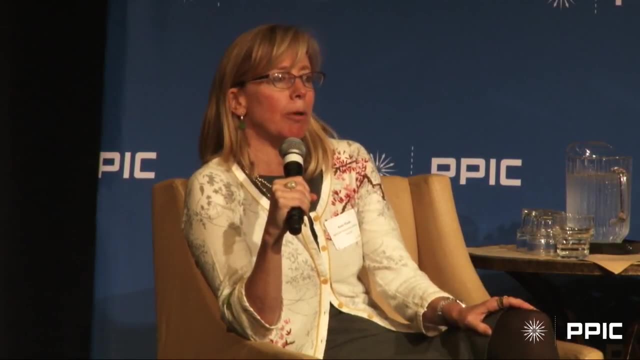 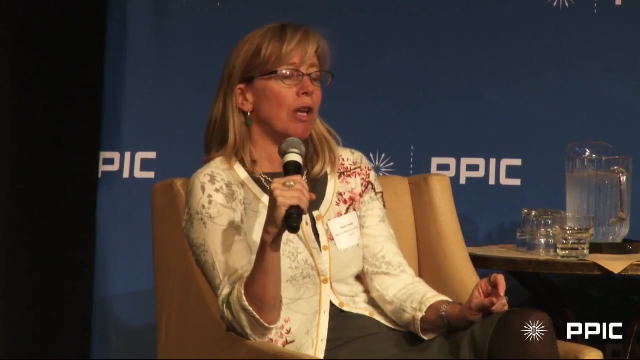 of our sort of minimum baseline environmental standards that we've seen during the drought, to prevent that from occurring again in the future, because that's really made, you know, a bad situation for the environment in terms of the drought far worse by taking at least a million and a half acre feet of water. 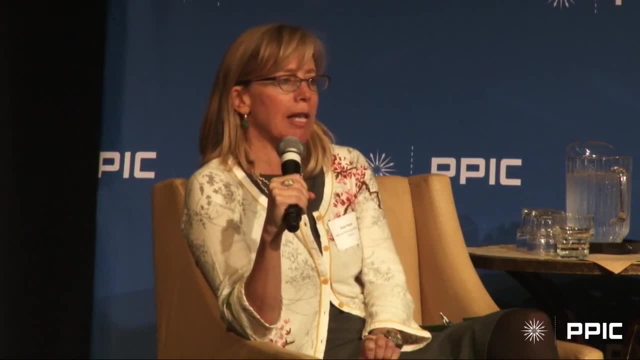 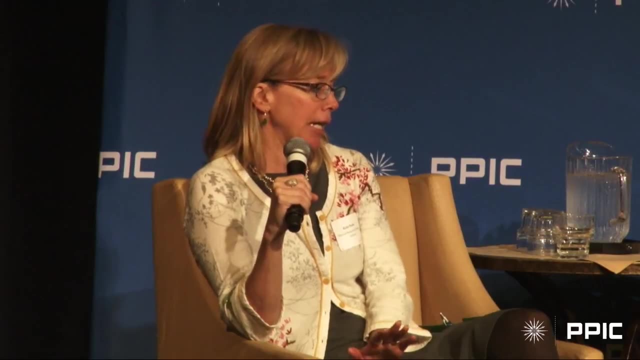 away from those minimum environmental protections over the last three years. So yeah, I think that there's a role for the courts to come in and say, no, you can't do that. You got to actually pay attention to your laws And then you know. 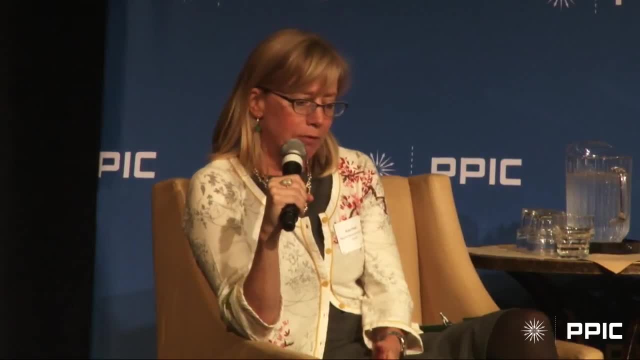 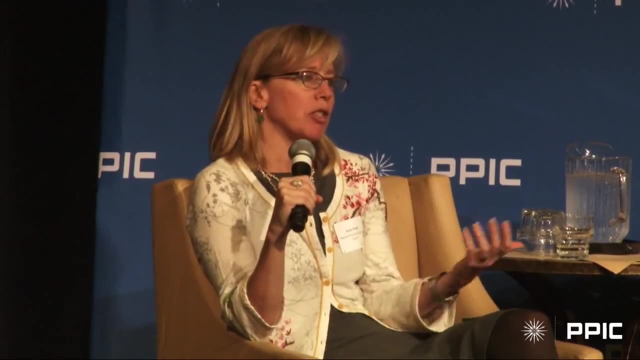 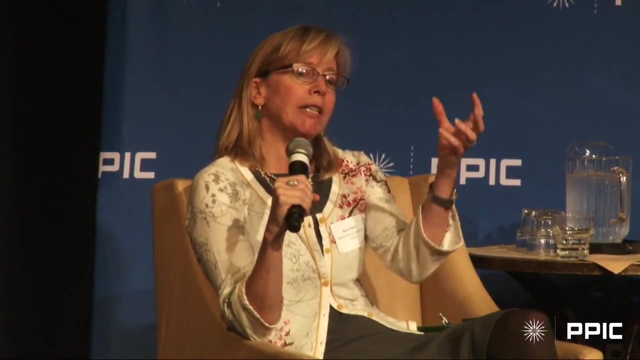 we have to enforce those. We have to get the state board to update its water quality control plan. We have to look at all of the measures we talked about on the previous two panels holistically, So you know how can we bring the Governor's Water Action Plan. 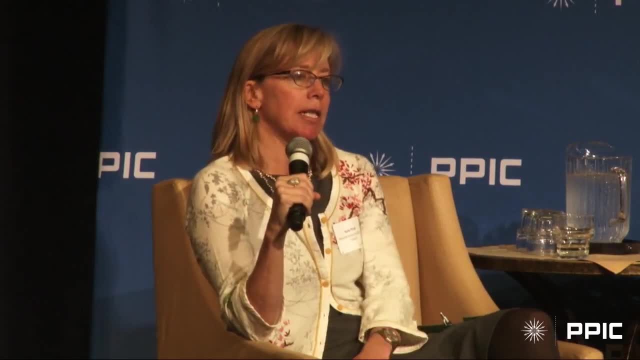 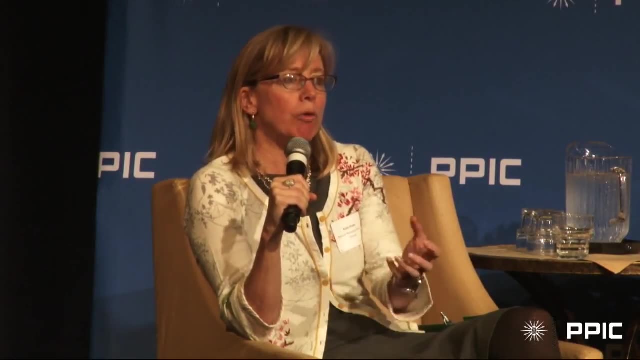 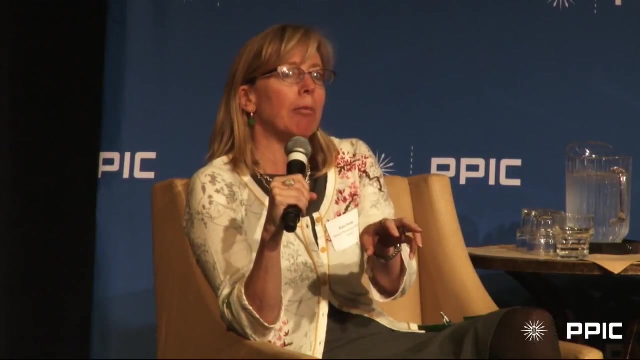 which has a lot of good ideas for achieving a sustainable water future. how do we really add some meat to that and make sure that regions and communities can look at all of their sources of supply and demand management and be able to take less water from overtapped rivers? 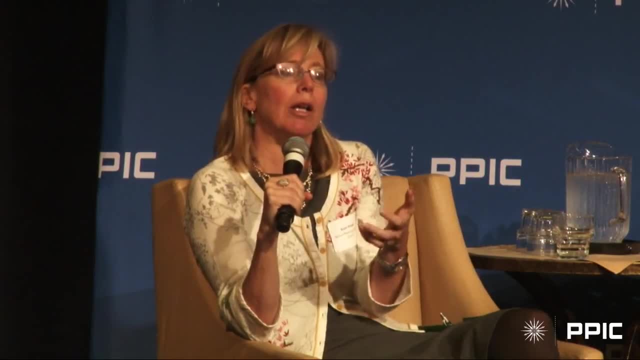 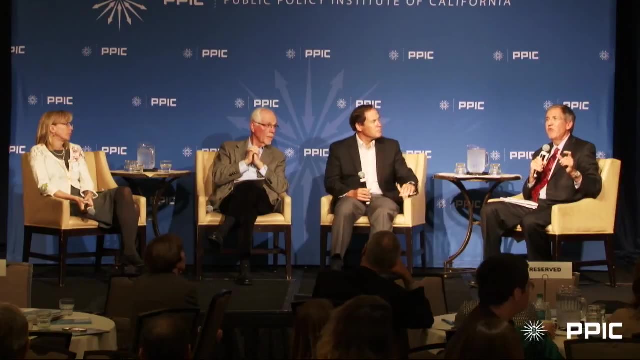 and put more water into the groundwater basins, while creating enough of a supply to get into the future. Okay, in a minute we're going to open things up for questions from the audience, but I want to take the opportunity to ask one last question. 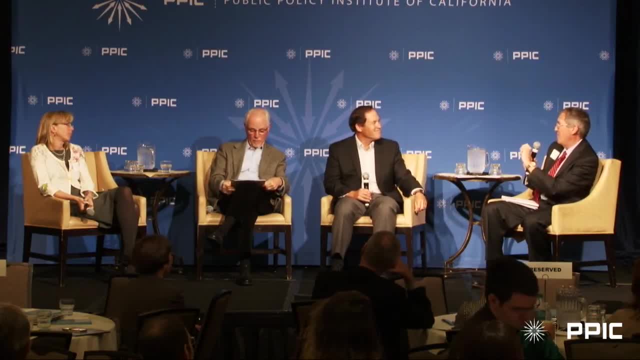 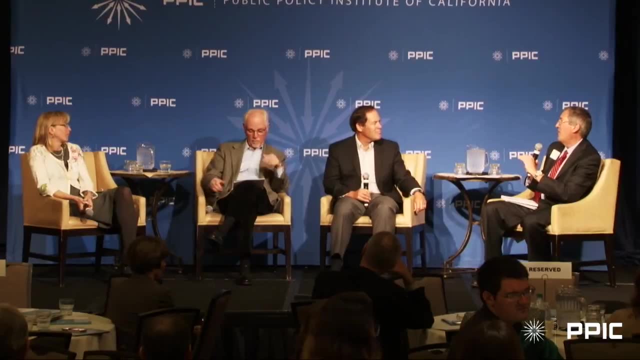 I hope this is enlightening And the answers do need to be short, as Jeff just mentioned, But I want you to imagine that we're now in 2030.. We've come back here for the 15th annual PPIC conference on policy priorities for California's water. 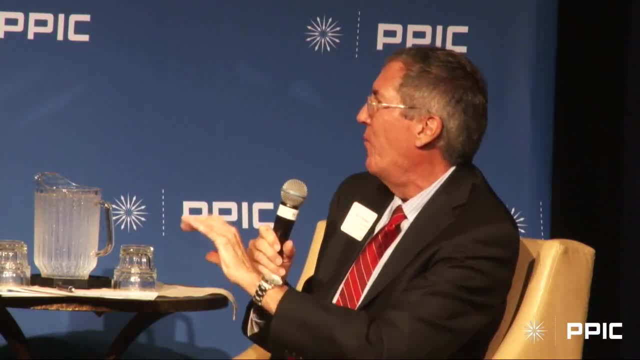 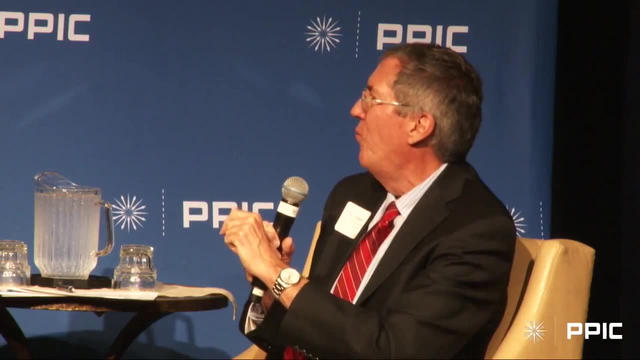 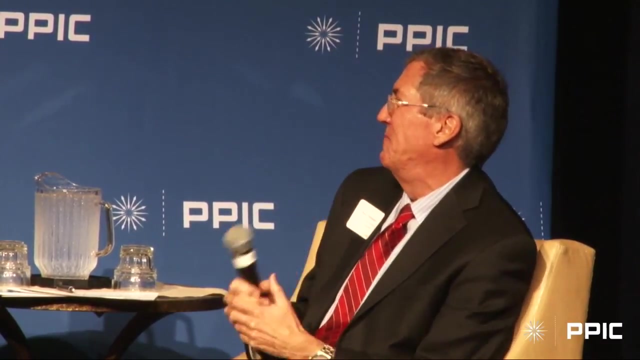 A couple of us get up to the stage with our walkers, but we get up here, And what I'd love to know is your prediction as to what's going to be the state of the aquatic environment in 2030. And how will we have gotten there? 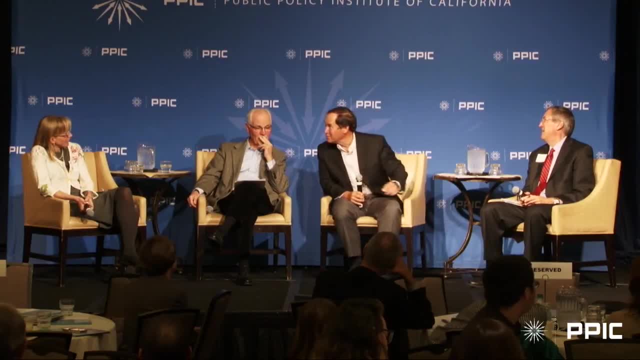 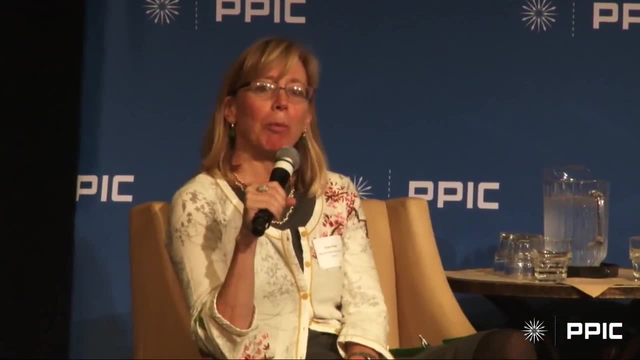 I just started that in, Kate, you first. Well, I'll just keep harping on the State Water Board updating its water quality control plan, because I think that is, you know, sort of the key thing that we need to do in the near term. 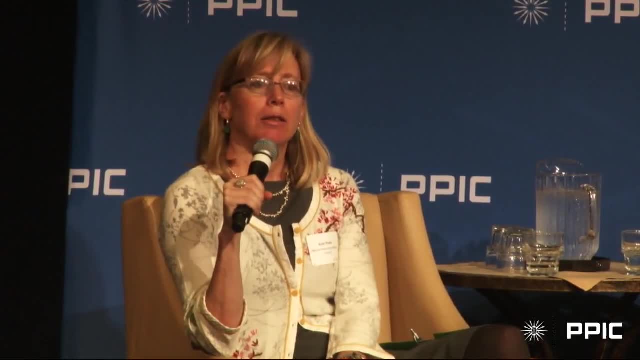 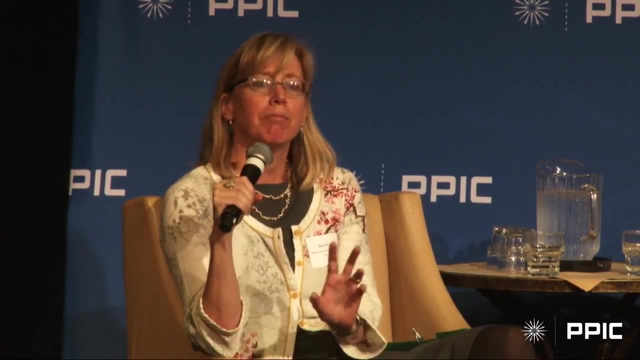 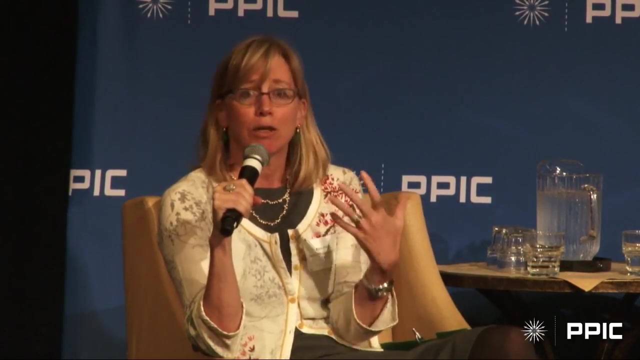 And that addresses not just the decline of species that we're seeing. but, you know, the proliferation of toxic algae blooms um toxic, you know other toxic contaminants and other contaminants in our water quality system provides the flow we need for habitat. 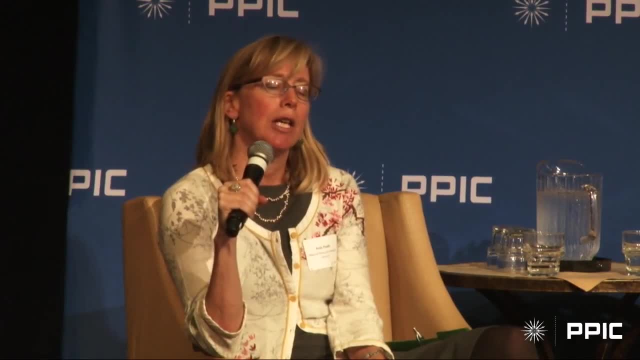 So that's going to be a key piece And if we can do that quickly enough and in combination with some of these investments and other tools which a lot of people are doing- You know we haven't mentioned the mayor of LA. who has announced he wants to reduce their reliance on imported water supply by 50% by 2025, I believe maybe 2030.. So there are a lot of people who are taking these steps And if we can marry those things effectively, 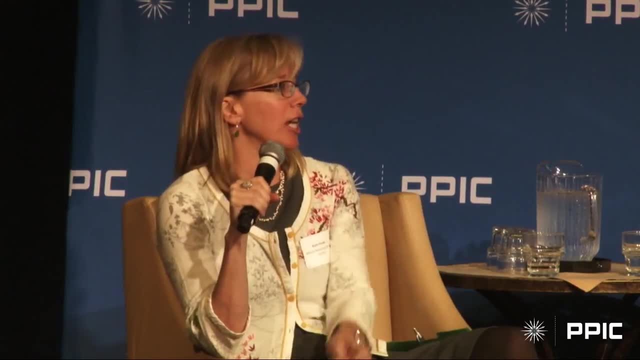 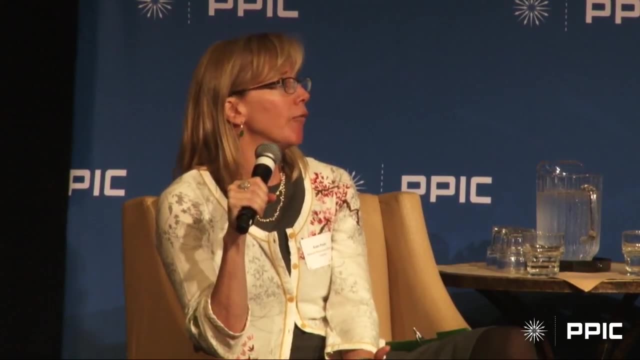 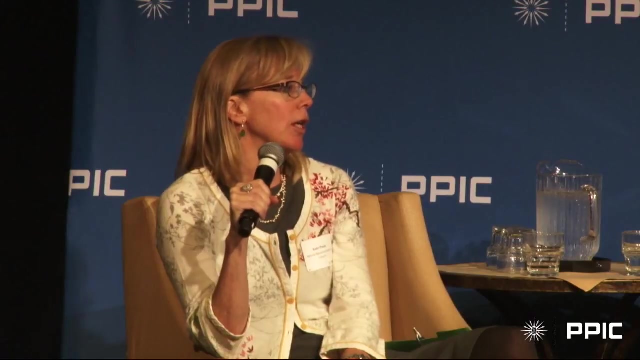 I think we can come back here and see the trajectory for many of the key species that we want to retain and have the healthy river systems that provide a lot of ecosystem functions, on the path towards more functionality than we see today. Okay, Your answer was prefaced by if. 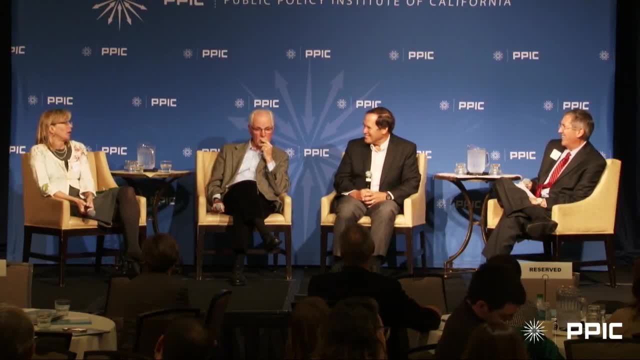 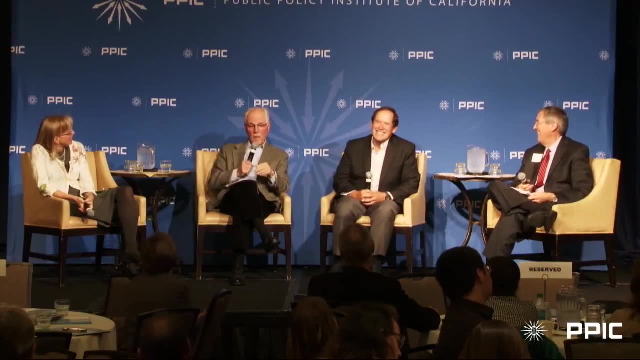 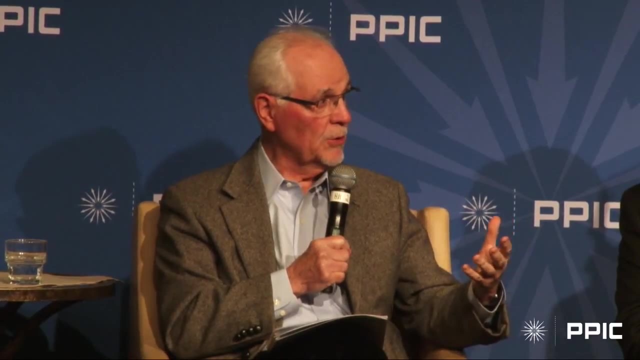 Will we? I can't answer that, but I'm going to be working on making it happen. Okay, Phil, I don't see you can. I can't imagine you can get much positive change in terms of big solutions. I mean, if everybody approved tunnel construction tomorrow. 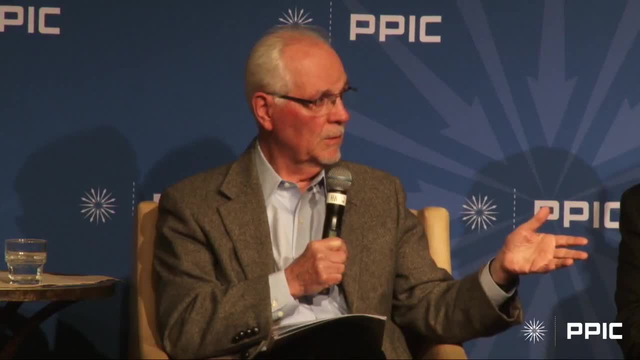 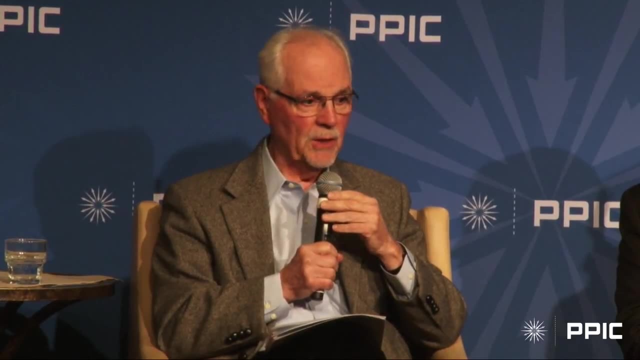 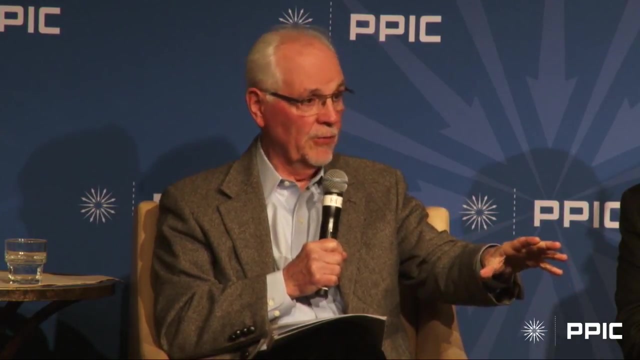 10 years from now. it wouldn't be finished, So you know. so it's not as, if that's possible. It might see some accelerated pace of the agency's compliance with the 2008 biological opinion- for God's sakes, which hasn't yet started. 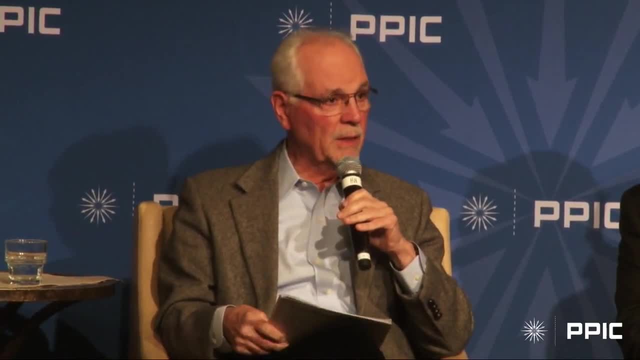 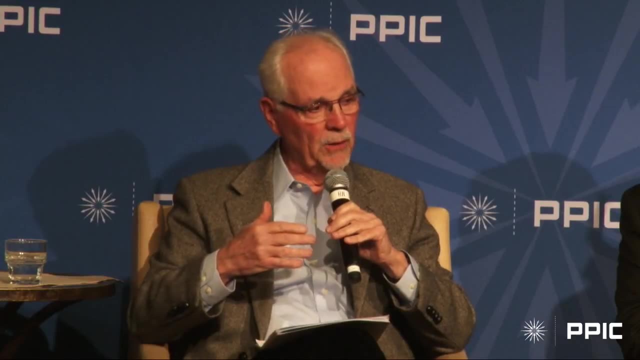 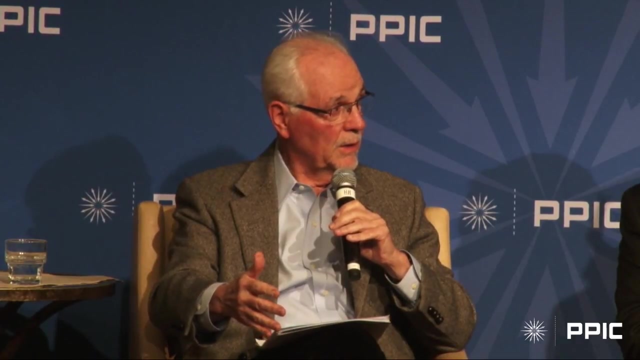 but is supposed to be underway. But you know there's kind of an example of how rapid the pace is complying with federal orders, I don't. You know you could see some further deterioration of the fish species in the Delta likely. 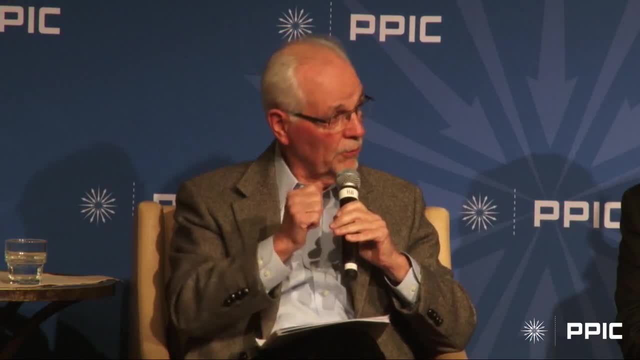 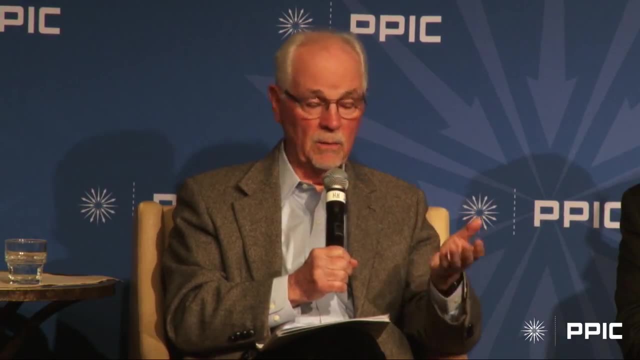 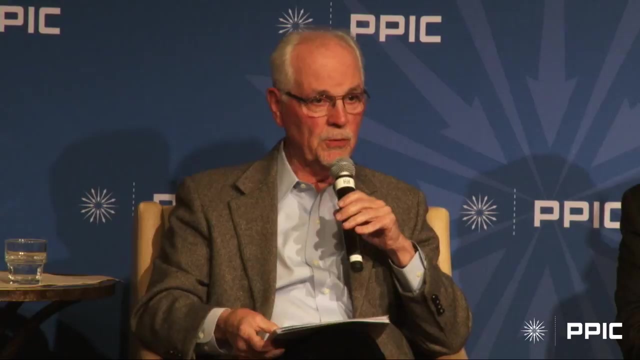 but how much more dramatic, I don't know. The real kicker is: if the dry years continue, hope to God that the Water Board reimposes their mandatory water requirement. I mean, I heard all the discussion about local agencies who are doing the right thing. 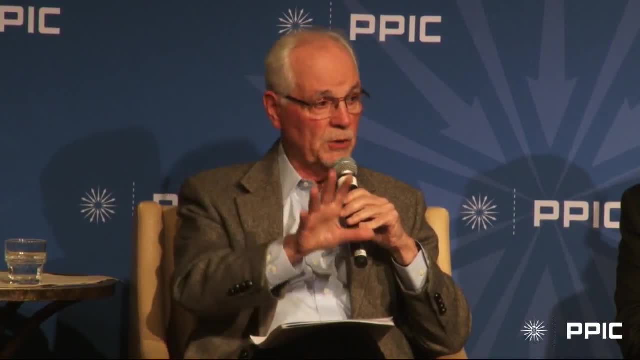 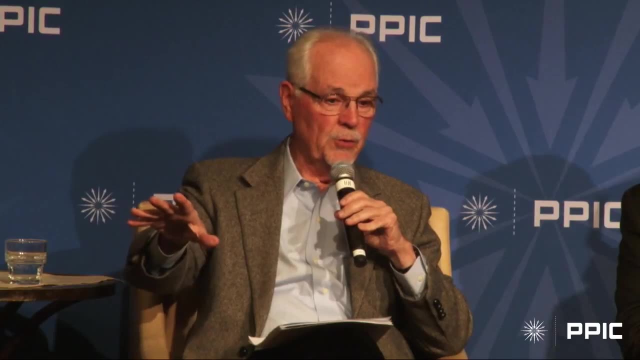 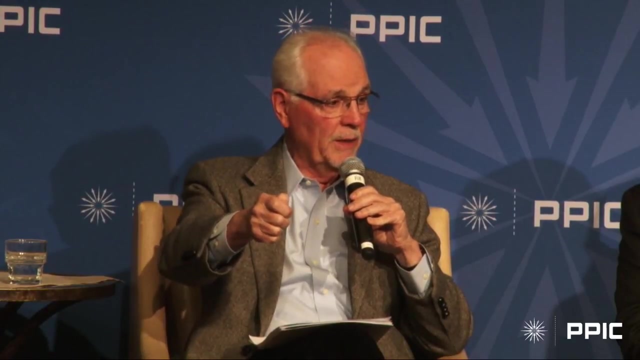 but the reality is you can't solve statewide problems or problems scattered around California by giving 1,000 jurisdictions kind of free rein to do whatever they want. Adding up the individual actions of all the people of California does not constitute a water plan. It constitutes a status quo. 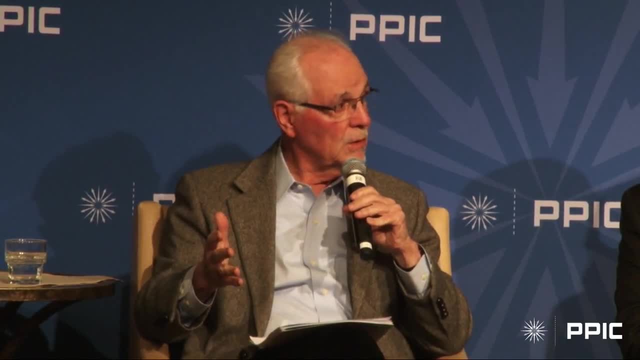 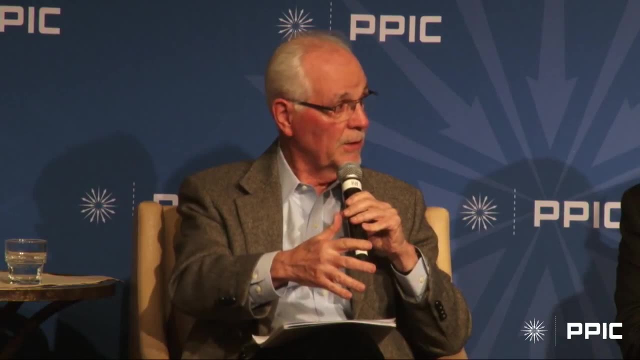 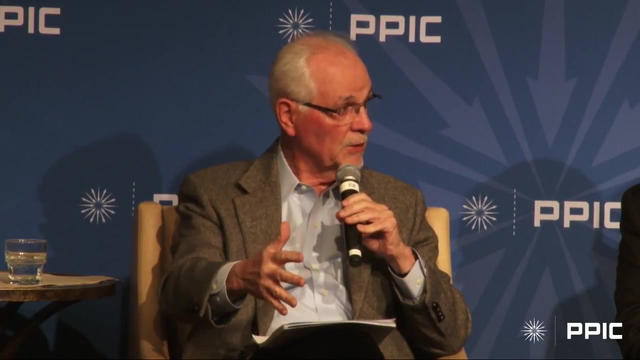 So you know, I think you don't see much change in 10 years, 20 years, 30 years. Now there can always be a cataclysmic event. What an earthquake, What an earthquake would do. What a massive spill of toxic chemicals. 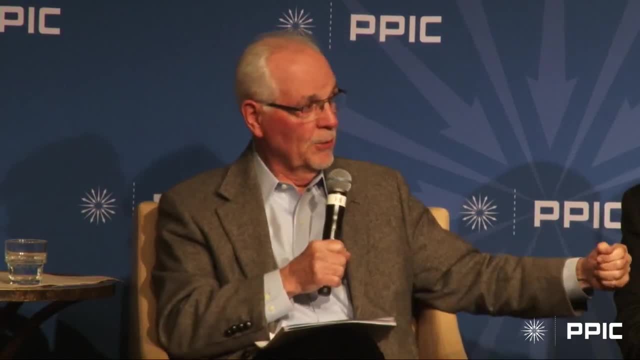 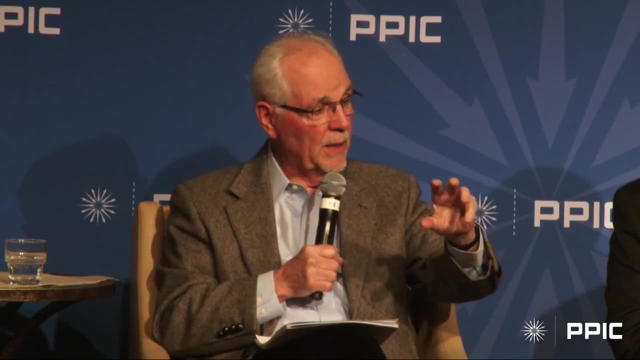 might do in the wrong location. That's where Dr Doom comes in and he can explain all that to us. That could lead to change, But I think the biggest possible driver is the fact the public's advanced beyond. The urban public has advanced beyond. 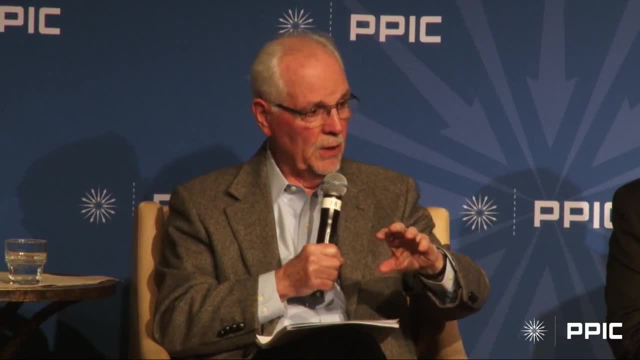 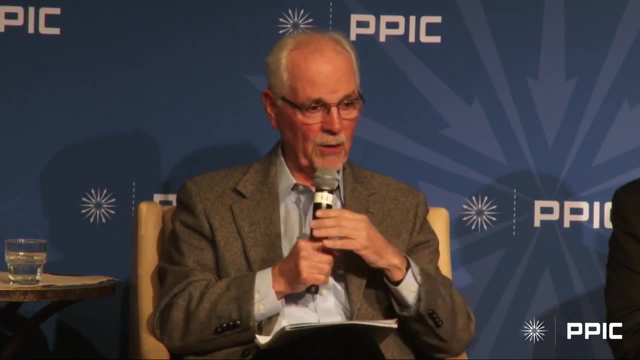 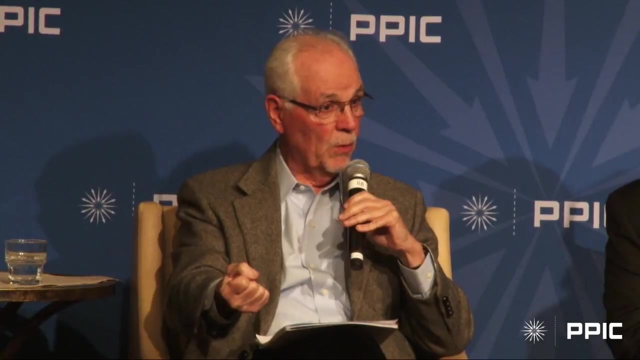 all us policymakers and water managers, because they were. They learned a lesson. They learned a lesson, Gosh. we actually reduced our water use and we saved a reasonable amount of water, and the world didn't come to an end. The absence of a continuing conservation requirement. 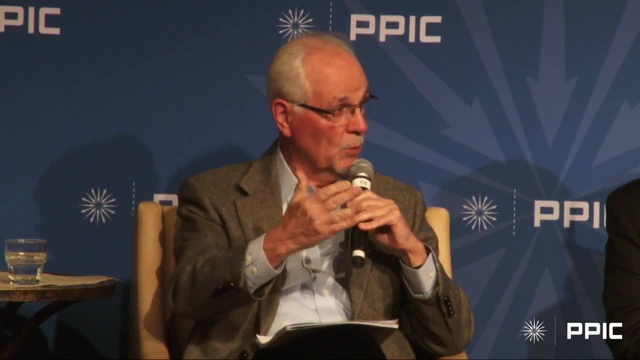 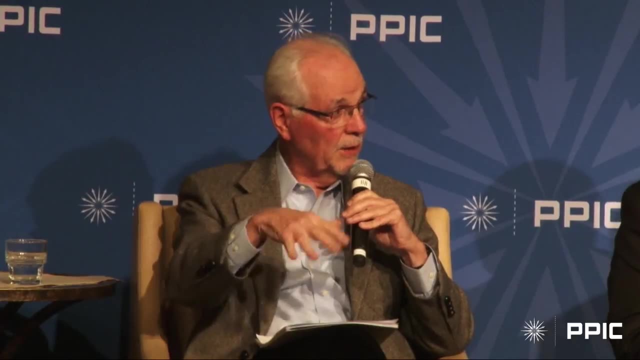 jeopardizes that opinion because it means more and more real people say, well, it wasn't a real emergency anyway. That's the only chance I see of getting near-term action. Okay, And Jeff, quickly, Let there be a ray of hope. 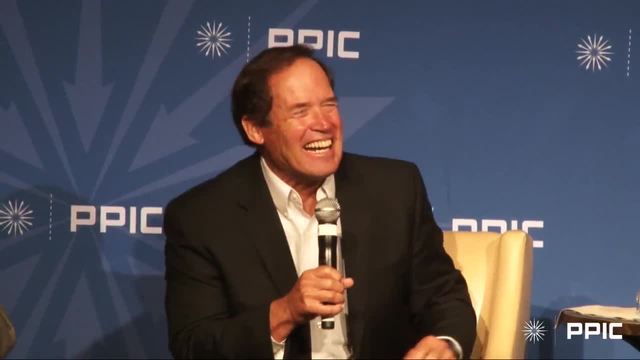 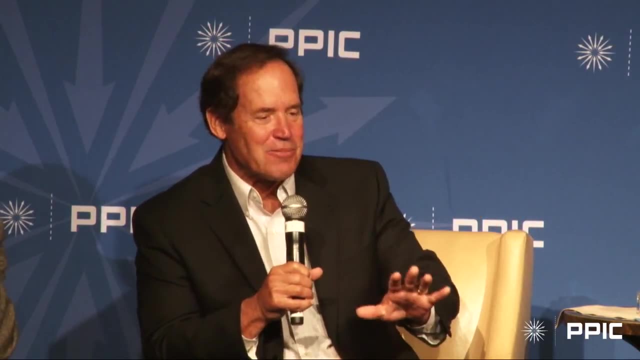 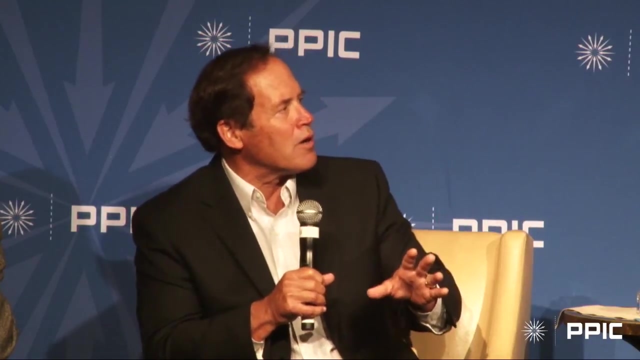 I hope I'm here So, dude, when I daughter up here. I have a very different view of this, which will not surprise anybody. The Sustainable Groundwater Management Act will be considered the most seminal water act, the most profound water act in our lifetimes. 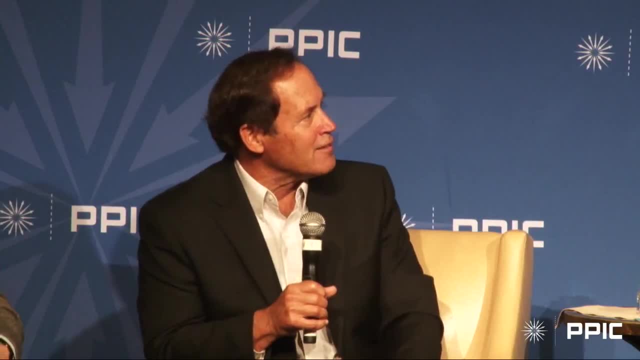 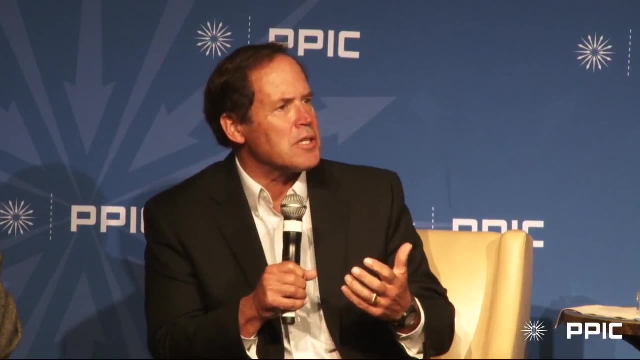 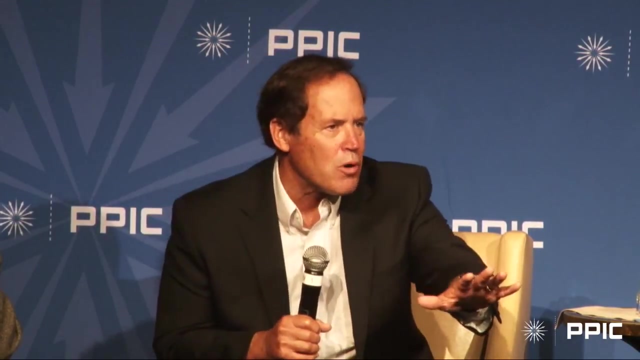 And here's what it did, what it will have done when we come back. It will have triggered the fact, triggered us to have a good and productive conversation about reliability And why reliability is so important, even if you're now relying on much less water in Kern. 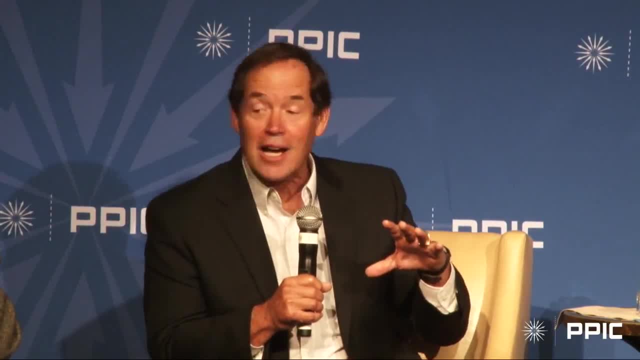 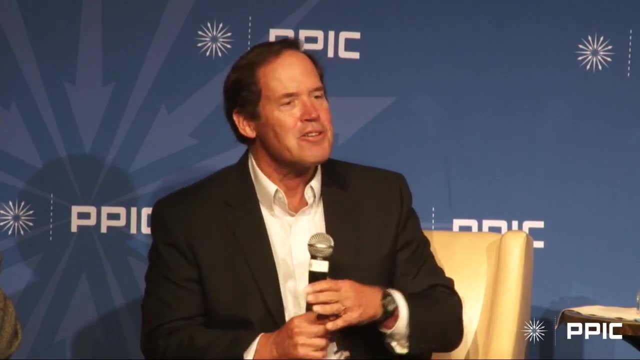 The gold standard for them will be reliability. At the same time, the environmental interests and the state board will come in and say: look, let's negotiate a solution on this. So here's our solution. Our solution looks like: yeah, you're going to get less water out of the delta. 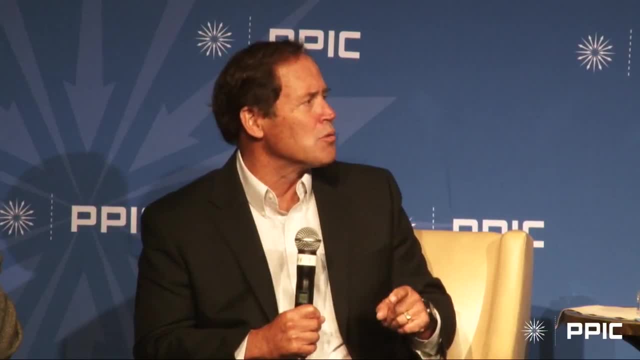 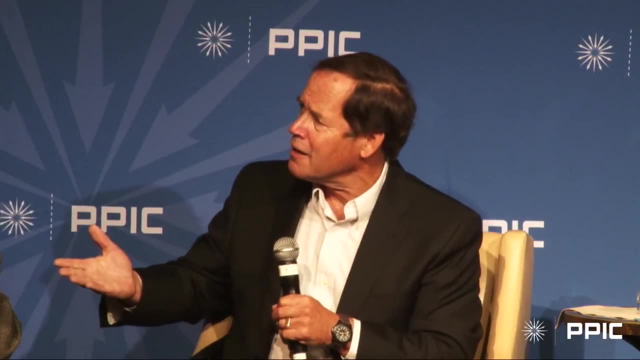 but it's going to be much more reliable. That will help you deal with the Sustainable Groundwater Management Act and its implementation without blowing it up. We'll still have more reliability, And the way we're going to do that is we're going to allocate the environment. 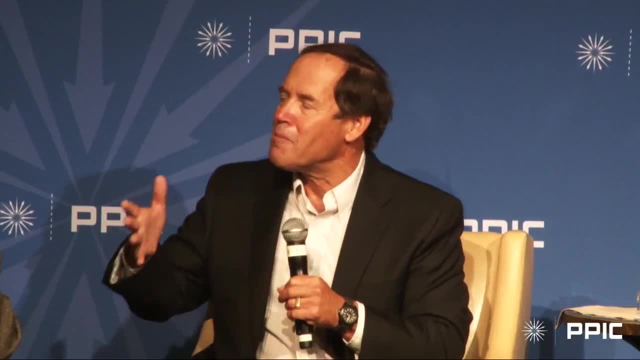 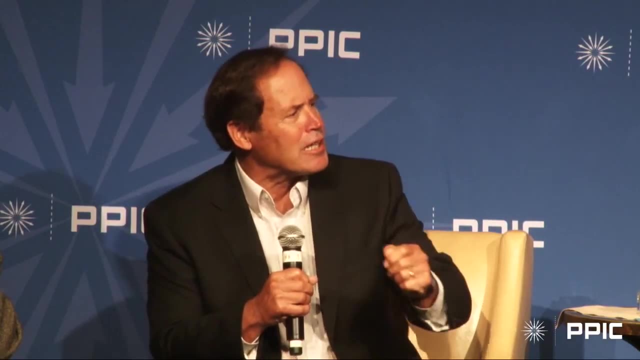 a certain amount of water, And that's what the environmental managers have to live with, that they're assuming some of the risk And rather than just I need a little more, I need a little more. No, this is what you got. 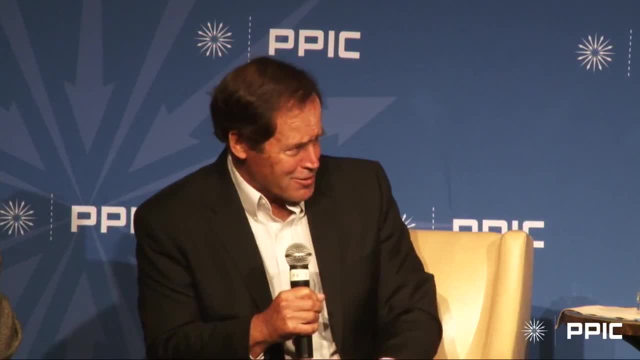 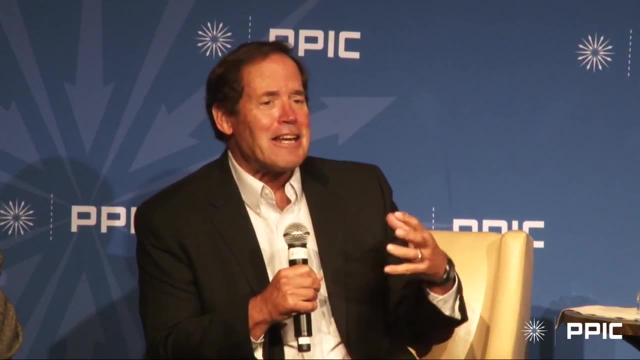 Work with this for 10 years, because we need that sustainability south of the delta. That's where I see the big breakthrough coming, driven by the Sustainable Groundwater Management Act, And at the centerpiece for all of this will be our changing State Water Resources Control Board. 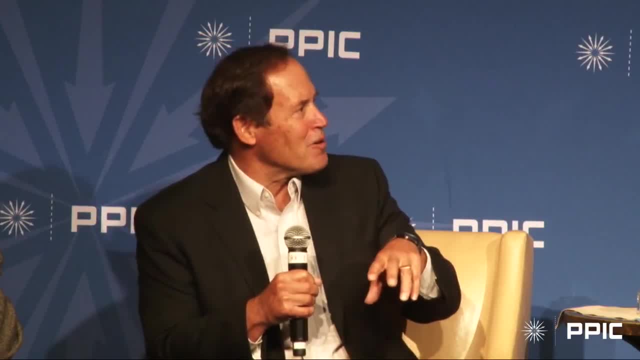 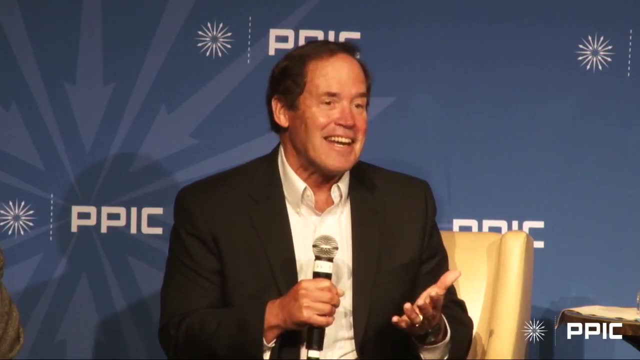 Remember when, in our youth, the State Water Resources Control Board used to have people go out and negotiate stuff and they accepted it. And now they're a very different board And now they're actually trying to push us to solutions rather than accepting solutions. 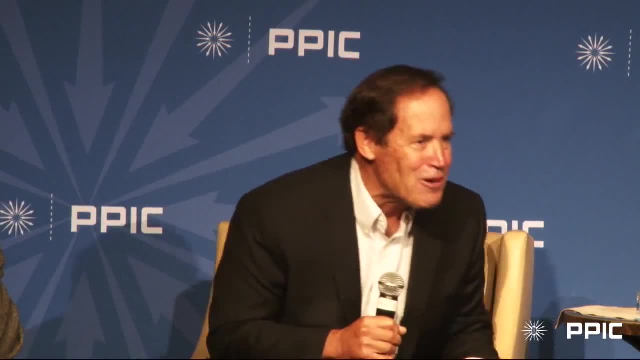 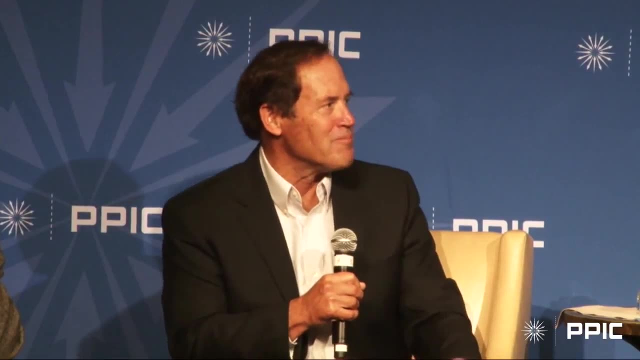 So on that day when I daughter up here in my, what we will be talking about is how the Sustainable Groundwater Management Act transformed environmental management in California. So there, that's optimism. Okay, thank you. So now we're going to open things up. 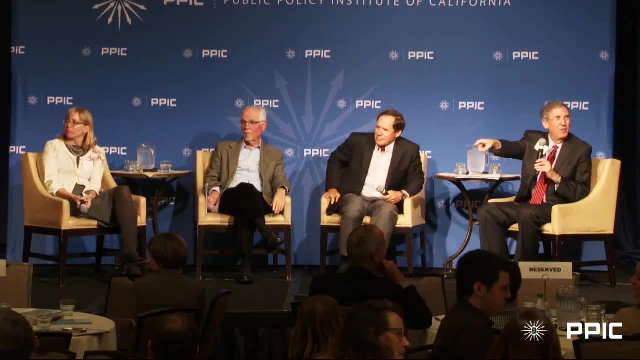 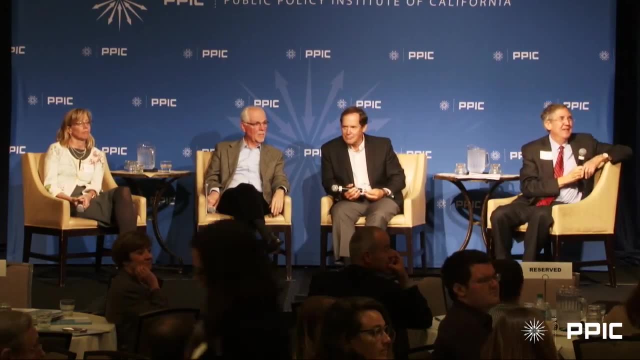 for questions and answers And we're going to start back here And then after there, then we're going to come over here. Hi Warner Chabot at the San Francisco Estuary Institute. It's a delta question for all three of you. 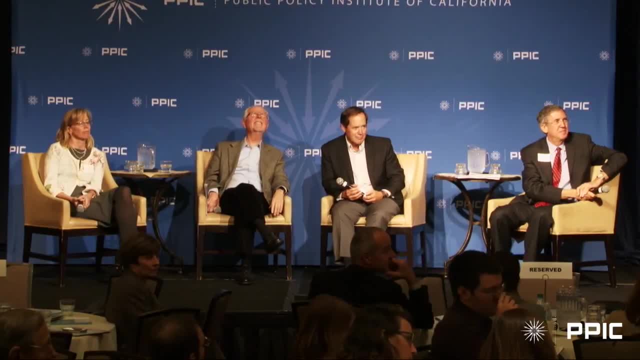 Because of the wisdom that you've demonstrated today on the panel. you've now been appointed either emperor or empress, respectively, of the delta, But you're only empowered to perform one single action that will shift us towards large-scale ecosystem management. What's the one action that you would take? 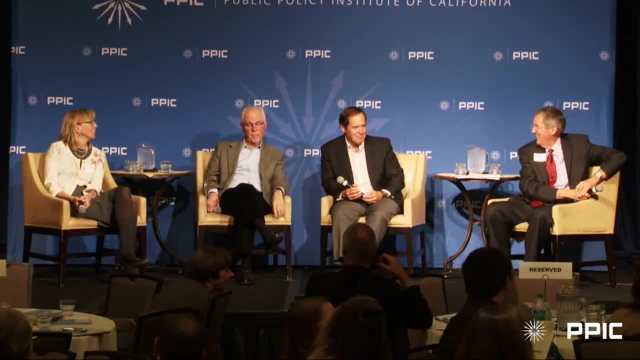 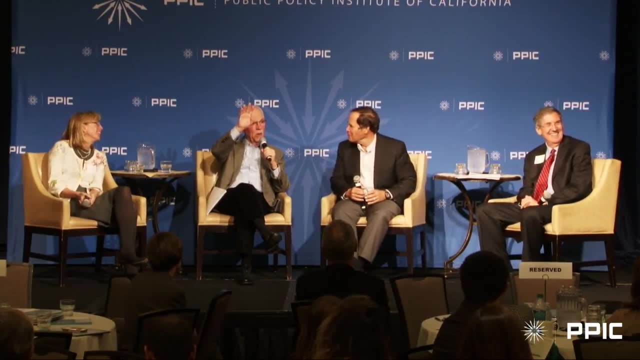 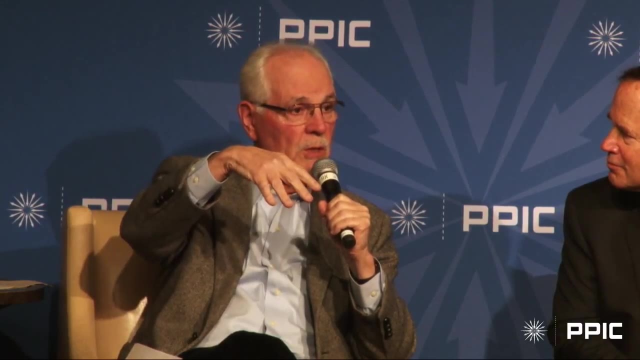 I think this is Phil's. I'd do it. I'd take all the state and all the federal employees from the coordinated operations agreement that's been in existence for some time. I'd shove them in one building. I'd tell them to read the California law. 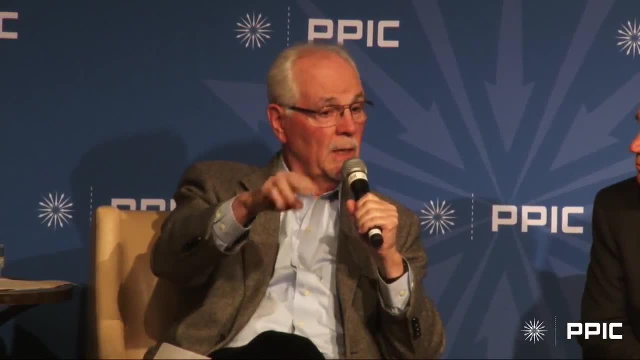 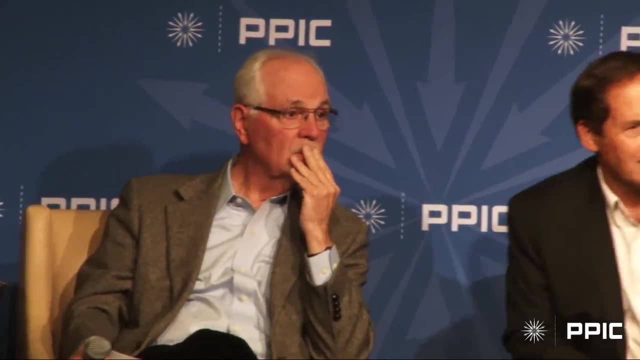 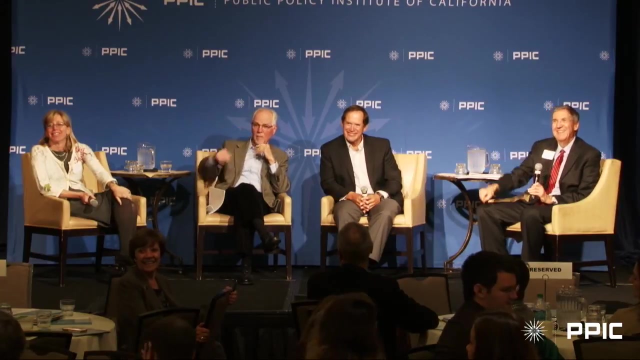 on co-equal goals and reduced reliance on the delta and say, guys, don't screw it up, That's what I'd do. I'm with Phil. Okay, there's a question back here. Jacob Katz, California Trout. It seems to me that there's a very key fact. 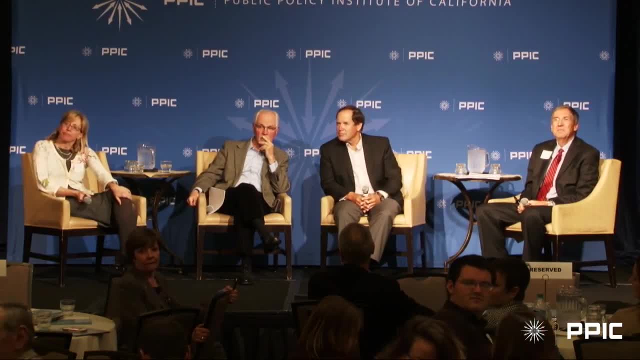 that's missing in this discussion, and that's that extinction is driven by a very simple phenomena: When native species can no longer recognize the systems, in this case the aquatic ecosystem, and they can't recognize them. they can't recognize the ecosystem. 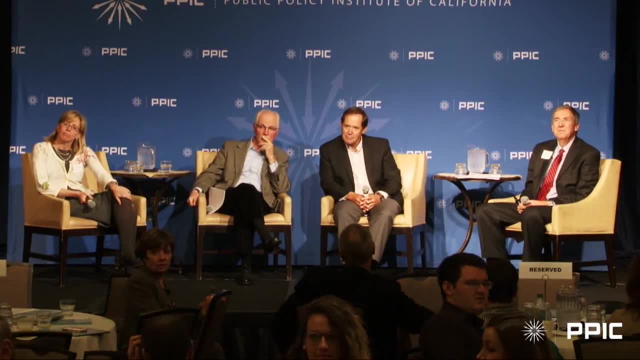 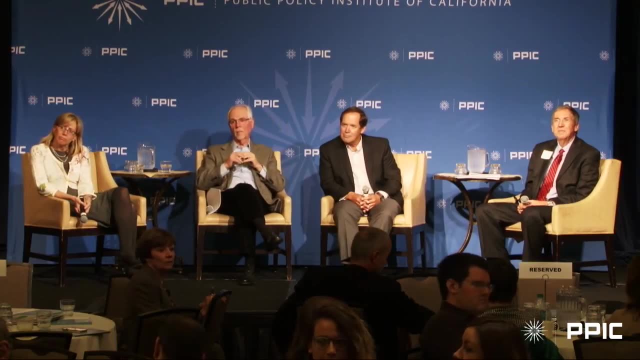 that they evolved in, to which they're adapted to, you get replacement. You get species that evolved here replaced by ones that recognize a stable system. You get, instead of salmon, you get bass and catfish. That's what we have right now. 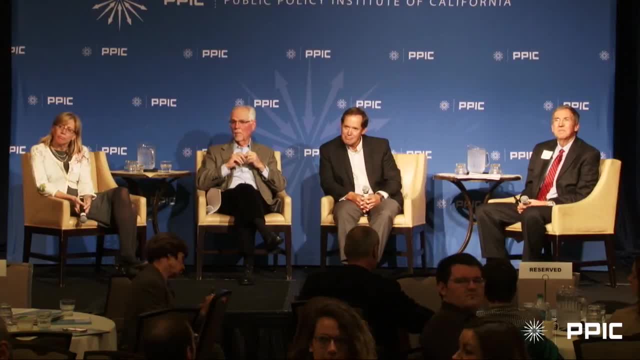 and it's a direct result of water infrastructure laid down 100, even 150 years ago. We hear a lot of talk, decades of talk and hundreds of millions of dollars spent, but very little has been done to actually change the way that water flows across California's landscape. 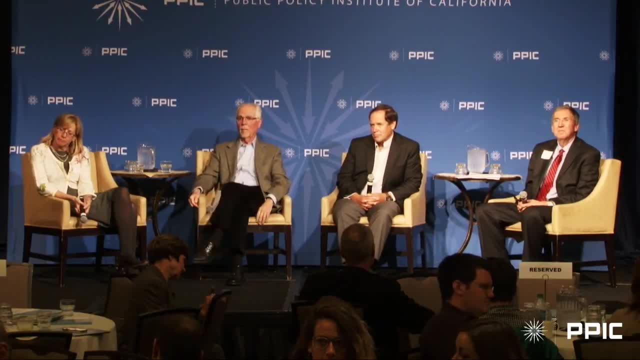 How are we gonna do that? How are we gonna transition- and I recognize this is the public policy Institute of California, but this is about implementation- How do we change the footprint of California's water infrastructure, Jeff or Kate? Well, I'm happy. 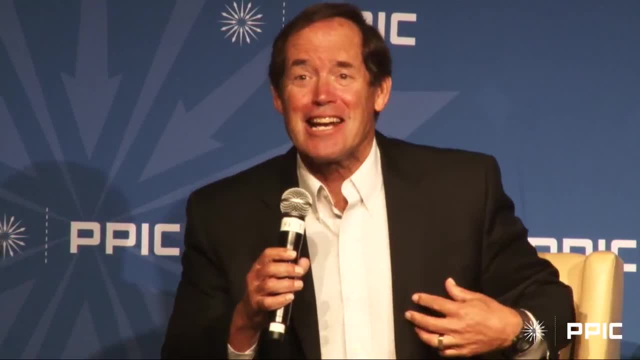 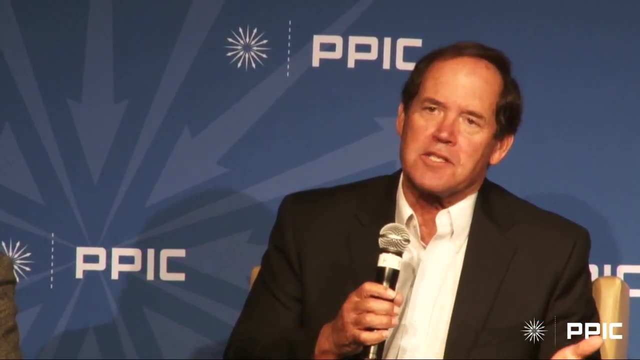 since you are my former student and I am channeling your major advisor, It seems appropriate, Jacob. this goes right back to taking an ecosystem-based approach, and that is what are the ecosystem functions we want to manage for and restore in this system. 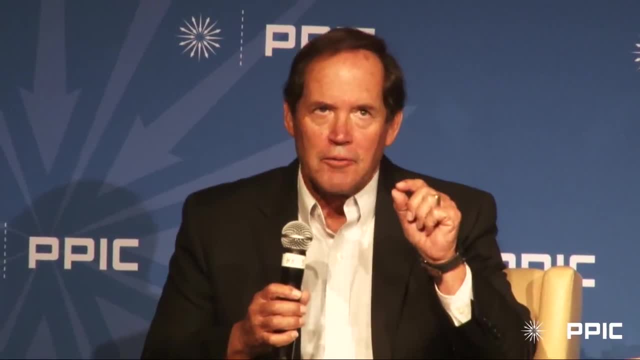 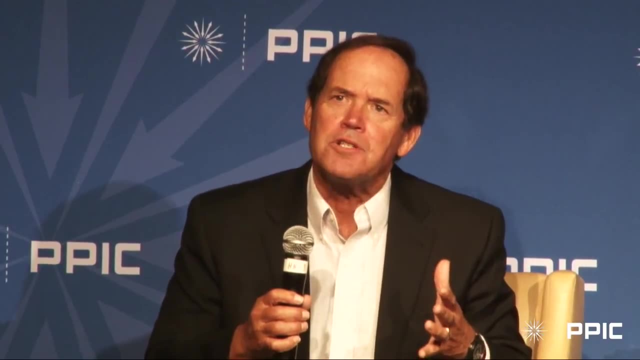 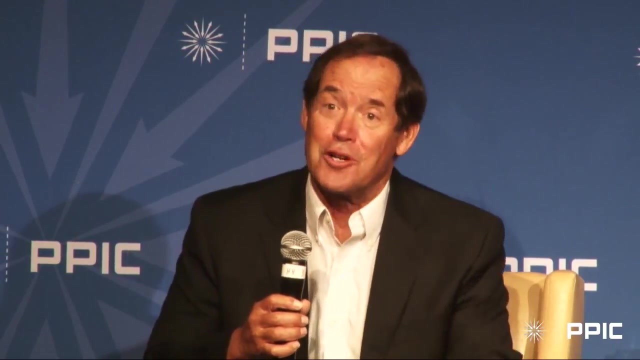 rather than saying I want to focus all my effort on delta smelt, No, I want you to focus on re at least establishing the functions of an estuary. Or I want to save the. well, let's take the winter run Chinook salmon. 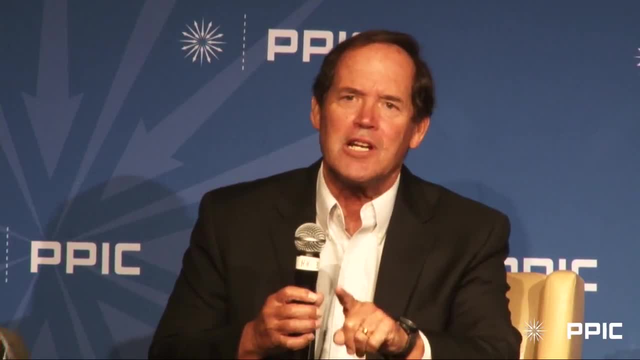 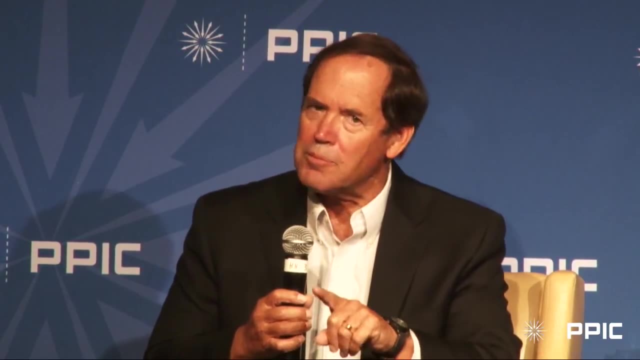 as a good example. No, no, no. I don't want you to focus on the winter run Chinook salmon. I want you to focus on reestablishing the functions in this system that support anadromy. okay, And that's a little bit of. 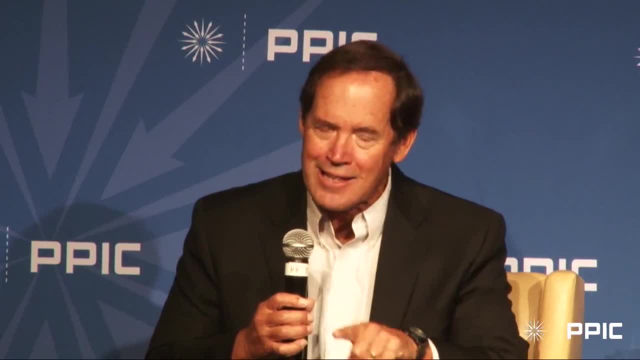 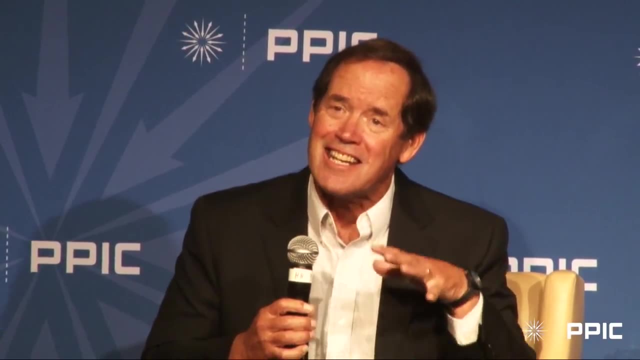 let the chips fall where they may approach, But I think, with a very rapidly changing climate and major fiscal constraints, that that's why I say: you take an ecosystem-based approach to this, And I know you're in the thick of this out on the Yolo bypass. 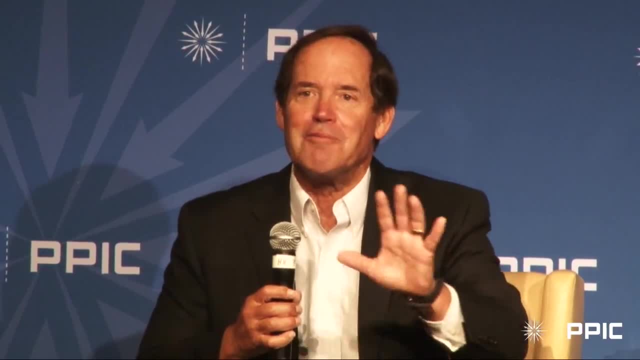 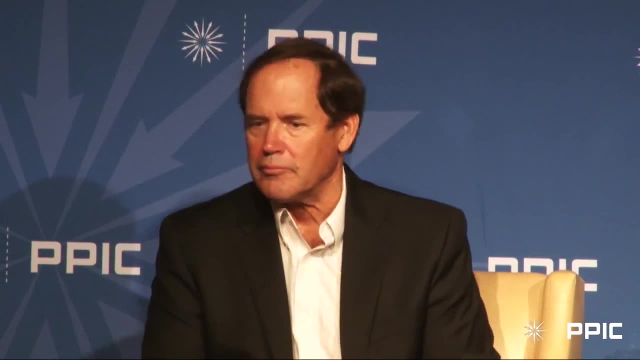 which is glorious, taking forever to get this stuff done, but is a terrific example of focusing on function rather than a specific species. And Kate, Yeah, I totally agree with that. I think we- I mean we- have a pretty amazing base infrastructure. 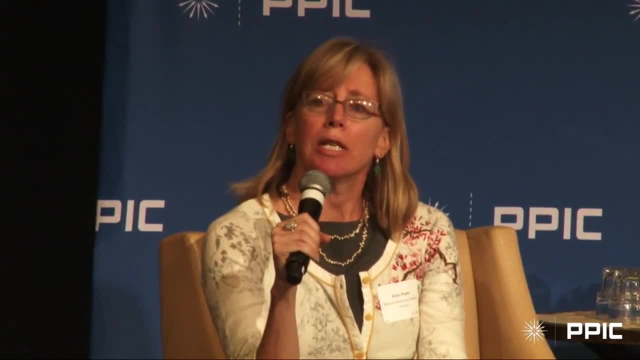 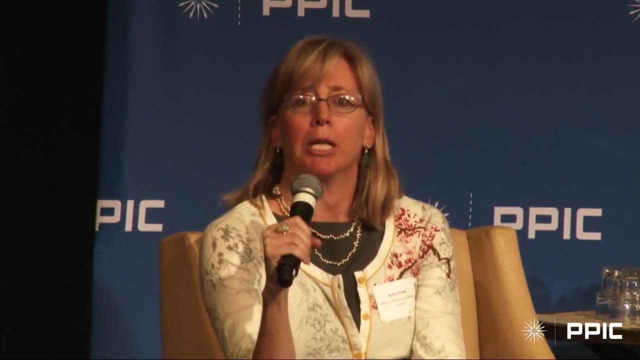 in this state and I think we can use it much more to our advantage. And Yolo's a great example. If we actually operated the Yolo Basin floodplain to you know, increase salmon productivity, it could be a huge resource. 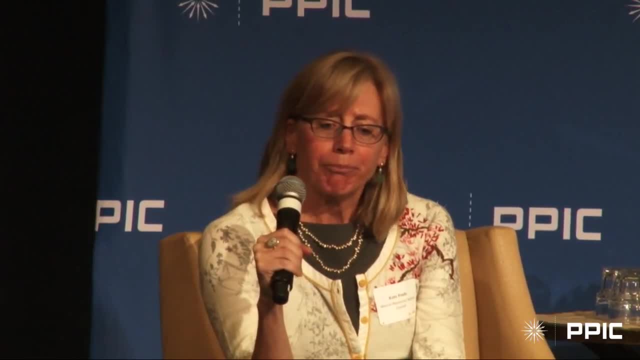 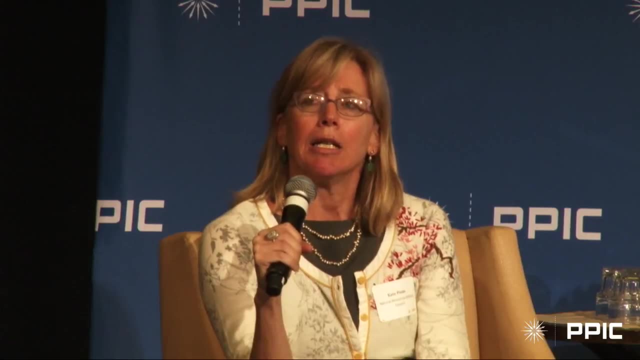 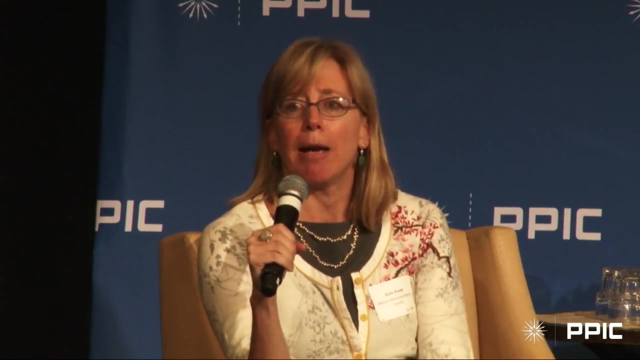 But we haven't operated it that way very well And I think you know in terms of how intertied we are throughout the state. we can start thinking about moving water around in different ways than we have in the past and perhaps get more recycled water. 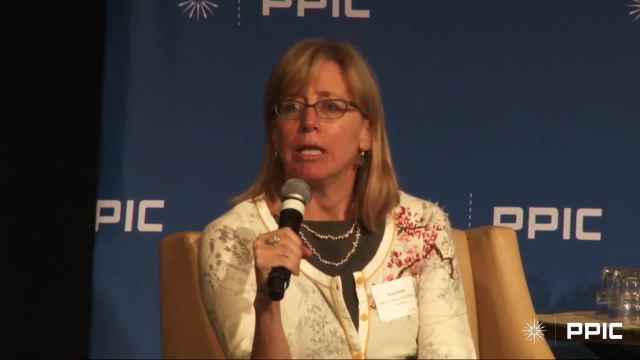 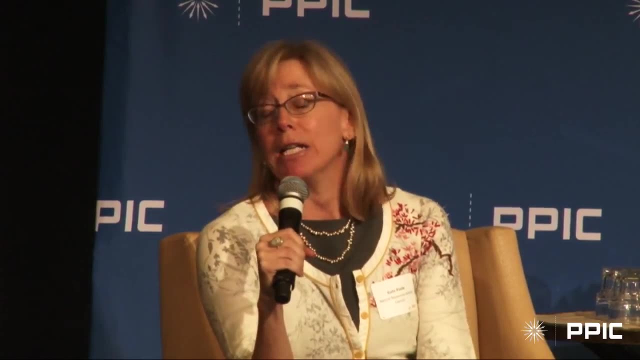 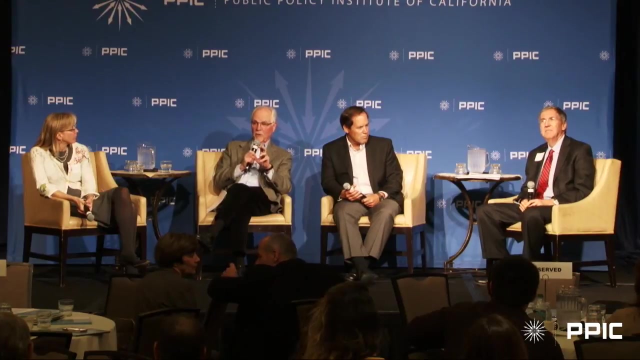 from urban areas into ag areas to help, you know, ease the transition from less groundwater pumping and less surface water pumping. So we need to operate it differently is the bottom line. I may have read into your question something that you did not intend. 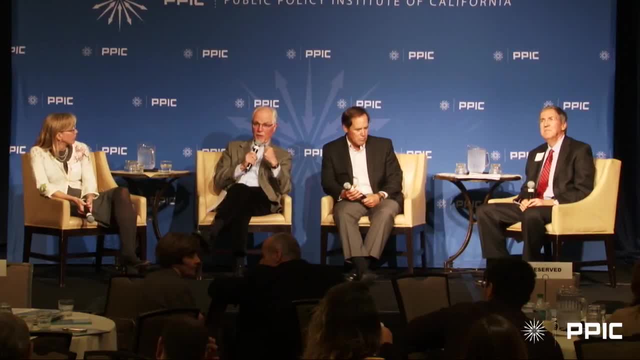 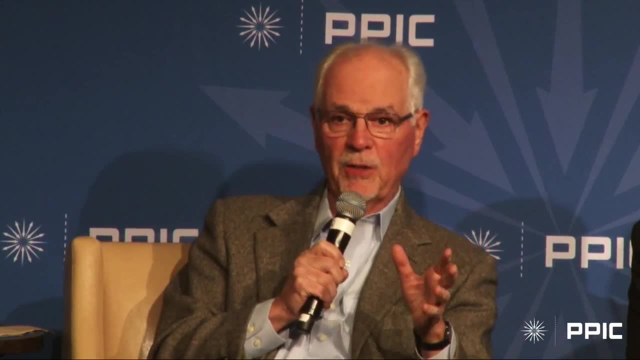 but I've just finished reading the latest book by John Wiens. Dr Wiens, who's on the Delta Independent Science Board, a landscape ecologist, smart guy- and he writes in English, so I can almost understand what you guys say. 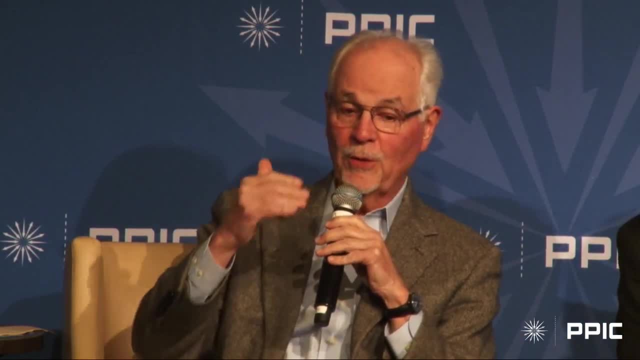 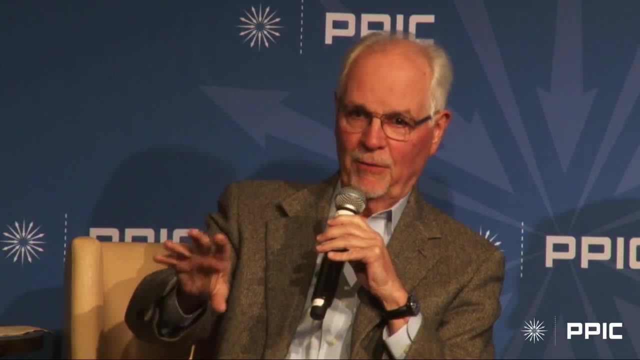 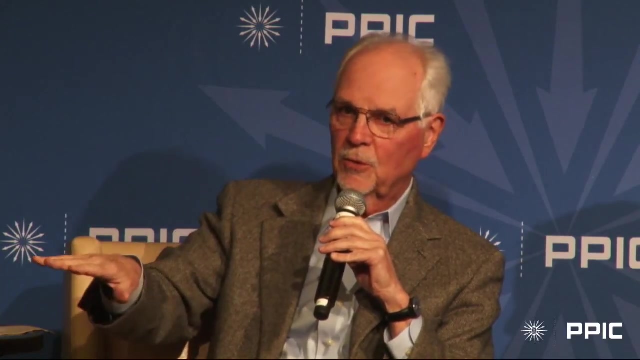 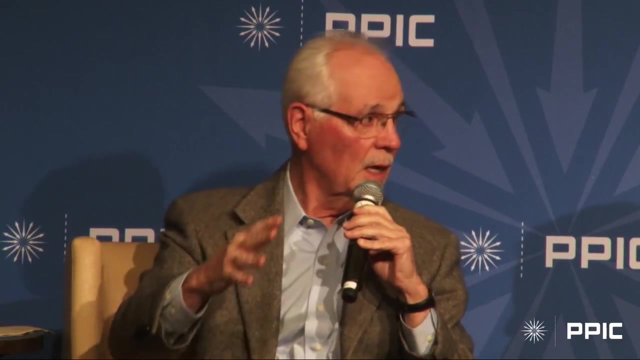 But his reminder- his reminder forcefully- was efforts historically to restore what used to be called the balance of nature. the natural condition to which everyone must aspire has been surpassed by science. It's the periodic disruptions and the constant change and almost turmoil that goes on in the natural environment. 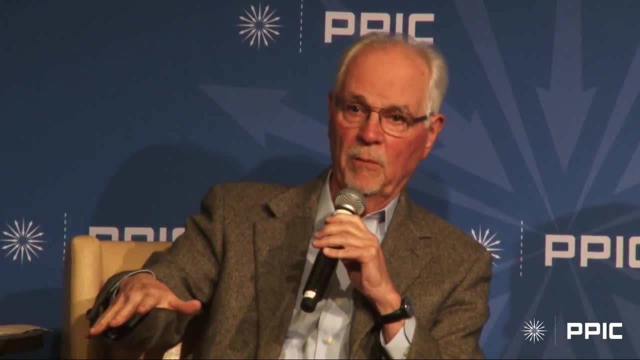 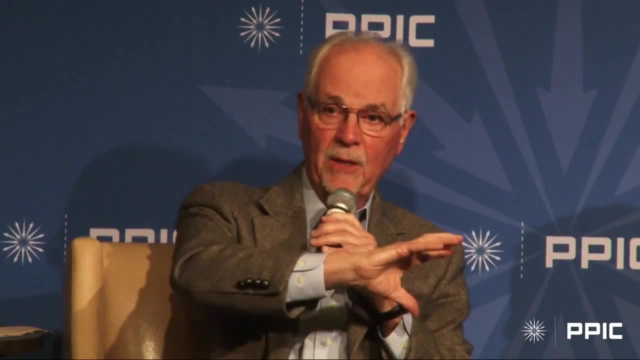 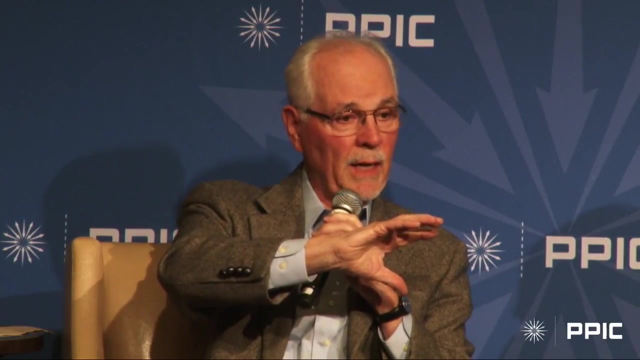 compounded by human impacts on that environment that make it really difficult. That, as much as anything, is why I favor the notion of talking about an ecosystem, although I didn't initially start with that view about 10 years ago- And so I think all of these solutions 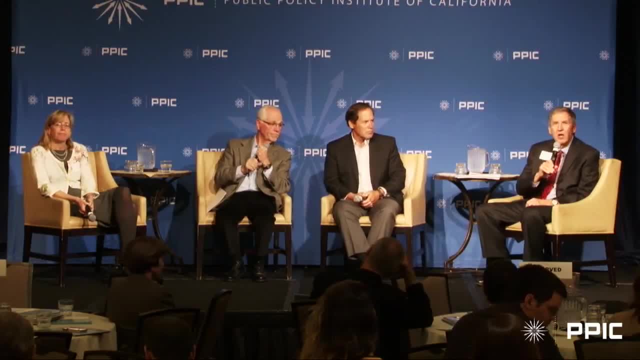 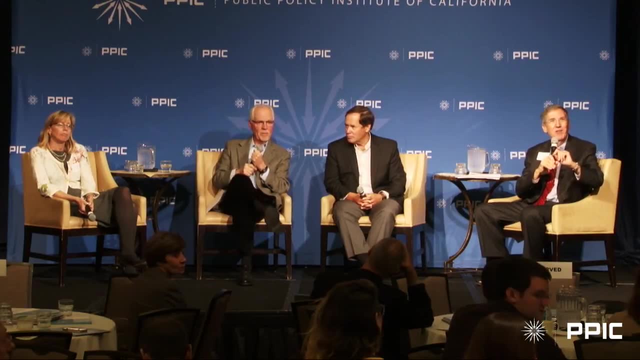 or comments are appropriate. Okay, I think we have time for one and, if we're fast, perhaps two more questions. And there are people going around with a microphone and that's how we determine who gets to ask the question. So right back here. 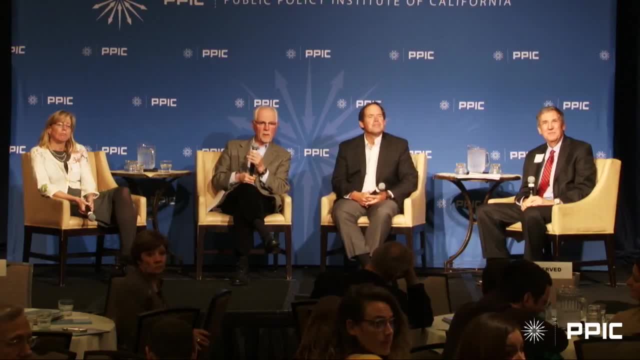 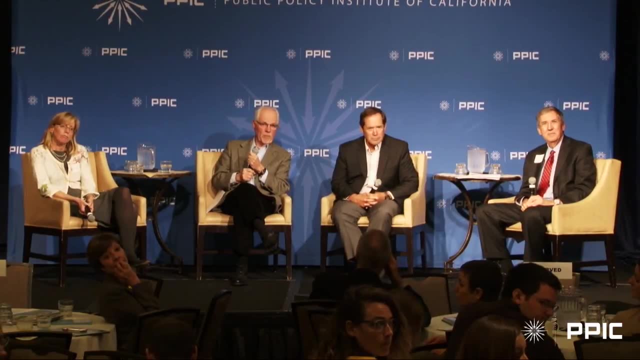 Hi, Ted Grantham, UC Berkeley. You've talked about this transition from sort of a species-centric management approach to an ecosystem management approach And it seems like as part of this ecosystem management vision, it's important to know what you're managing for. 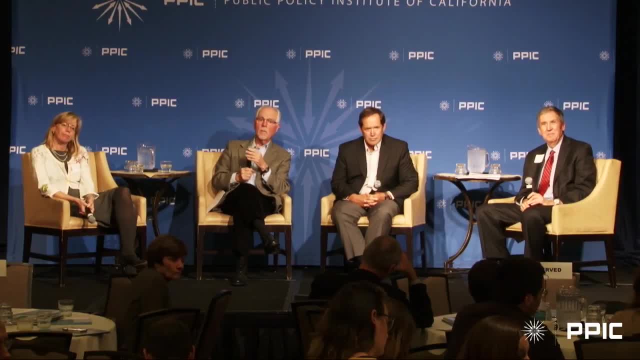 I think one of your comments earlier- Phil suggested that what is our vision for success, And I'm just curious if you could comment on what that process looks like. Is it for science to define sort of what those fundamental ecosystem processes are, or is it much more of a social process? 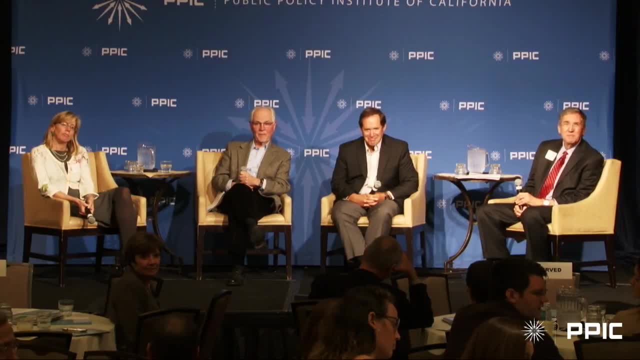 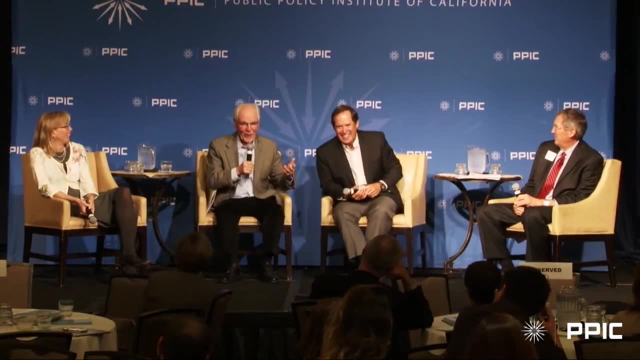 to define what kind of environment we want to live in in sort of a policy context. How would that even work? That's for you Okay? Well, all these science guys wander in and talk to us poor public policy people and they say: 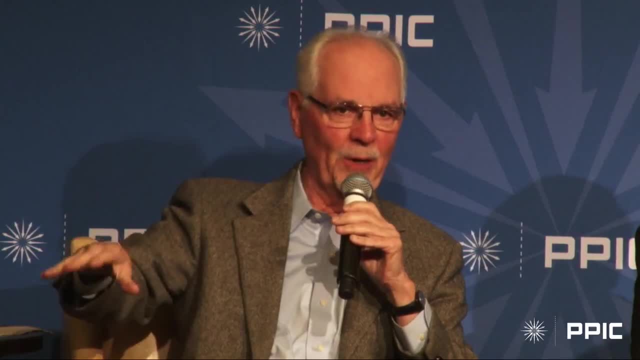 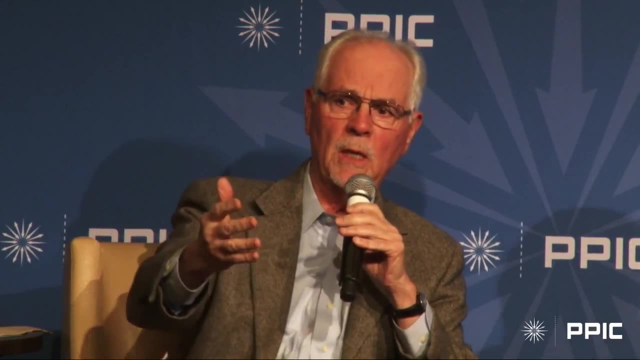 look, here are the problems with what you've said you want to do, And we say, oh God, that's terrible. Tell us what we should do, Not our business. You set the priorities. You set the priorities and we'll tell you when you're wrong. 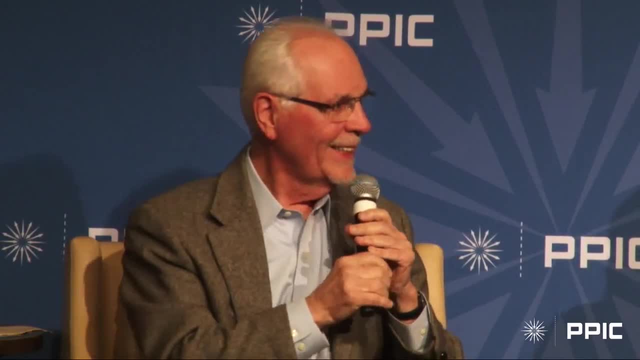 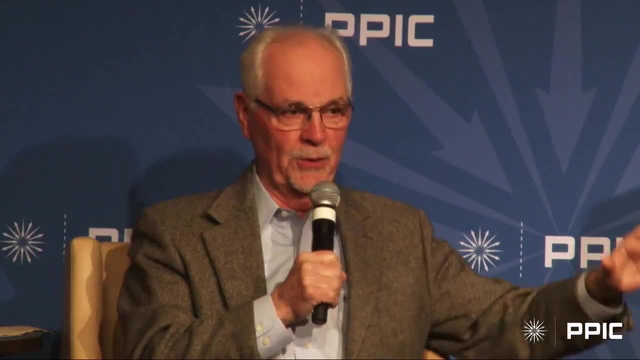 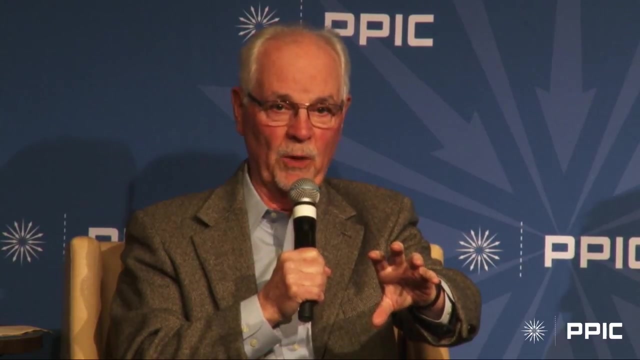 Well, screw that, Who cares about that approach? And so I just think what you got to do to the scientist. That's why, in addition to merging the operators of the Central Valley Project and the state operators of the State Water Project in one building, 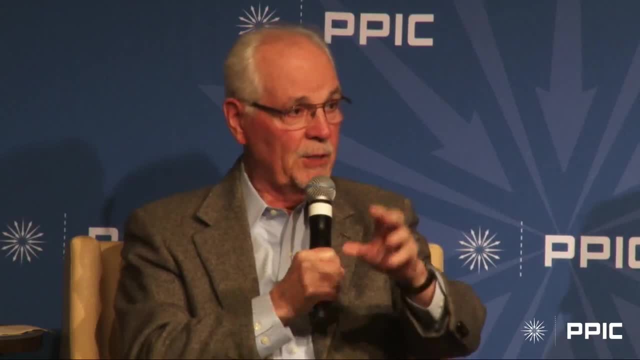 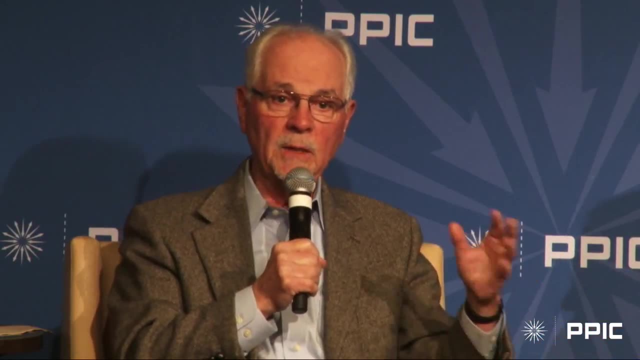 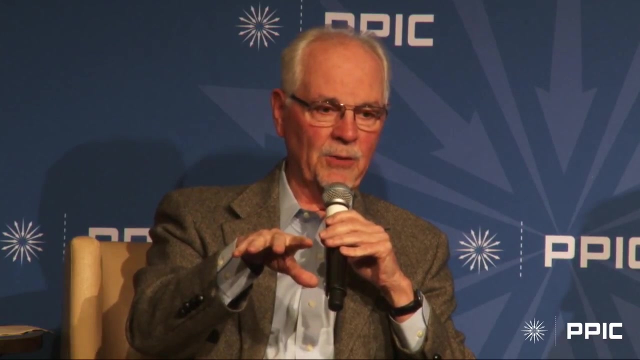 I'd throw these scientists in and say: you get to vote on both water issues and ecosystem issues, so you can't screw up either. Because I can't think of any better way to approach this than to try to figure a mechanical process that takes the policy decisions. 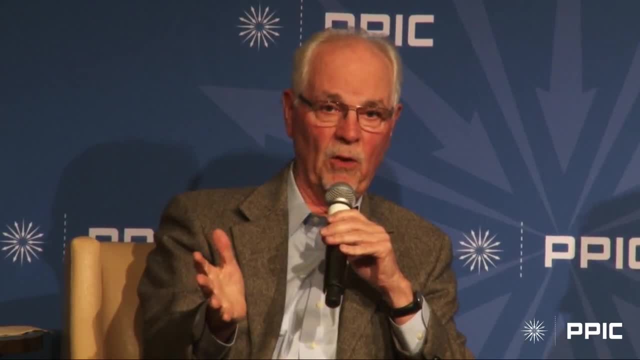 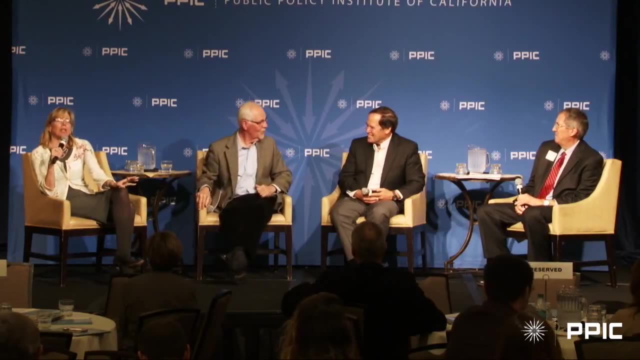 no matter how imperfectly written, that are in state law and tries to implement them. Kate, Just one quick thought on that. I don't agree that we have been so focused on single species approach to our detriment. You know, I think a lot of. when we looked at how do you restore the San Joaquin River. we looked at how do you restore salmon, Because if you restore salmon to that system you bring back a whole host of- you know, the native community. Same for the Bay Delta system. 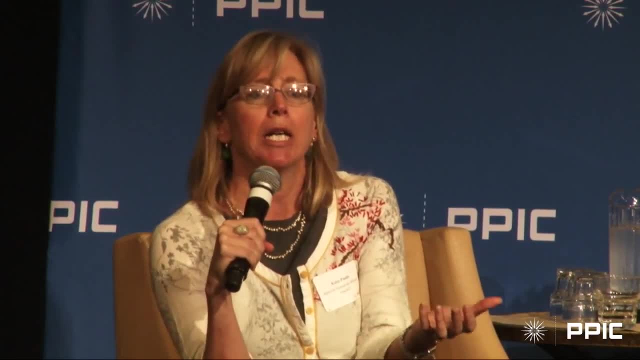 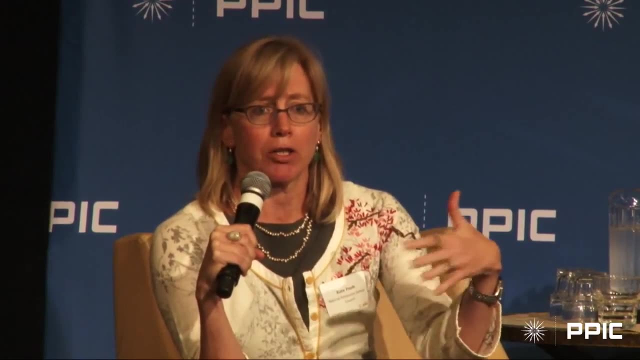 And I think a lot of the focus on the Delta smelt has been because it's an indicator species for the health of that estuary which relies on that freshwater-saltwater interface that the smelt likes to hang out at, and you know how functional that is. 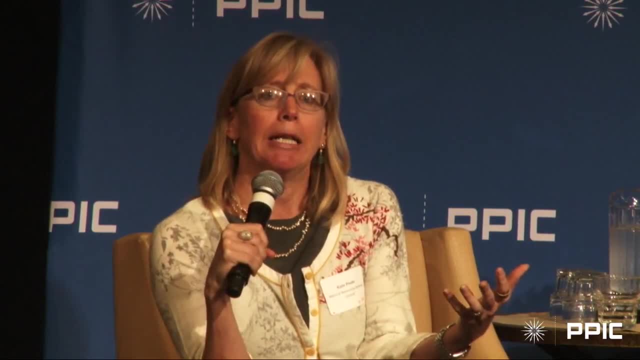 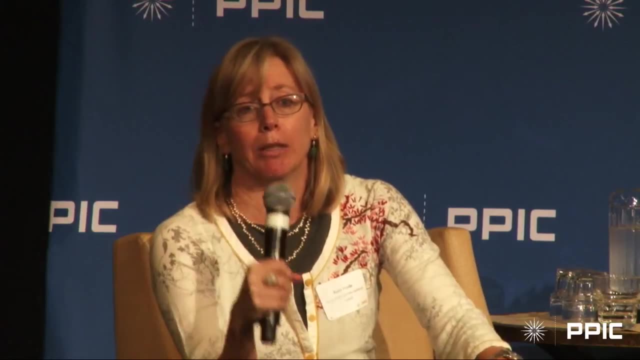 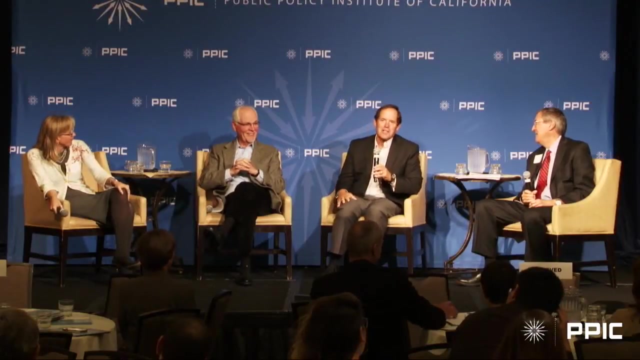 So these are species that really support a whole host of functions and it's not just about those individual species, in my opinion And Jeff, I have been on the receiving end of Phil's abuse over all these years and I've enjoyed it so much. 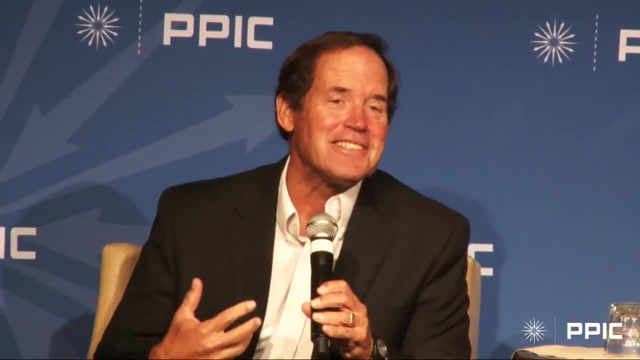 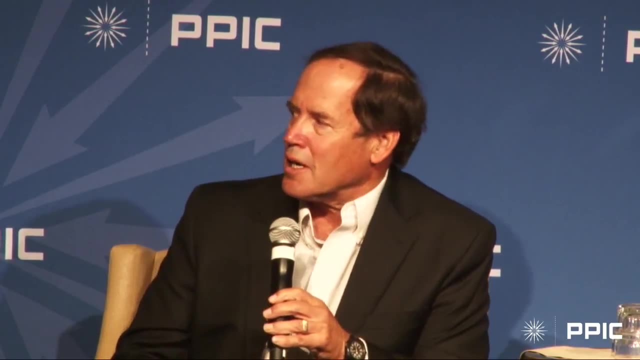 And so it's such a pleasure. And I am guilty of being a weasel. when it comes to this very issue, I'm the first to say: nice idea, that won't work, and that's usually where I stop. So I agree with him. 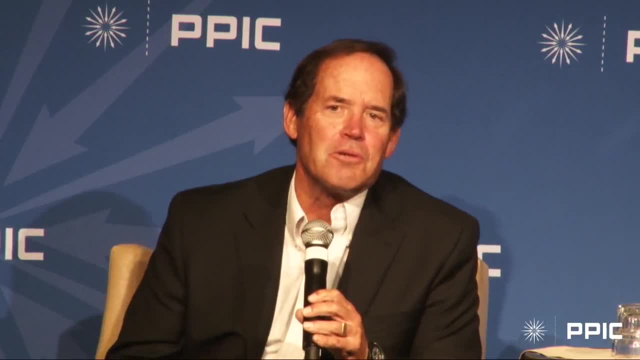 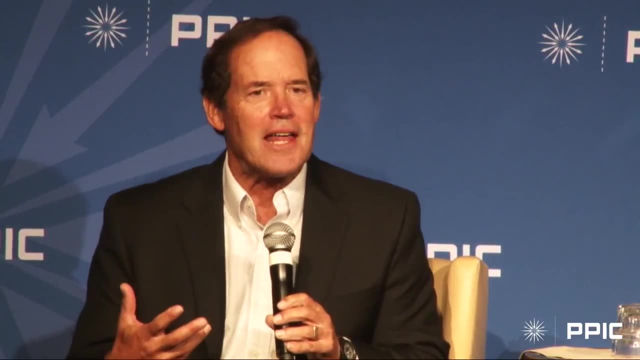 And, Ted, this actually goes right to you And the kinds of work you do is. this is where the scientific community has to science up is the best way I can describe it, And what I mean by that is that we need to engage on the sociological side of this. 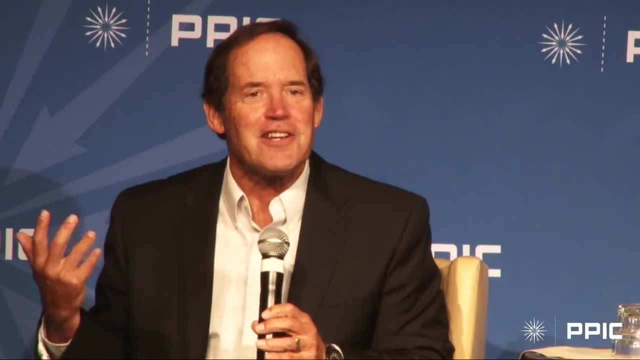 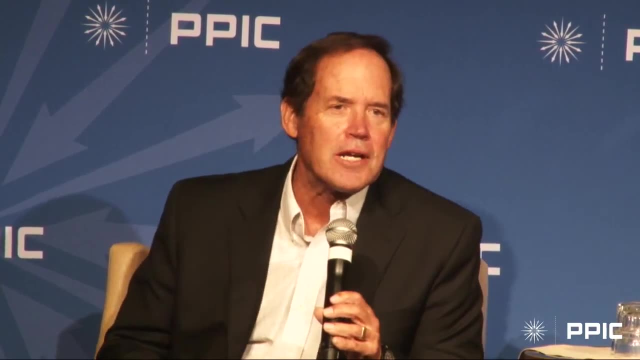 and be honest about it. So yeah, if I got locked in that room with Phil, I would say, Phil, here's what I think you can accomplish. I think you can accomplish a system in the San Joaquin River which has fabulous riparian habitat. 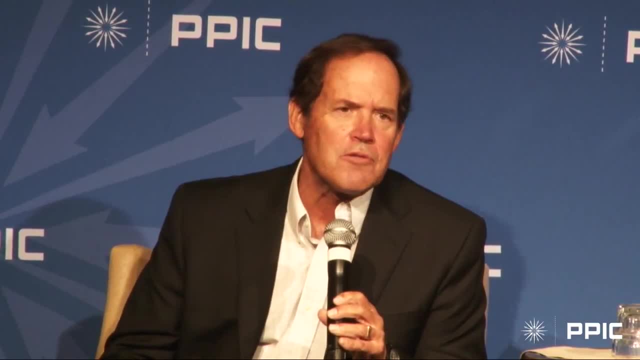 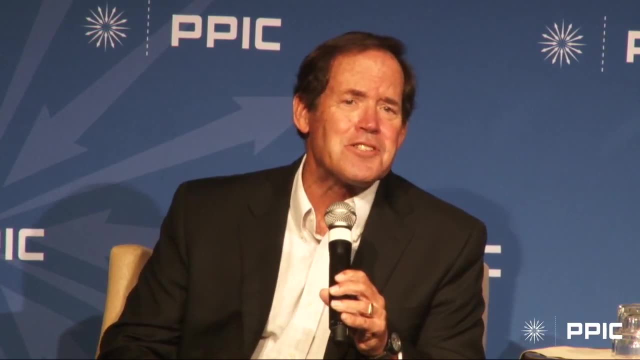 that supports riparian function. I'm a little more dubious. you'll be able over the long term to support salmon, as climate change is in that system. but I can tell you where you can and you can in the Sacramento system and that maybe this is part of that notion. 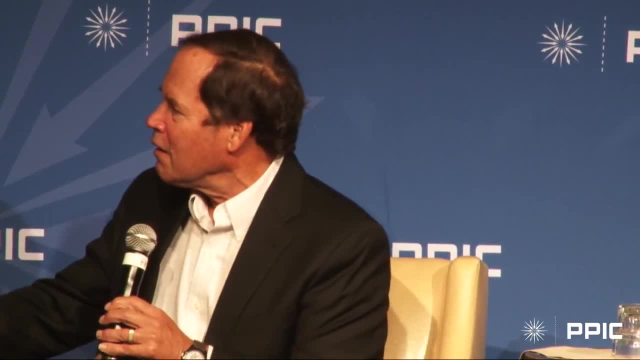 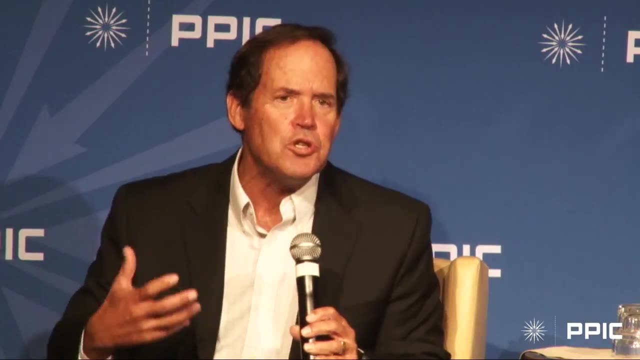 of specialization. I also tell you, Phil, I think you can restore a healthy- and healthy is a movable target delta- that you can have a delta with good estuarine function within it. It may not have the native species you want. 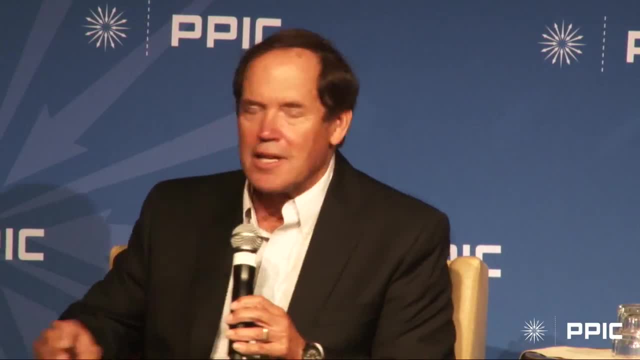 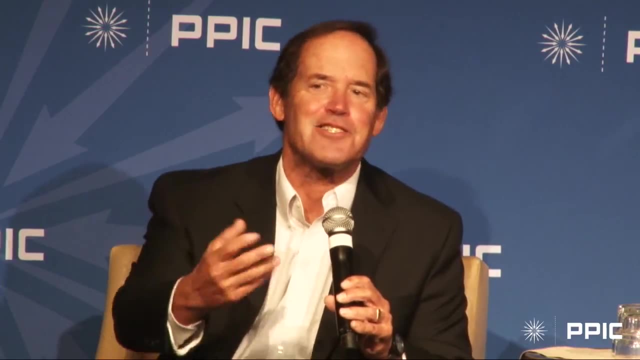 but it can be- this is part of that visioning- it can be a healthy ecosystem, as we as humans decide what that healthy ecosystem is. So I think the scientists- this is where we have to get out of the business that I've been in all this time.